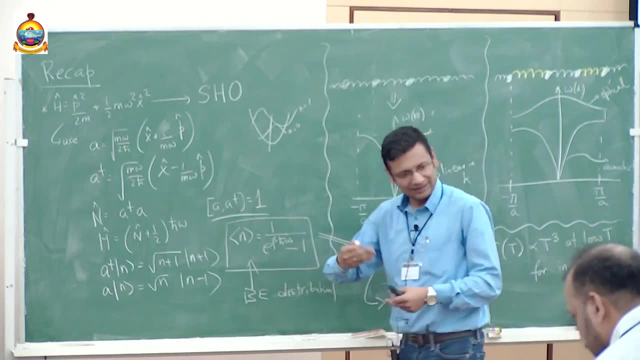 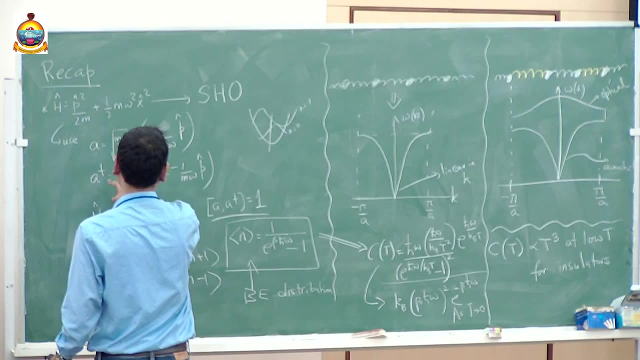 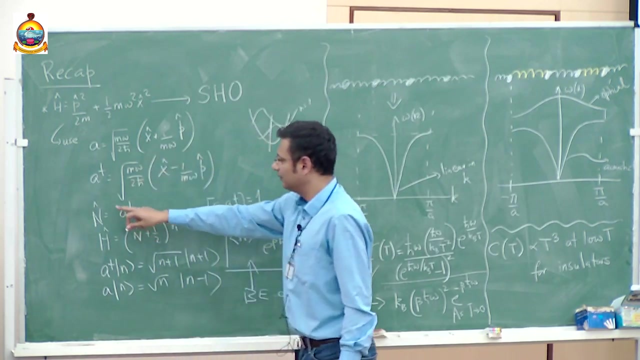 are rare, And so, typically, whenever you see such things, there is a better way of demonstrating the physics of it, And, in fact, in this example, the better way of demonstrating the physics was, as we saw, by using these creation and annihilation operators. right, And then we? 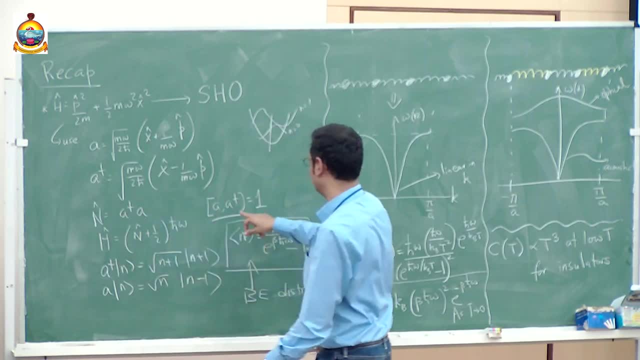 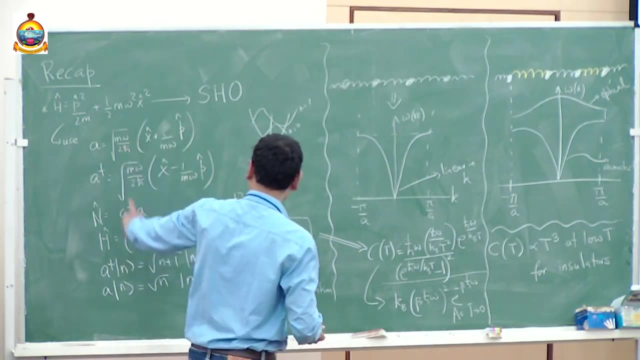 saw that this literally looked like a boson problem and it had the right algebra And we could use this to get basically everything, and this also helped us understand this Right. And then, similarly, we get a, D- Okay, the additional operations in the right hand end. 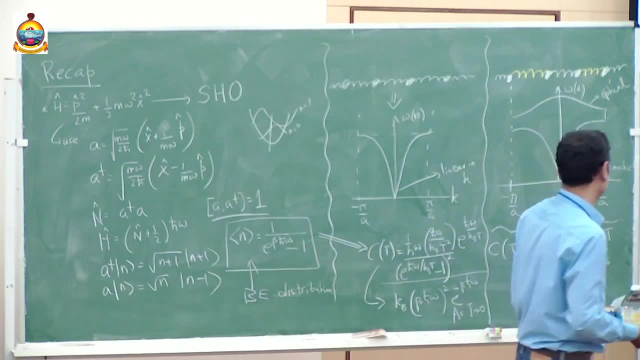 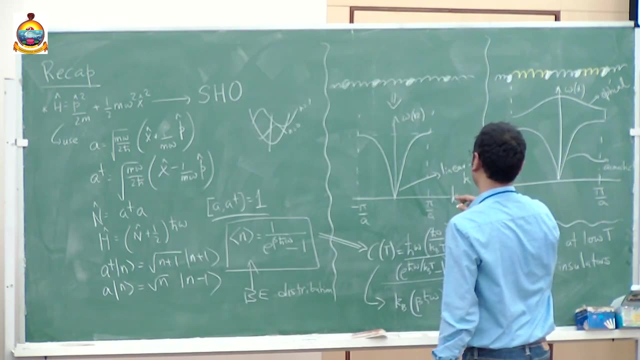 right why there's a Bose Einstein distribution here, right? so that was one thing. the next thing we did, and then we sort of ran out of time, is: take two very simple problems and sort of understand the quote-unquote normal modes of that. so basically, if you take problems, 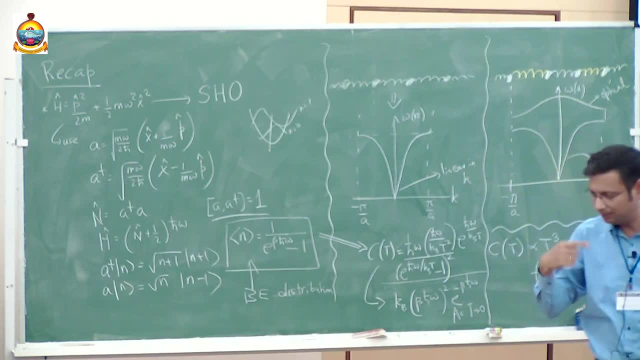 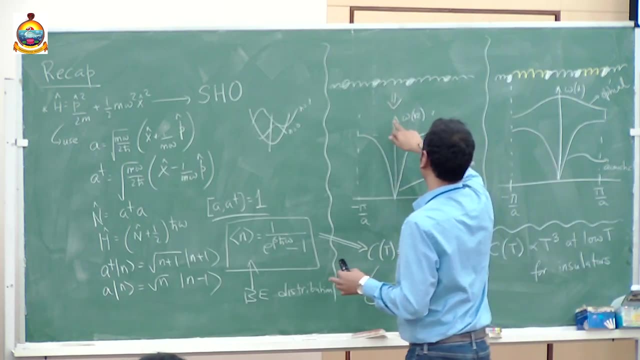 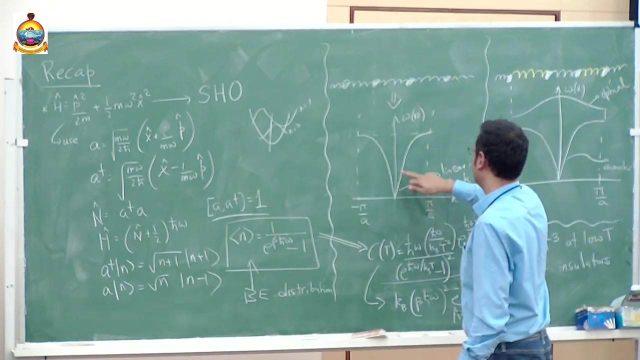 where the Hamiltonian is quadratic in both X and in P. then there exists coordinates in position and momenta, which are known as normal modes, where the problem becomes just a bunch of non-interacting harmonic oscillators, each with different frequencies, and for problems where there is translation symmetry, you can label each of those oscillator by its own. 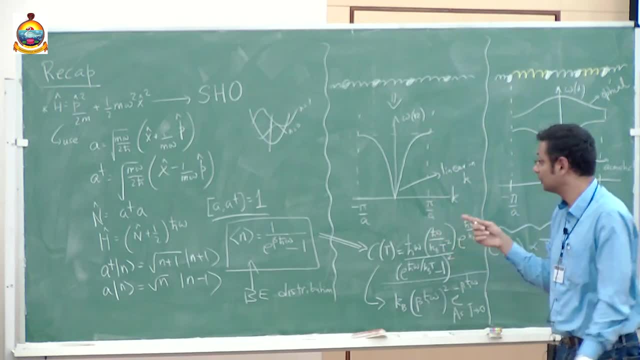 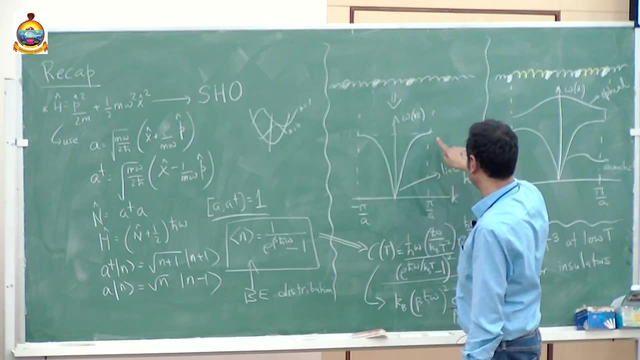 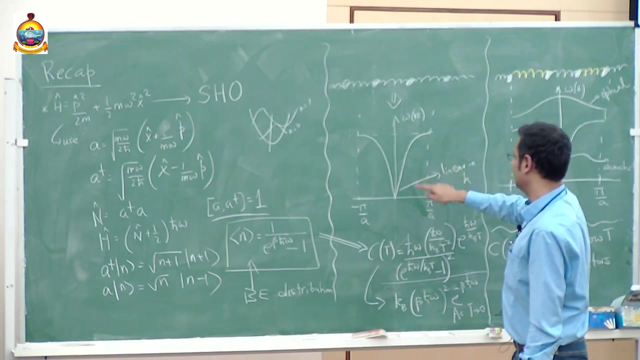 momentum. okay, because momentum is a good quantum number in those cases. so then, for the very simple case Where there are these, for example, particles connected by springs, we could obtain this dispersion for the normal modes as a function of K. and then, of course, we highlighted the 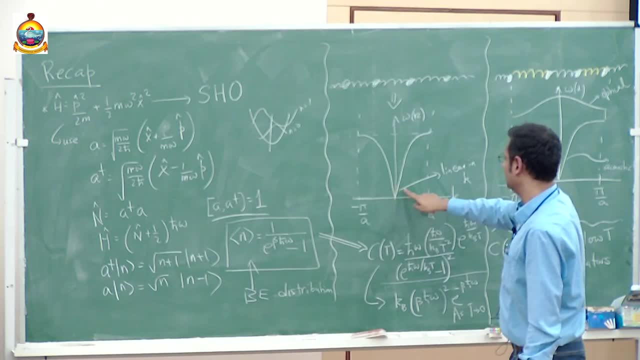 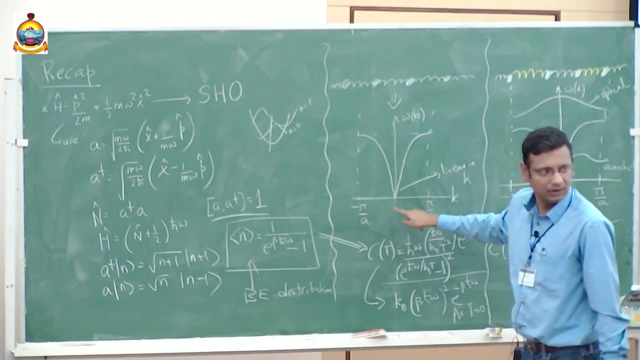 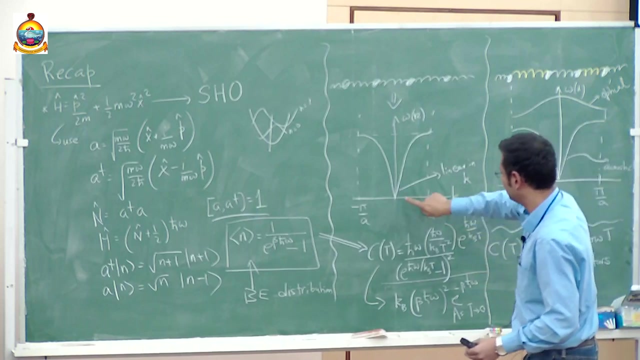 fact that a very interesting thing happens here- that there are normal modes whose frequency basically goes to 0, near K equal to 0. so the bottom line is that there are gapless excitations in this system, right? Because it creates a very small amount of energy to create an excitation near K equal. 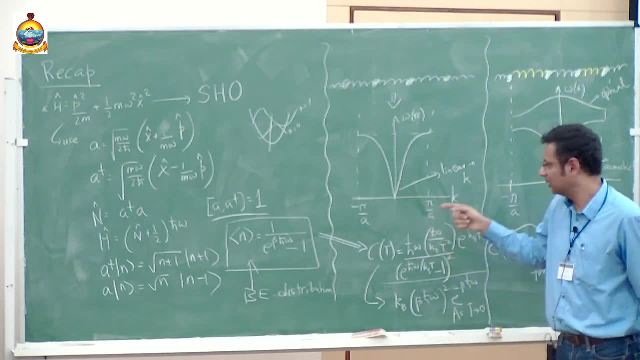 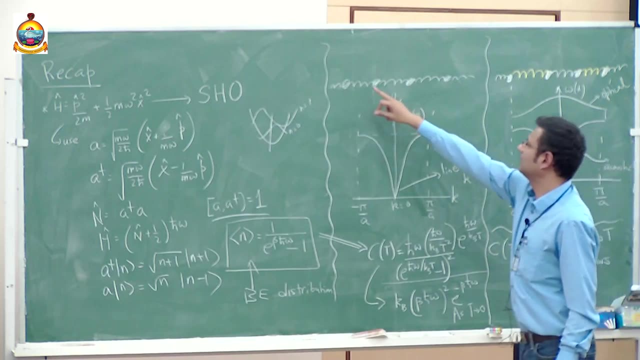 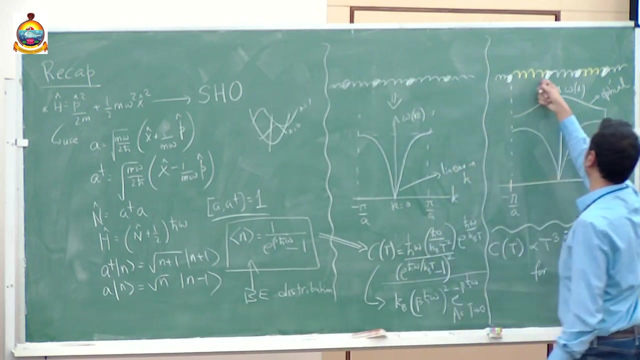 to 0 right, and that gap can be reduced to be as small as you want as you move to K equal to 0 right. good, okay. then we said: okay, let's take a slightly more complicated lattice. so we took that, where instead of one kind of springs we had two kinds of springs, if you 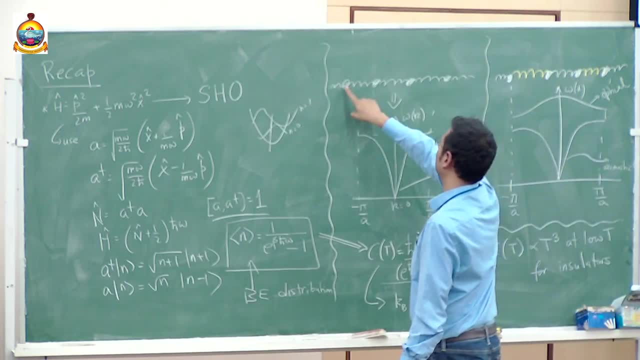 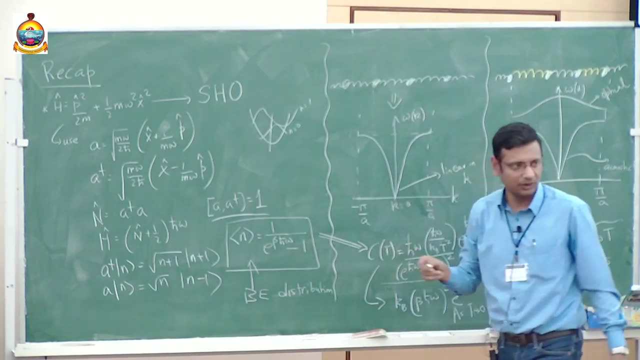 wish, or if you want to think of an alternate situation. maybe, instead of maybe, you can keep the springs to be identical but say that there is mass M1 here, mass M2 here, M1, M2, and so on. that also you can do, right? so then we realized that here the dispersion was slightly more. 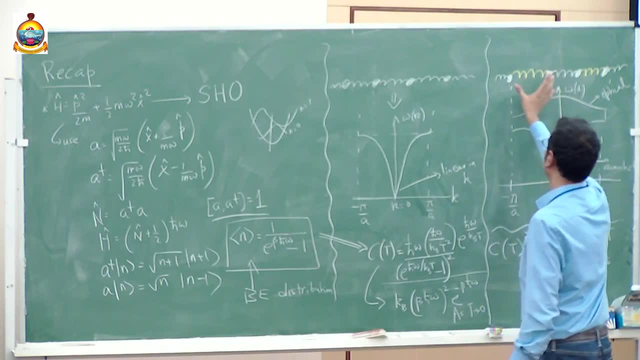 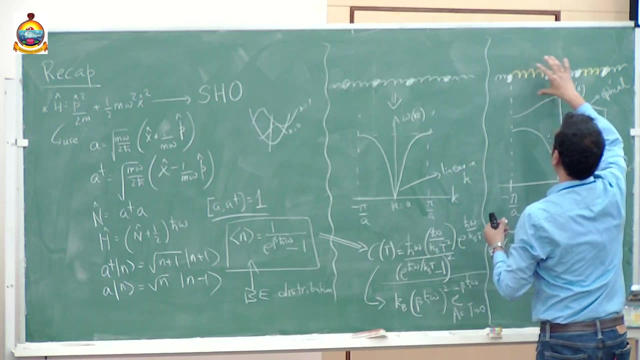 complicated. it had two branches, of course. the reason it has two branches is clear, because when you sort of write it in momentum space, you have to use a two point unit cell and that unit cell is repeated, and that's why you get two branches. If you took a 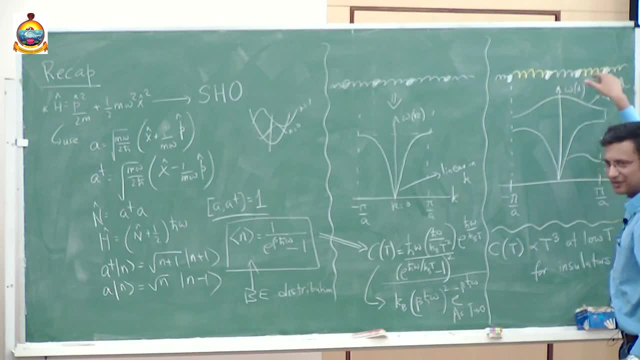 Problem where maybe I don't have two colors but three colors of springs and I keep repeating them. then I would have three branches and so on and so forth, right? So of course in a real crystal there are the unit cell. may be very complicated things like: 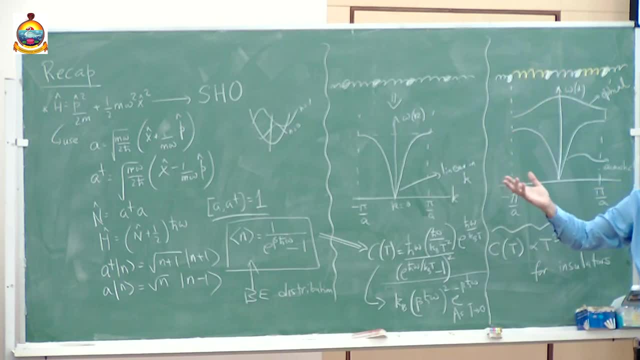 that. and then, of course, in a real crystal, you would expect many branches, right, But the important thing here is that again, there was a branch which actually became gapless. So When the momentum became close to zero, right, exactly like this problem. of course, there 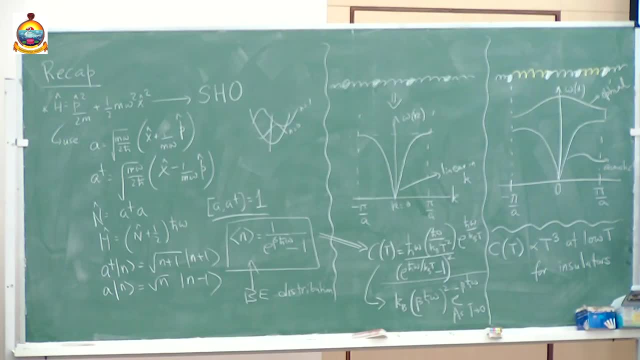 is also a branch which is always capped right, and we discussed why this is called acoustic, why this is called optical, so on and so forth. right, yeah, that's exactly what I just now said. yeah, like two sentences back, I said that. right, please pay attention, Thank you. 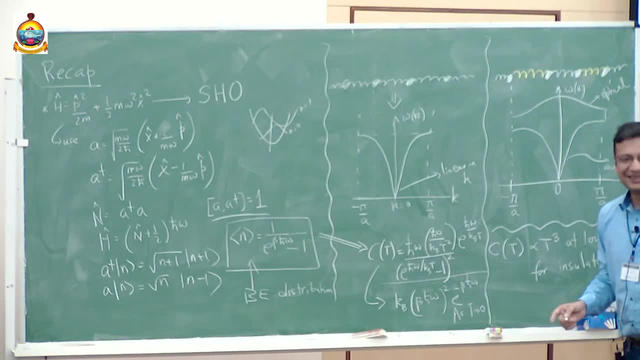 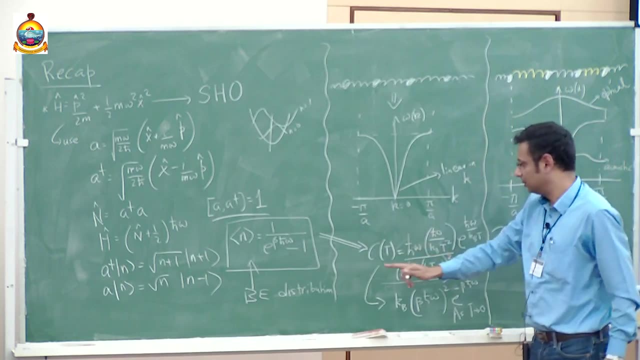 Thank you. Thank you. Now. In the harmonic oscillator problem we also calculated the specific heat, right, if you remember, and that was a very easy calculation and we got some complicated form. But this complicated form gave us two simple limits. at high temperature we got K B out. 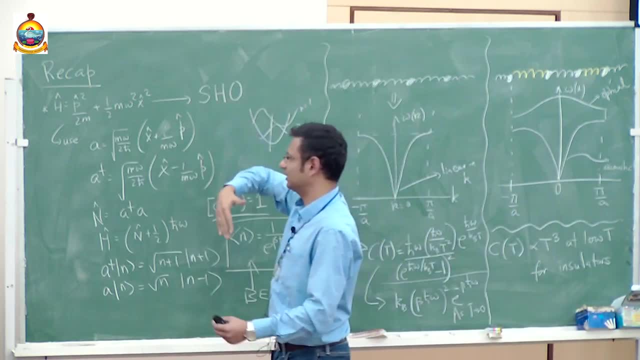 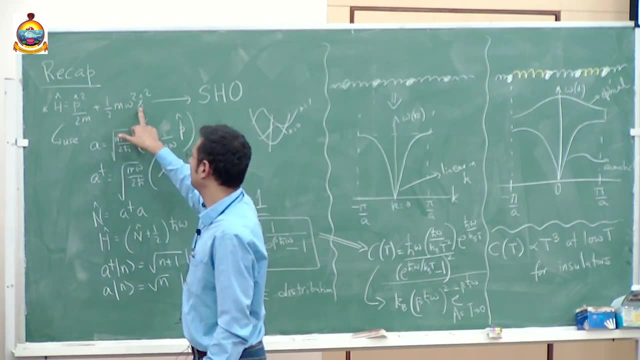 of this, and that's of course correct, because in the classical limit, which is what we recover when we go to high temperature, Ah is quadratic and this is quadratic and you know that there is something called equipartition theorem. so you will get half Kb from here and half Kb from here, so you add them up and 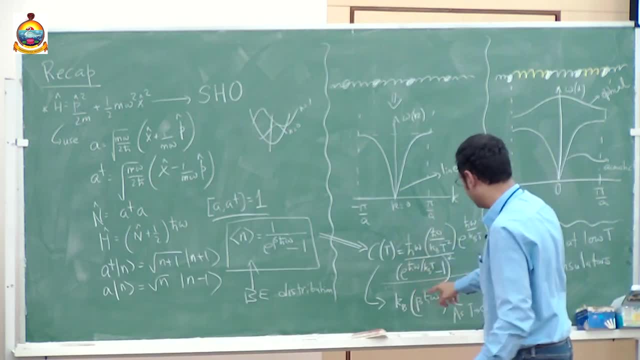 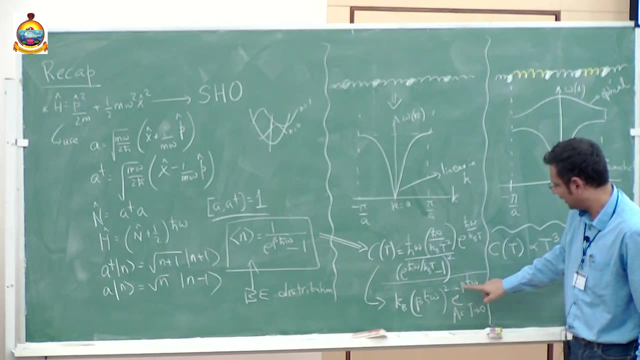 you will get Kb for the specific heat at high temperature. good, at low temperature. we got the following relation, which the important thing is: there is an exponential in temperature, right? so minus h cut omega divided by KBT, right so the specific heat is exponentially low at low temperature, and we in fact said that this is a general property of systems. 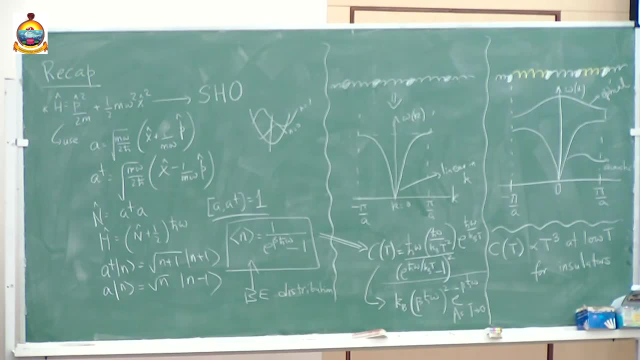 which have gaps from the ground state energy. ok so, and in fact, if you look at the low temperature, specific heat, in principle you can extract the gap from there. good. however, there is a very well known experimental fact that for insulators, for insulators, the specific heat. 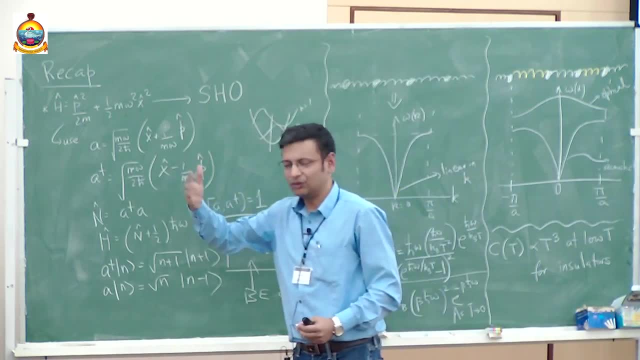 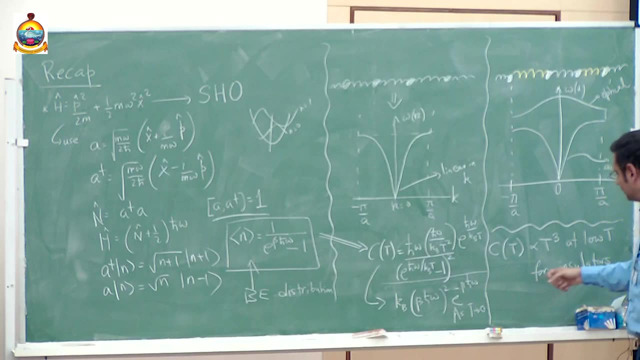 is not n times Kb, which you would have naively expected from equipartition theorem. in fact, it decreases to zero as temperature goes to zero and it decreases in this particular way. Tq ok, and that is sort of a universal fact. it is true for most insulators that we see. 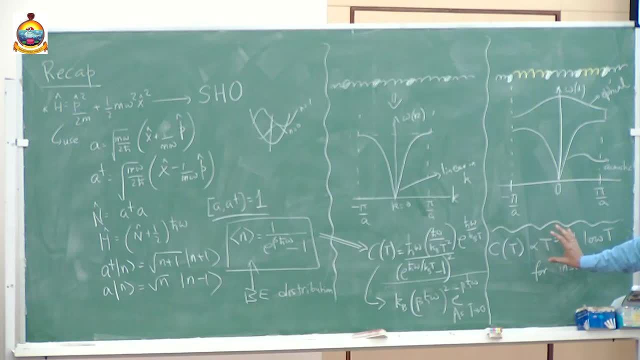 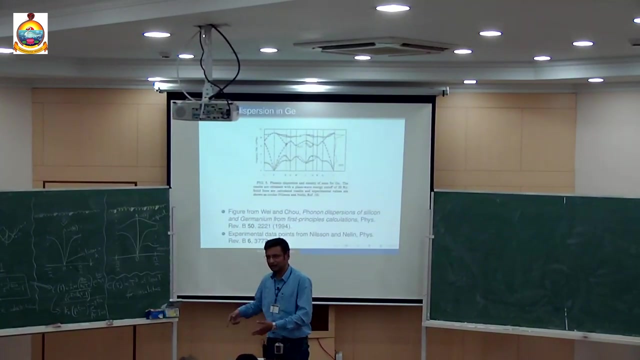 around us. ok, so then we plan to understand this statement today, right? so that is essentially the recap of yesterday's class. ok, so before I start discussing things, if you have any questions, you can please ask. well, we haven't seen it yet. we'll show it in today's class. right, we'll show it in today's. 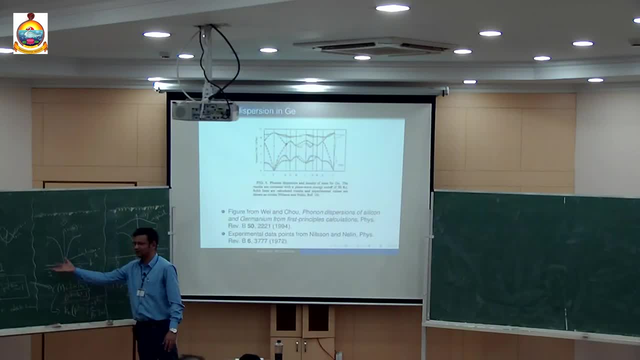 class. so right now we haven't seen it, we have just calculated this. but this is for a single harmonic oscillator. now we'll see what happens if you have a bunch of harmonic oscillators with omega k like this and each of it is an independent boson problem. and we'll sum up 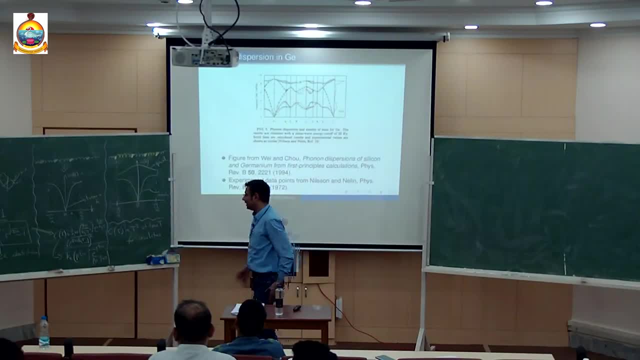 their energies and then from that we can get specific heat right. and the reason, see, this is important to understand is because, in this particular case, the information that I was asking you about has been given by everything, but the next step you will just take and add to appreciate the reason you don't get an exponentially small specific heat should be: 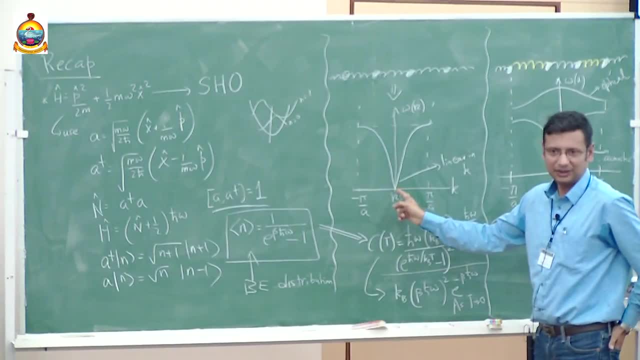 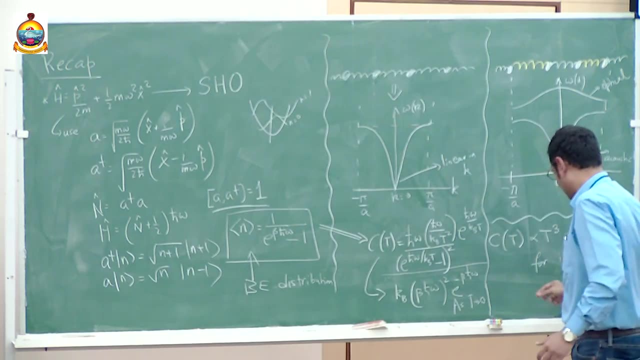 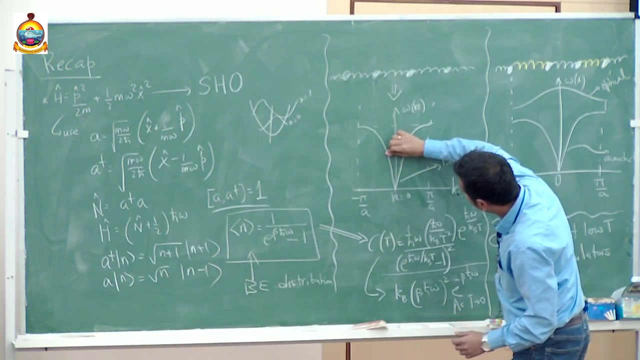 clear to you is because the gap is going to zero here. see, this is the thing to stress, right? suppose i gave you a dispersion curve which basically- okay, maybe i use some other color. uh, let's say, i gave you a dispersion curve which did not look like this, but look. 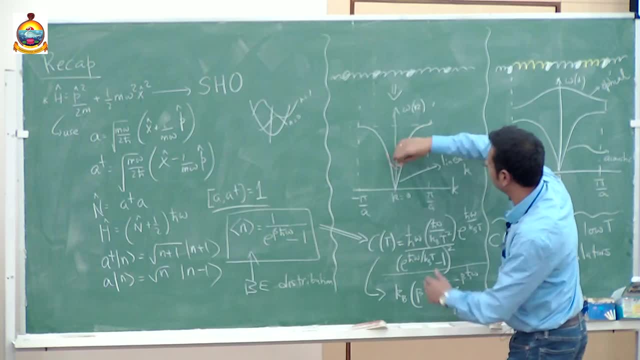 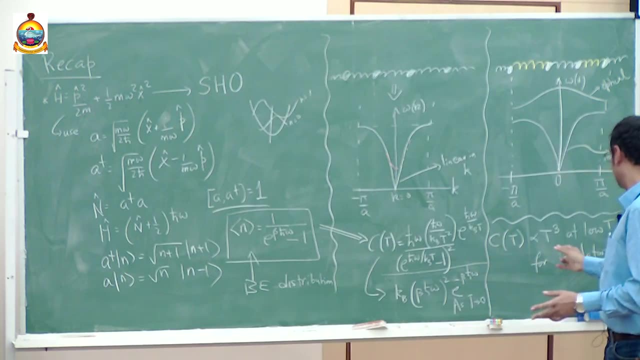 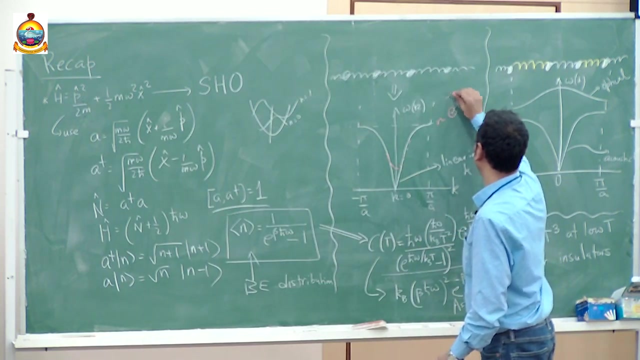 like that right and this same curve right, but it sort of goes like this right. then, even without doing any calculation, i can tell you that the specific heat won't be t cube, it'll be just, let's say, this gap is delta. it'll just, at low temperature, be e to the minus. 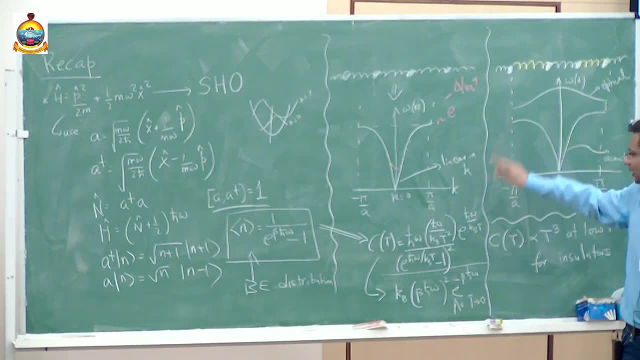 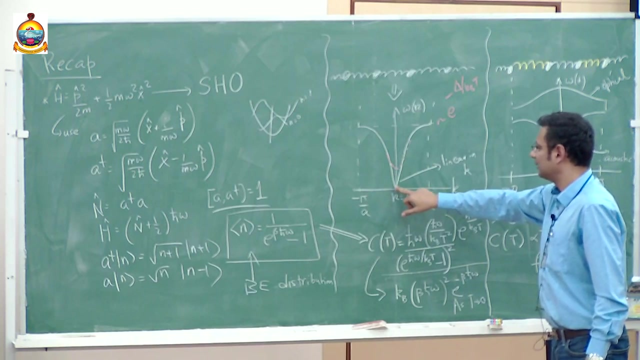 delta by kbt. that's it. okay, it can never be of this form, right? okay, good, uh, but we learned at least from these two calculations that that is not the case and, in fact, what i told you, without giving any proof, is that, uh for a crystal, there will always be some gapless. 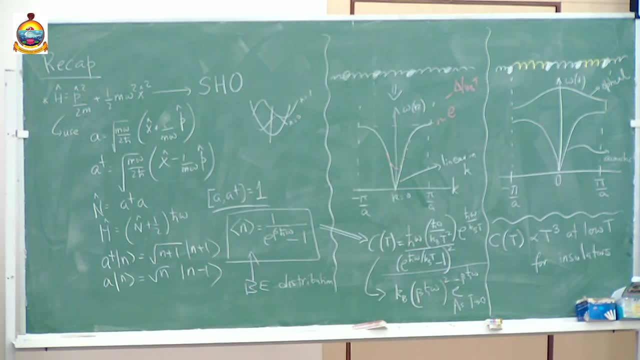 excitations, because you can see that the heat is not going to be t cube, and the heat is not going to be t because a crystal spontaneously breaks a symmetry when it forms and that's a continuous symmetry of translation. and whenever you break a continuous symmetry, uh, you get these. 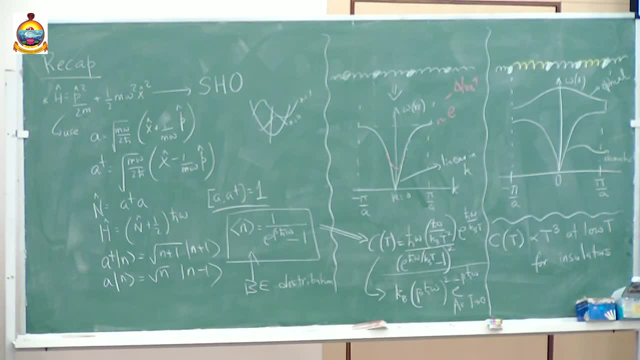 gapless modes which are called goldstone modes. i did not prove it, i just stated it. but this is a general uh thing for these kinds of continuous symmetry, breaking any other question. oh so goldstone modes. goldstone because among other people there were many people who sort of proved: 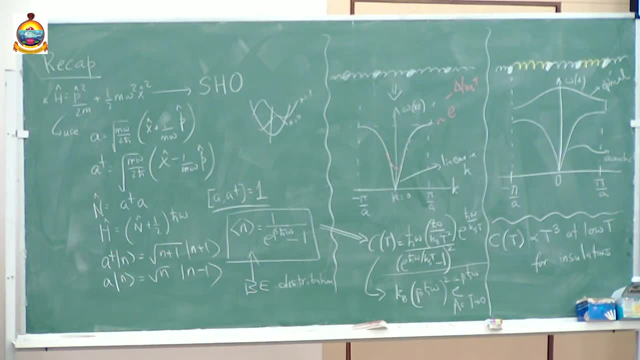 this roughly at the same time that if you have continuous symmetry breaking, you get these kinds of gapless excitations. but somehow the name of goldstone got associated with it. that's always the case in science. many people somehow: okay, this is an accident. but okay, yeah, goldstone. 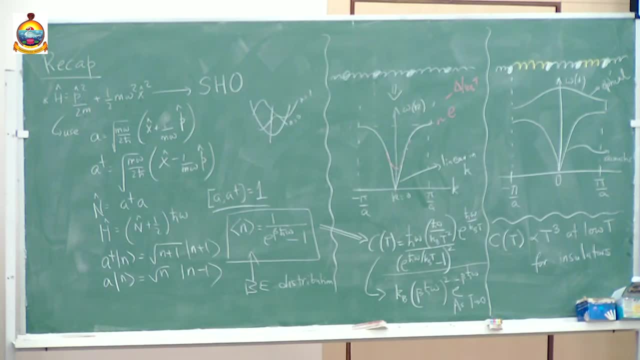 was one of them, but there were many other people. yeah, then it's quadratic, then it's k square. yeah, instead of k square, then it's k square. yeah, correct, that's also important. yes, that's also important. so, as pk said, suppose this harmonic thing is not there, then it's just a free particle dispersion. you know what it is, it's k square. 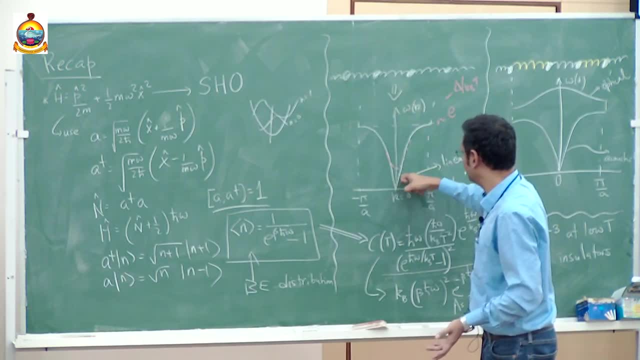 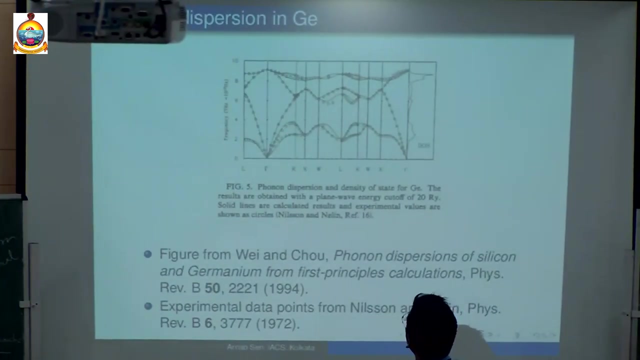 but because, because of these uh, the dispersion changes from k square to k. that's another important thing to keep in mind. okay, good, any other question? okay, good, so now let me show you a complicated curve. this is actually a, actually the phonon dispersion of a real element. this is actually germanium. okay, and i have 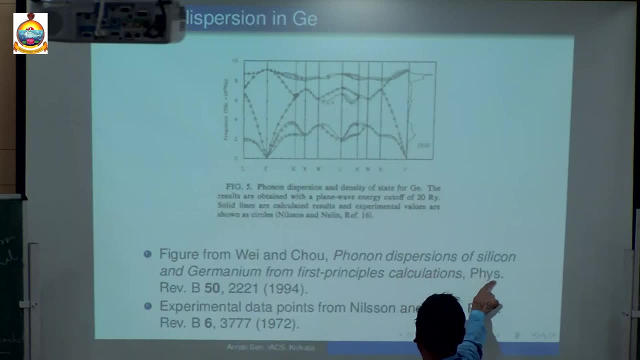 taken this figure from this particular paper. here is the reference. so in case somebody does not believe me, somebody can open this paper and see right and basically this paper. these two authors were trying to explain, from some first principle calculation, the experimental results of these two authors. okay, 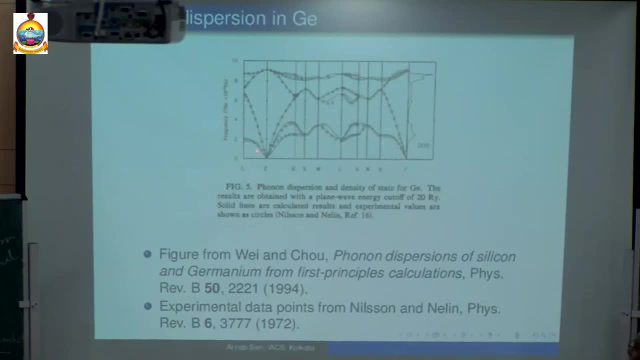 so this experiment was in 1972, where through some neutron scattering techniques they obtain these dots. so using some experimental technique they could actually obtain in germanium what is the phonon dispersion curve? okay, and these are these dots. these dots and these lines are from this theory. now please notice one thing: as we just now discussed- i mean of course, 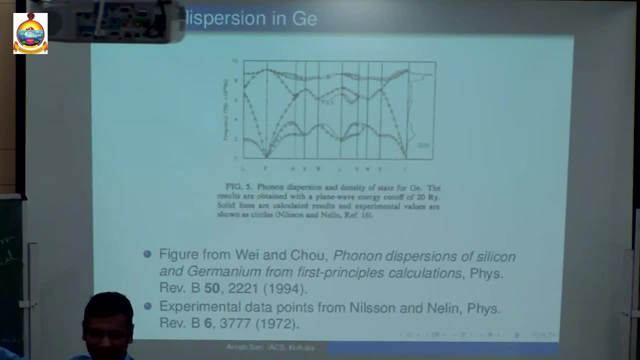 in a real crystal with a very complicated unit cell, you can have many branches, right, that's now what i just said. you can have many branches, right, that's now what i just said. so of course, in this thing there are many branches. but please notice something which 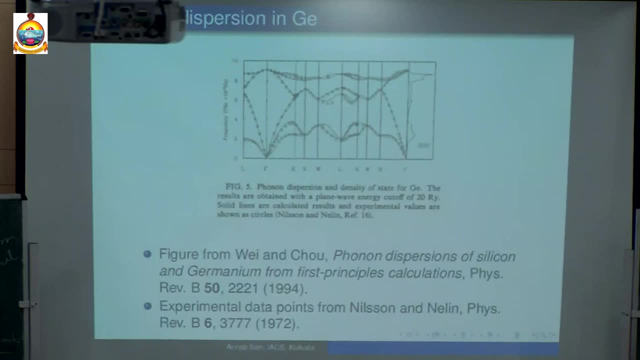 we discussed right now. whatever the complicated thing is, there are these linearly dispersing modes which are gap-less. so everybody can see those linearly dispersing modes here, right, they are here and they are here, right. and you can also see the analog of these optical 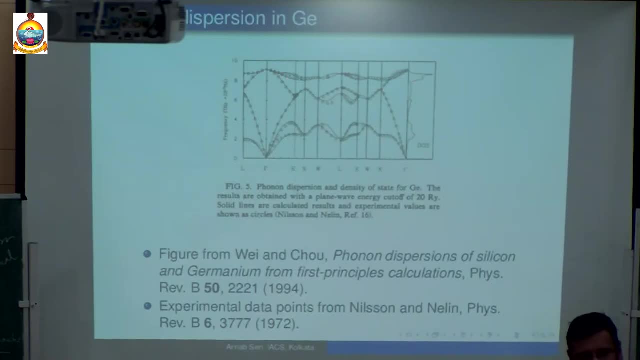 branches. so they are these guys, for example. right, good, so yeah, okay, now let me show you so for any complicated insulator which forms a regular crystal. this is always true. okay, and then we'll construct an effective, simple theory which just takes into account the fact that 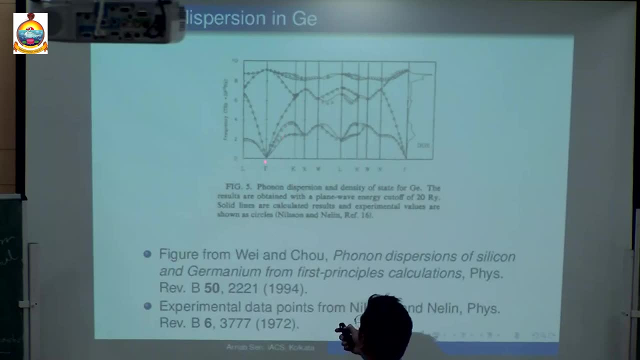 there are these linear dispersing modes. see, suppose your temperature. you're looking at a low temperature property, you're looking at the specific heated low temperature. then you see, it's enough to just take this structure into account. you don't need to worry about all this complicated. 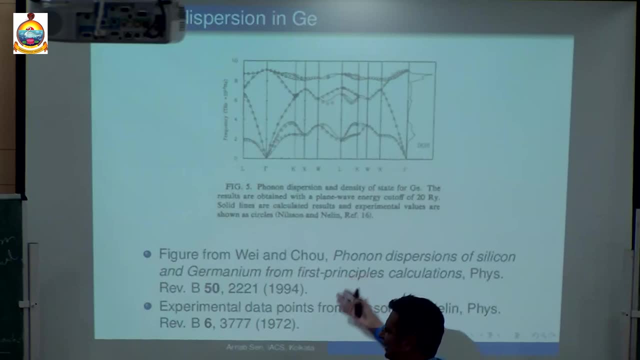 structure, high energy- right, and then you can just construct the theory which takes this into account correctly and you will get this answer correctly. you will get this t-cube dependence correctly. that's what we'll see. of course, this coefficient in front may slightly change because you have all this high-energy stuff here, but that's it. see, I'm using low energy. 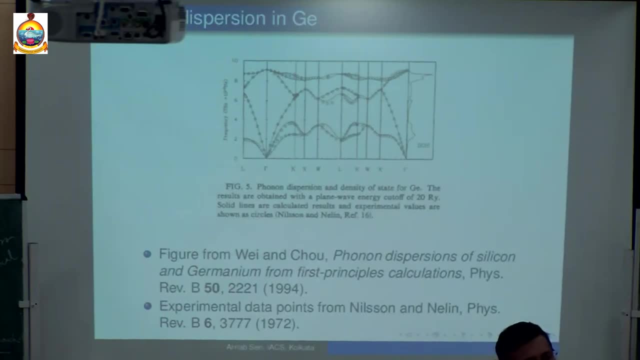 high energy in the sense of the temperature sets a scale here, right? if your temperature is T, then of course, if you're looking at an energy e which is much, much greater than kBT, that's like high energy, right? because there's a very small probability of making. there's a very small 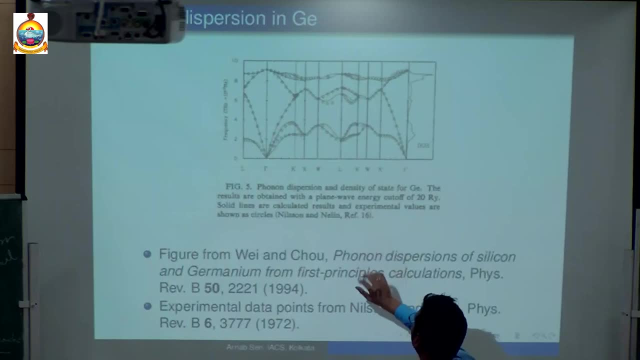 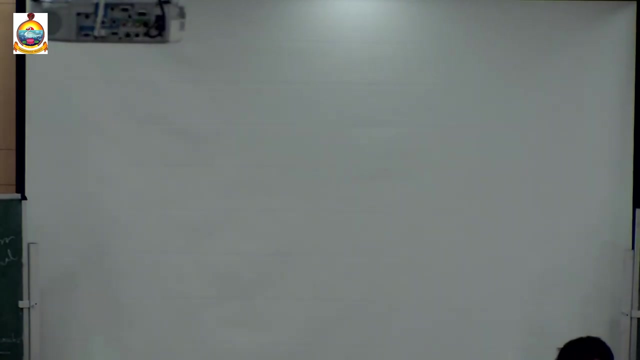 probability of occurrences of those states, right? so yeah, so the important thing is, if you are at low temperature, then what is important is this lower part of this figure, right? and then if you know that it is very low, its lower part of the figure, then what is important is that it is. 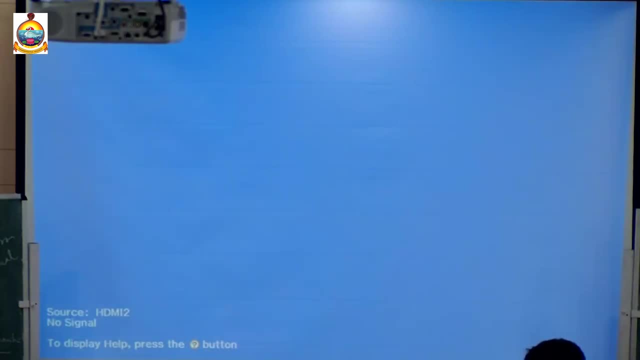 not just something which is very low temperature, but something which is very low temperature, right? so it's very, very simple, right? so that's another very useful thing to remember about condensed matter, right? I mean, when you're trying to understand a phenomenon, you should ask yourself what is important and what is unimportant, and you should try to throw out the unimportant stuff. 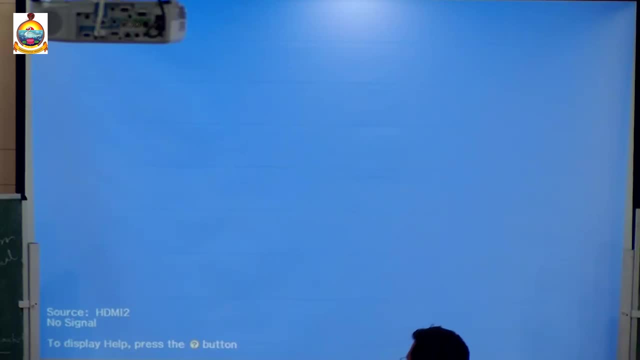 because if you keep everything into something, normally it's impossible to solve it. I mean, that's a fact of mathematics, nature, life, everything right. so, yeah, oh, I did something, maybe didn't like. maybe I did right, so let's do it again, right? so if you, if you take a long temperature, current, a certain temperature, it's going to be. 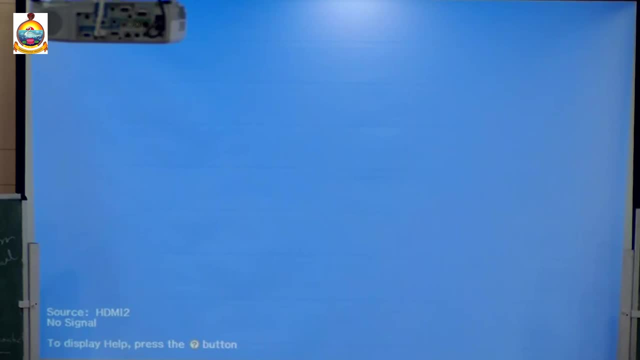 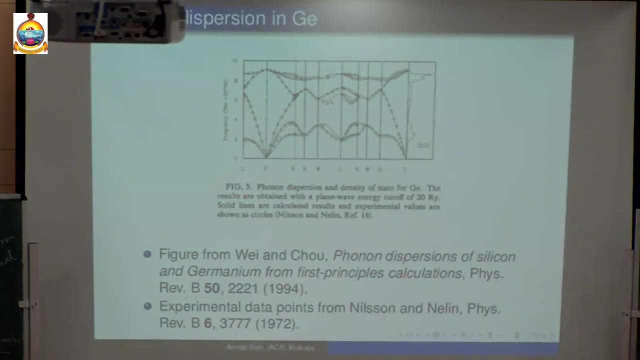 I'm not sure if I have the right number. I'm sure you did not carry around anything by that matter, so Anyway, but that is okay. oh, press the button, would that? oh, thanks, okay, good, So this is what we will try to understand, but I will also give a small prelude to what 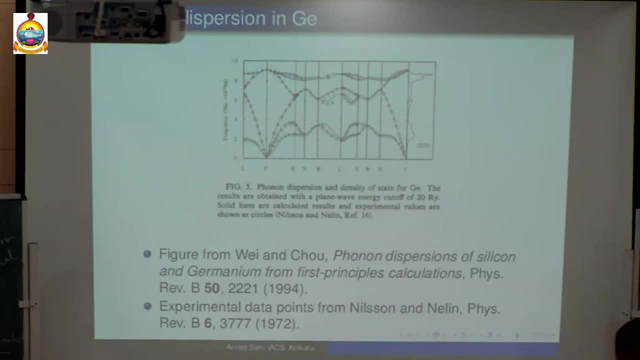 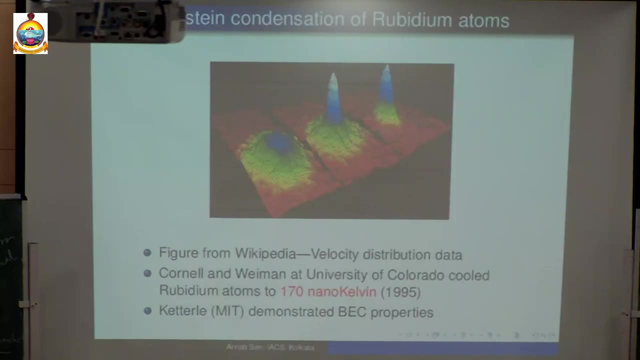 another phenomenon we are going to understand. So this is one phenomenon we will understand in this lecture, hopefully, or part of the next lecture. but another phenomenon which we will also understand is this other thing of Boh Einstein: condensation. This is some picture which probably everyone has seen. I think right, because somehow 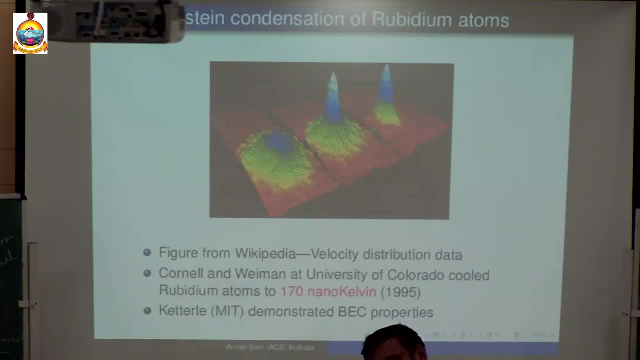 I remember there was a time when I used to go to any seminar, whatever the speaker was talking about, the speaker would show this picture. So there was a time like that, But anyway. so this is basically a picture, so this is a remarkable experiment. 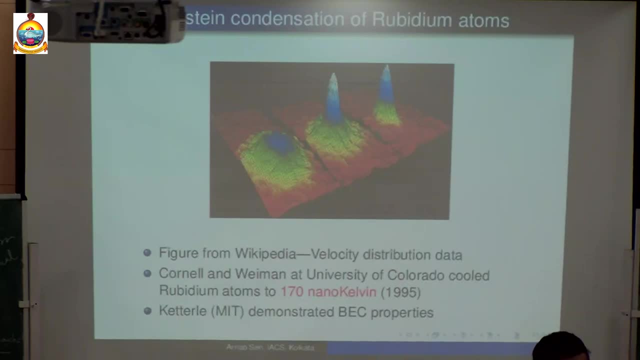 So what happens is that there is something called laser cooling, And using laser cooling you can go to fantastically low temperature for quantum gases. And then Cornell and Wyman first, could achieve this incredible feat of cooling a bunch of rubidium atoms- to please note the temperature: 170 nano Kelvin. 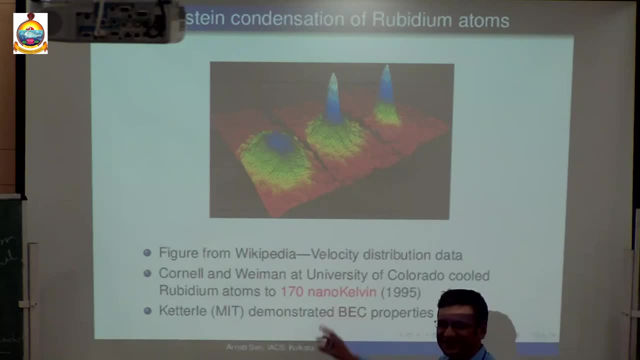 So that is incredibly small, right, I should have maybe not used the color red, but it is incredibly cold, right. So right, Okay, Good, And then soon Ketterly. and collaborators also could see that this condensate at this very 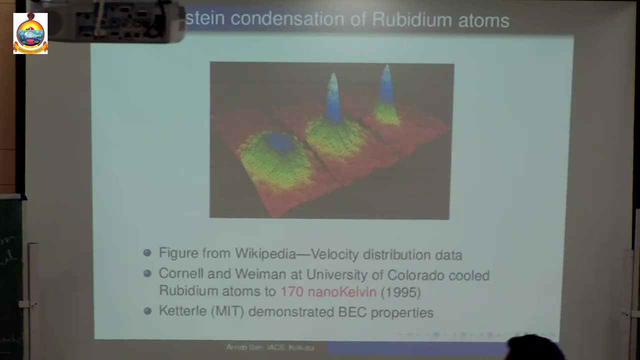 low temperature was really a Boh-Einstein condensate. So what is the meaning of that? So those graphs sort of show you the velocity distribution in momentum space. Now you remember from your coursework that suppose I have a classical ideal gas. then the velocity distribution follows a Maxwell-Boltzmann distribution. 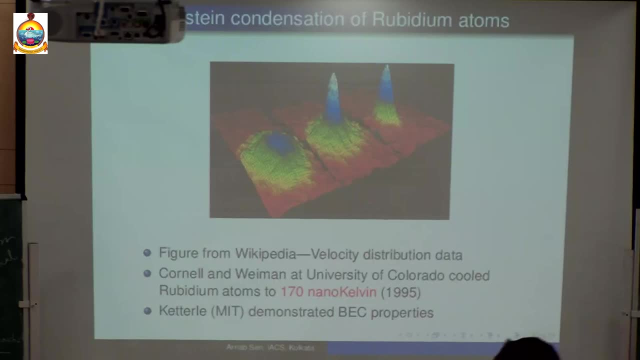 Which looks Gaussian, right And see, you can see that this guy, this guy looks more or less Gaussian. So this guy on the left is basically what the velocity distribution looks like before this bunch of rubidium atoms have condensed into a Boh-Einstein condensate. 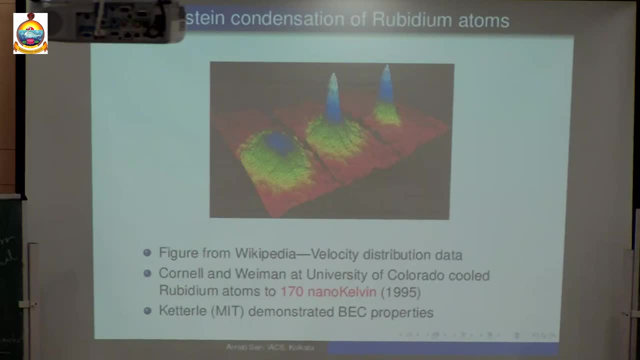 Because here the temperature is the tuning parameter. You have to go below a certain temperature so that this happens. Above this temperature you would not get a condensation. Now you have to go below a certain temperature so that this happens Now. we will in fact calculate this temperature in one of our lectures also, and you will see. 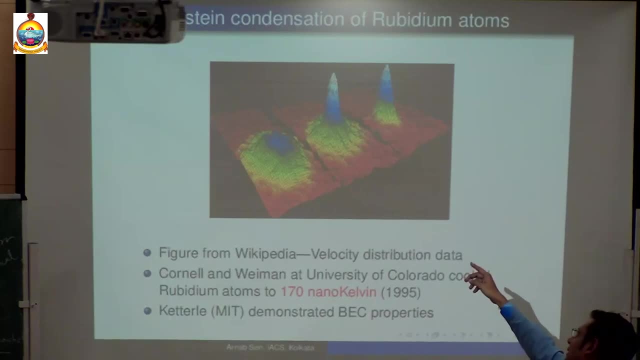 it is not very hard to calculate. Now, below the Boh-Einstein condensation temperature, something very interesting happens. What happens is that there is a macroscopic occupation of one of the K modes, which is the K equal to 0 mode, the ground state mode, the mode with the lowest energy. 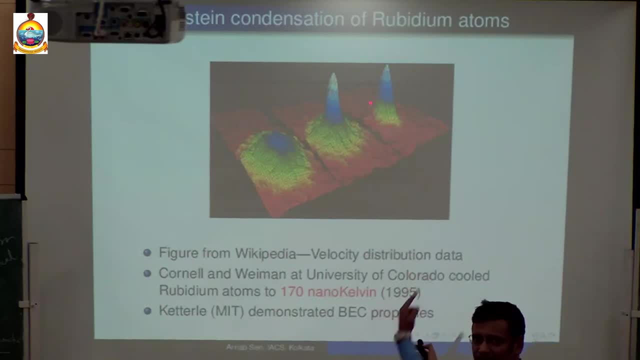 And that actually shows up in this blue guy spiking up Right. So see, here this is sort of at an. this is like near this Tc, near this Boh-Einstein condensation temperature and this is below it, and you can see that this guy is spiking. 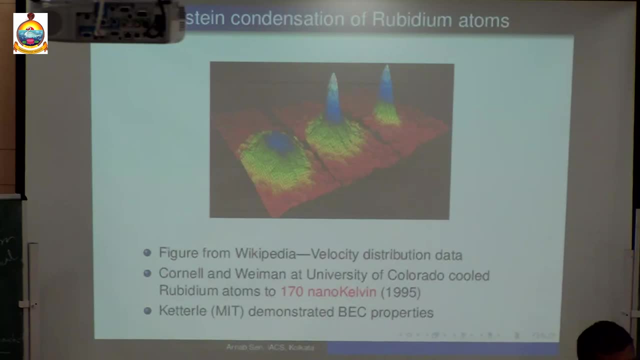 up Right. So it is really eating up all the weight of the Gaussian distribution, Right. And this was sort of the first experimental demonstration of the Boh-Einstein condensation by these gentlemen, and of course they were soon awarded the Nobel Prize for this. these 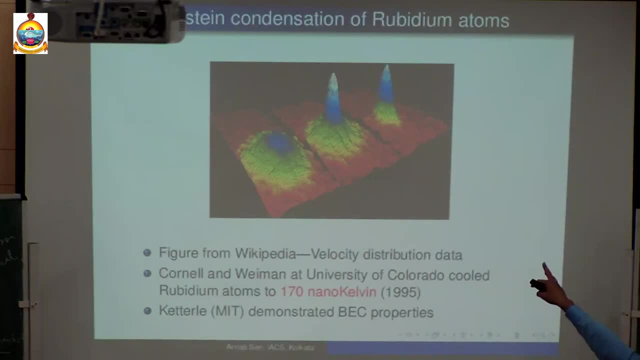 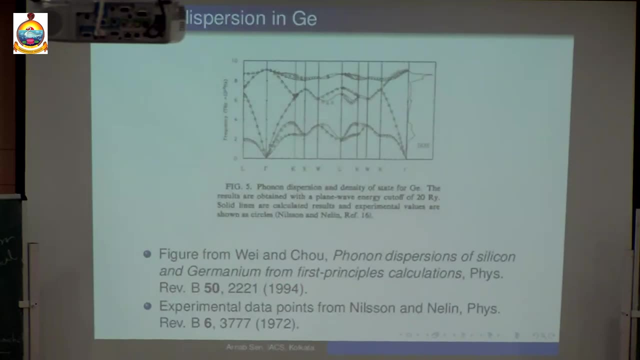 three gentlemen, Right, So? So we have to learn how to think about these things, Right? But today we will just first, in this lecture, we will just focus on this and its consequence. Good, So now, I do not need this. Now, I will just go to the board. 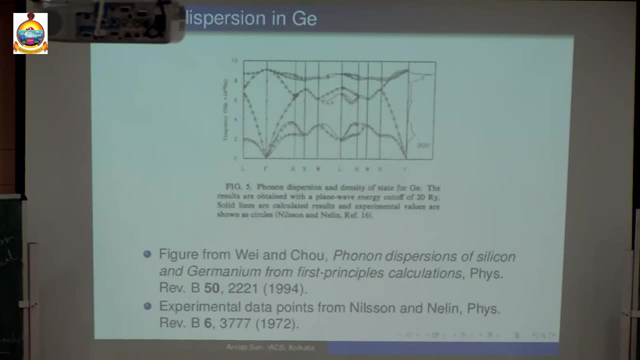 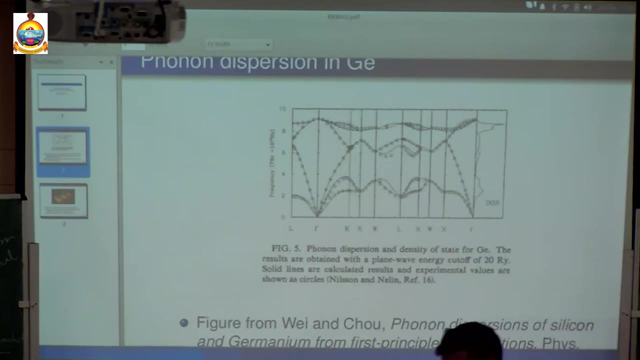 So can I? how do I switch it off? I mean No, but oh, I will leave it. Oh, it does not create any problem for the recording, Right? Okay, Then it is okay, I can leave it. But look at the board. 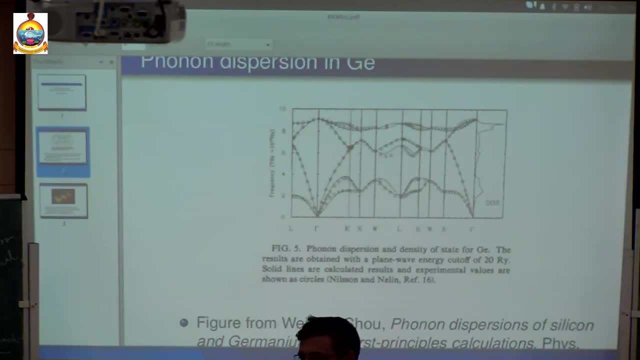 Do not look there Right. There is like: how can we get such? so it is so exact, right. What, Oh What are required to? Yeah, yeah, yeah, So okay, So right. I mean they, of course. 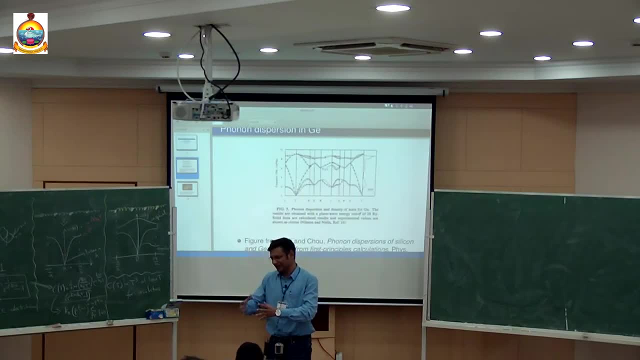 So there is a complicated lattice. At one level they did some harmonic approximation, But then they had systematic waves, ways of improving on those harmonic- what should I say- approximations. So they took It is like you have a unit cell and they sort of keep enlarging their unit cell. 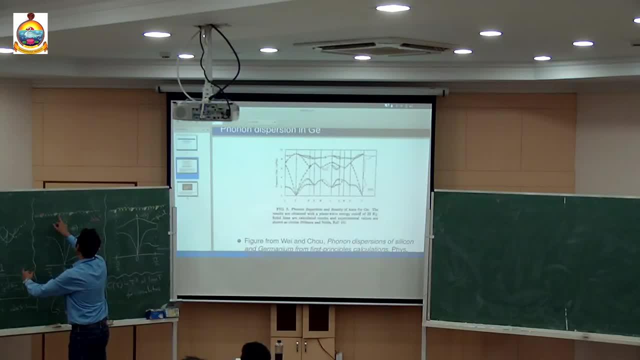 And then they can. So now you say: oh, maybe this is my unit cell and I should consider more interactions. Then you get more structures emerging and so on and so forth. So there is some systematic way of calculating that. I, frankly, have never done that myself. 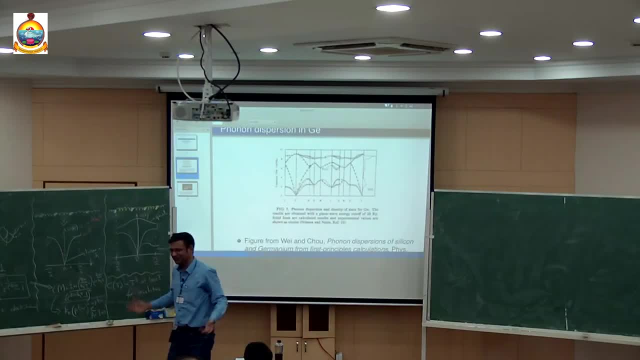 Because I am just happy to see this thing and I know that I roughly understand it. That is it So. But there are systematic ways of. These are called. These are called ab initio methods, Yeah, But Yeah, There is a huge community which 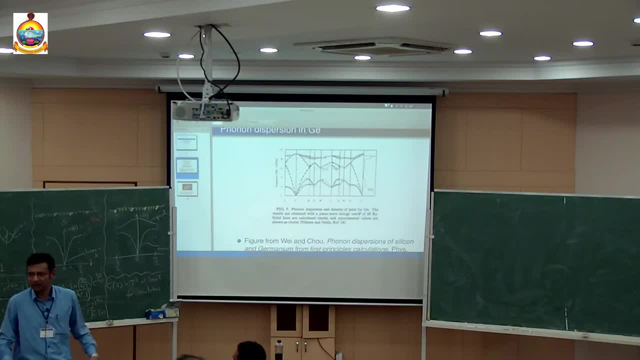 In this paper. No, no, no, So the theory was already developed. These two authors, Wei and Chao, They actually applied it to this problem. Yeah, Yeah, Yeah, But there is a big community which works on that. 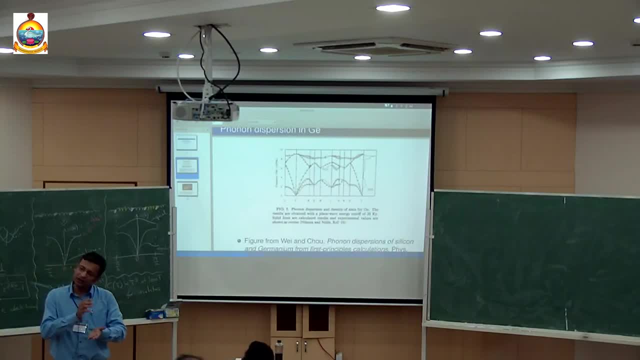 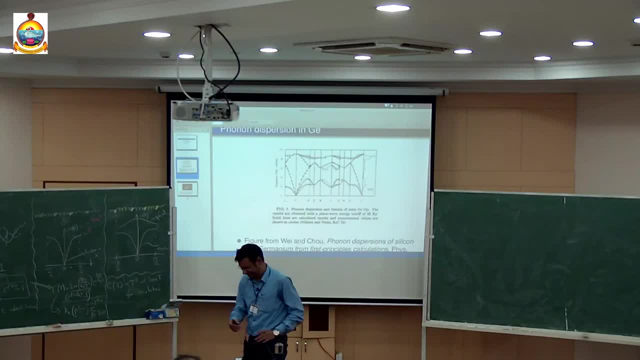 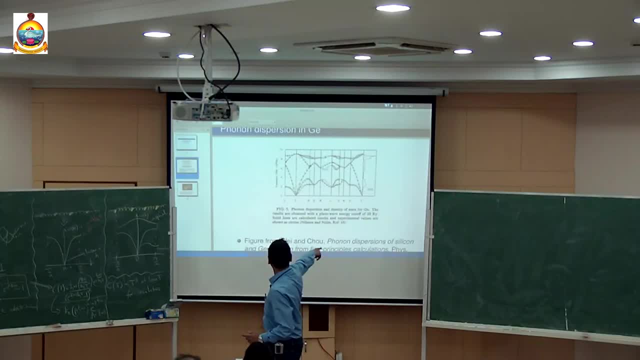 There is a. There is a. I mean, if I worry about all kind of things, Then I mean You cannot be good at everything And you cannot understand everything. That is it So Right? So I can recommend you this paper. 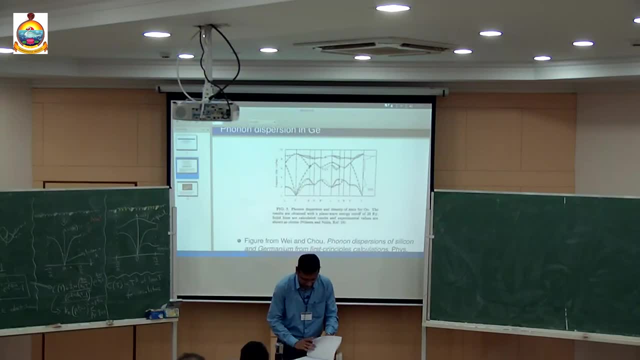 And you can read it. Yeah, That is it. Yeah, Good, So now we will go to our calculation on this board. I will keep this here: homework assignments. They are both very simple, So please do them. I mean, it will be to your. 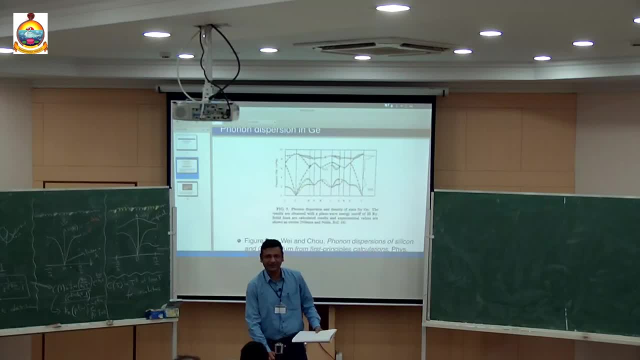 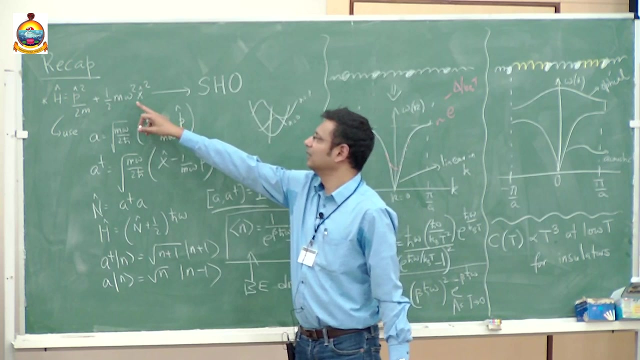 own benefit, and if you are stuck you can ask me tomorrow and I will try to help you, But hopefully you won't get stuck. So one of the questions which I got during the discussions after my lecture was what happens if this harmonic oscillator is not harmonic? Maybe? 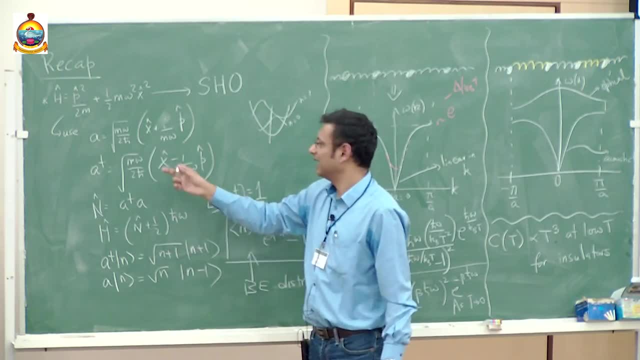 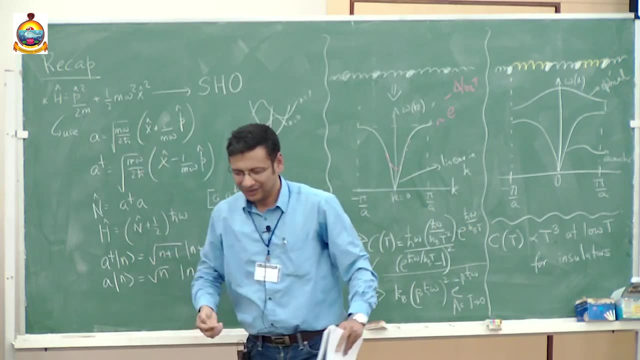 it is anharmonic. Of course you can still write this representation and the nice advantage of this representation is, as PK was also indirectly saying in his talk, See, once you have this algebra, you may. you don't even need to know the wave functions explicitly to calculate. 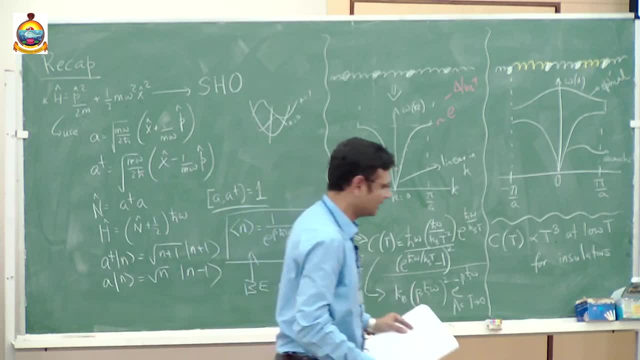 many things. So that is the power of this representation. So let me give you one small problem first, to calculate which you should do at home, and please try to do it today, and you can then tell me tomorrow. We can discuss the problem more tomorrow. 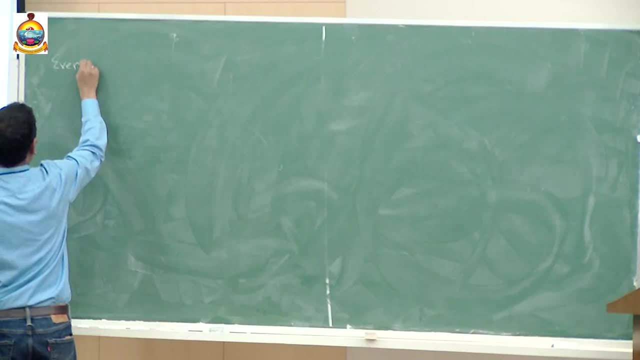 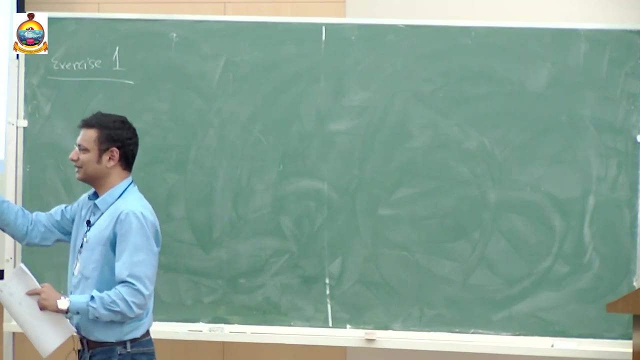 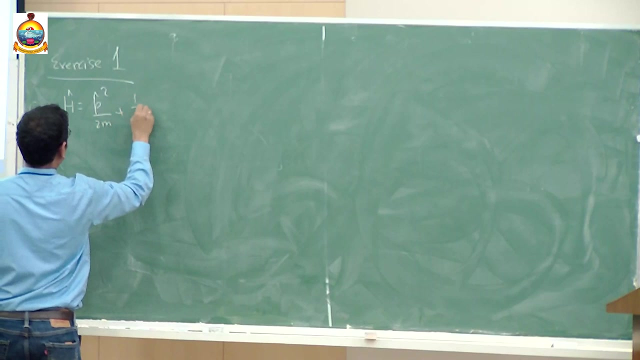 So this is exercise 1.. I mean, of course, if you do these simple exercises you get more hang of these things, because otherwise they might look very- what is the right word- abstract to you. So now let me just define this oscillator problem with exactly the same parts, but I add: 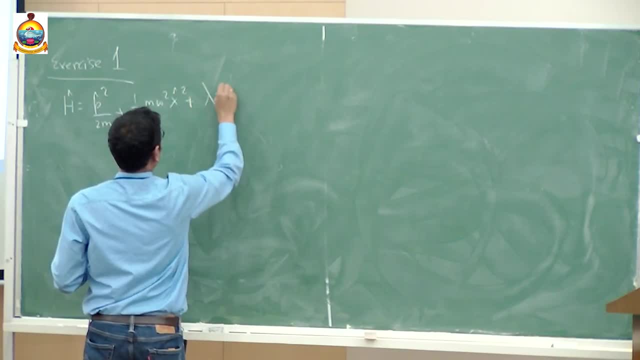 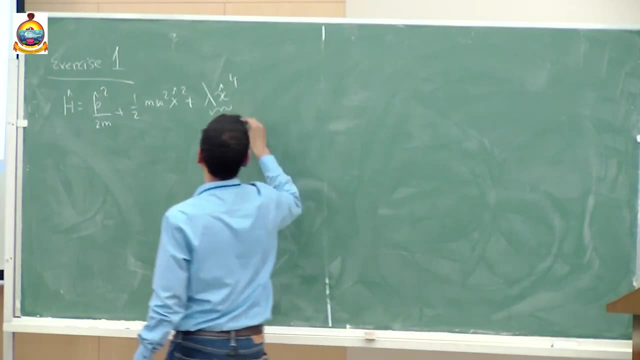 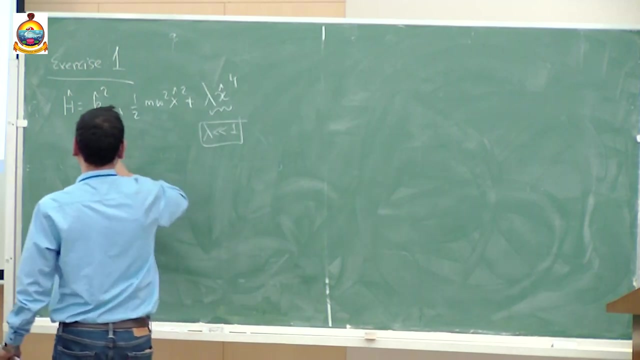 another small piece. So the small piece is this term. So this makes my oscillator anharmonic, and I further assume that lambda is much, much smaller than 1.. So then, what I am asking you is, of course, then, if this happens without this term, you know that the energy of each 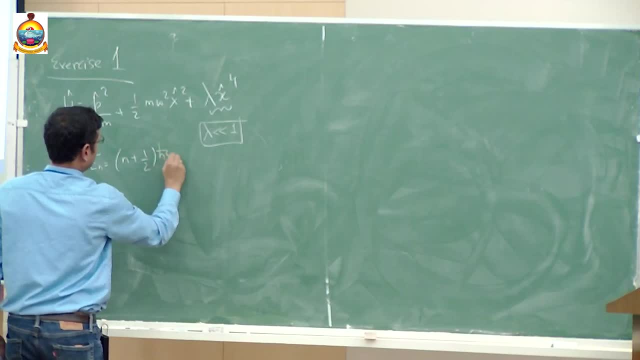 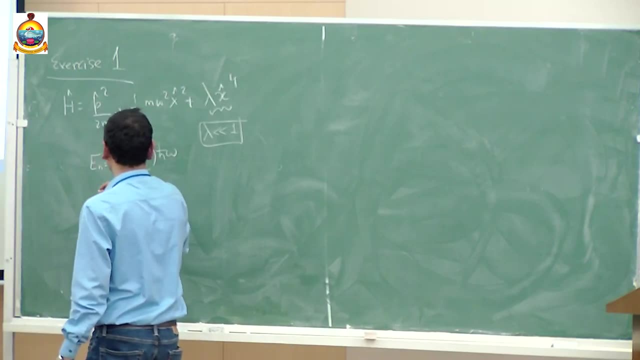 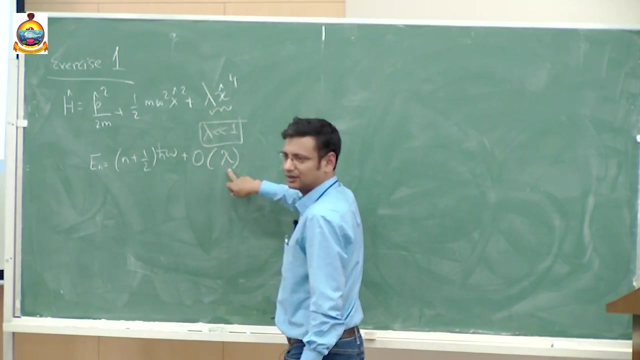 eigenstate is this, But with this term, of course, the energy is going to shift slightly. Now my question to you is: calculate the first order shift in energy, So the term which is order, this perturbation, So that is the first order shift in energy. but calculate it using 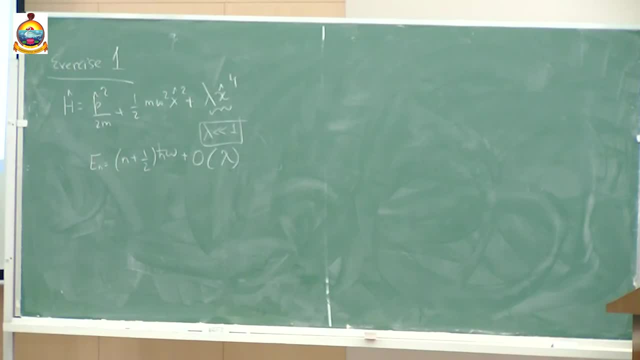 the method of a and a dagger. So that is very easy. I mean, I can just give you a quick hint and then you can try to do the calculation. Essentially, this shift boils down to- of course you need to insert factors here- Boils down to calculating matrix elements of this form. 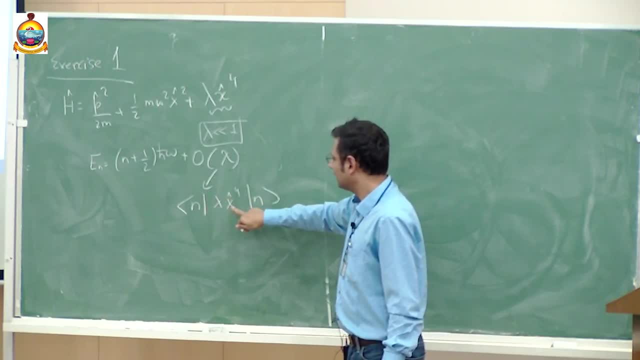 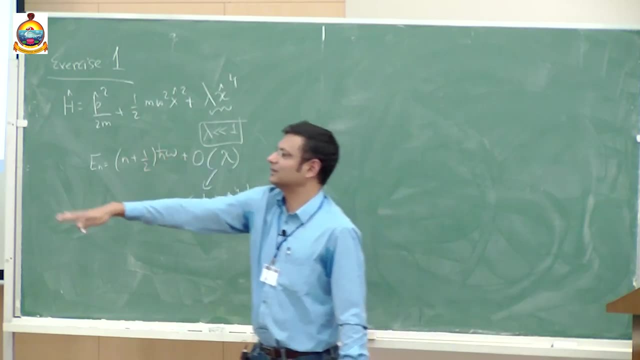 Matrix elements of this form from first order perturbation theory. What I am asking you is: please express x in terms of a plus a dagger, and then just use the commutation relations that we have written there, And maybe you can also note down these two relations And. 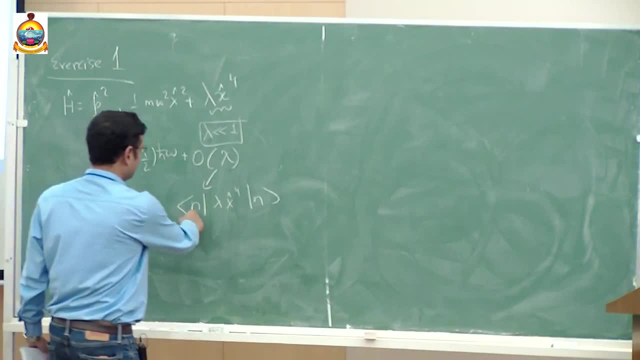 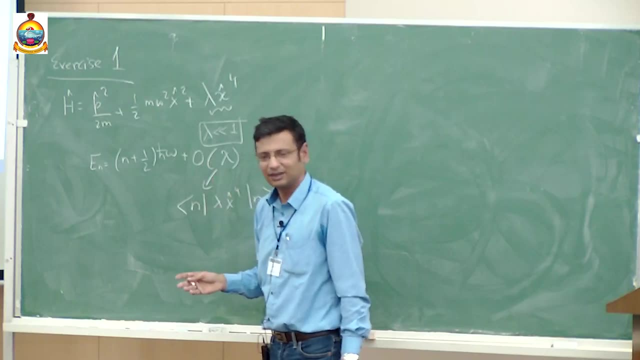 just using this, without even explicitly knowing the functional form of n, you should be able to derive this correction for an arbitrary n. So please try this and it will be helpful. So that is exercise 1.. Everybody understood the exercise. We can deal about how to do. 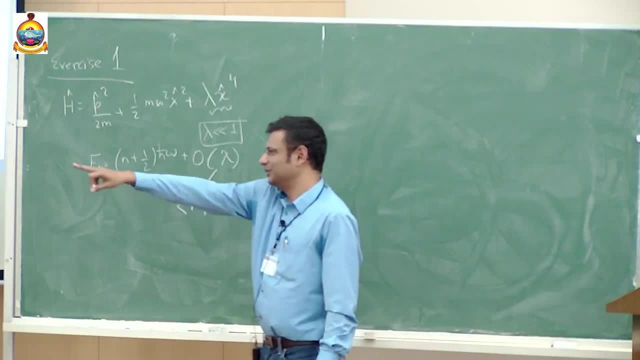 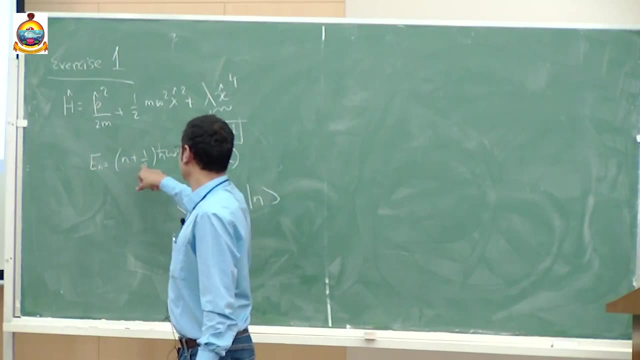 it later, but you understood the exercise, So you should use that technique to do this problem. Of course, when you write this in terms of a and a dagger, you will see that this problem is no longer a free Hamiltonian. It has sort of a dagger, a dagger, a, a kind. 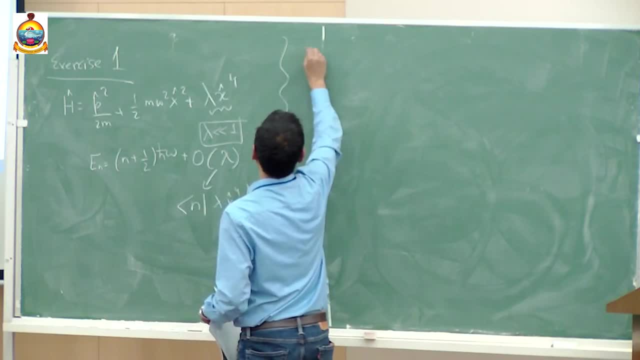 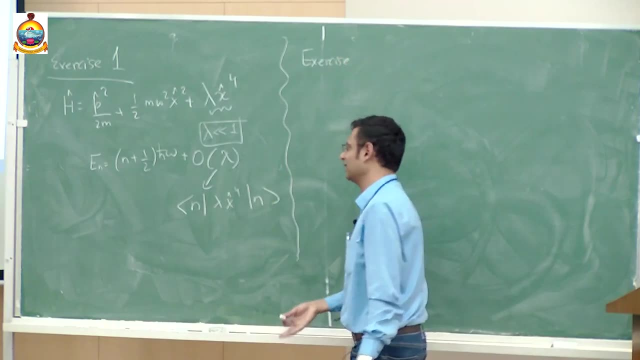 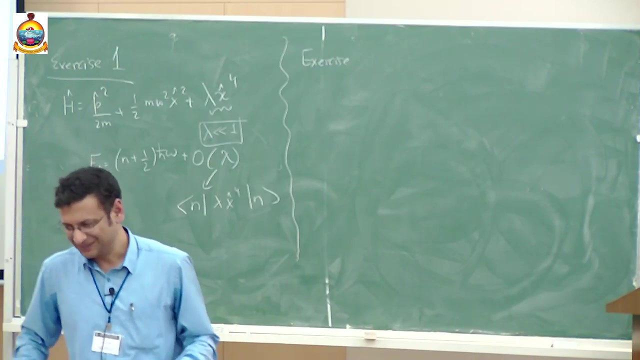 of terms and so on, And then I will go to the lecture. Okay, and I am giving the exercises to you now so that you have some time to do it, and then we can discuss it tomorrow, Right? I mean, I mean, this was my problem, So I am a very slow person, so normally when there used to be these, 1 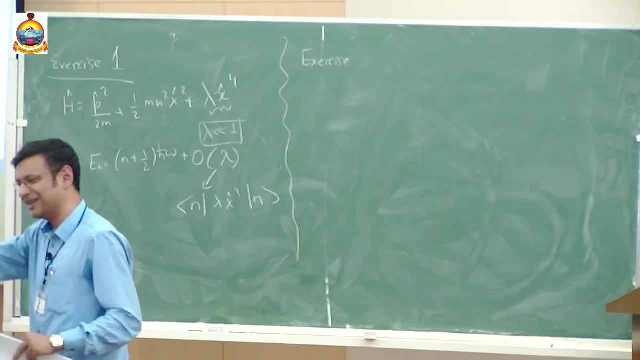 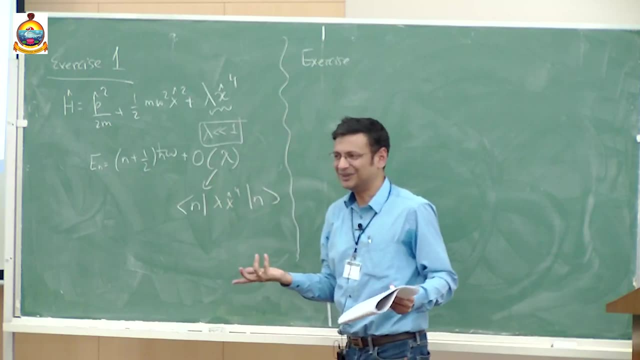 or 2 or 3 hour exams. I used to be very terrified, But somehow I managed through my school and college education okay So. But you see, when you go to your room you will have lots of time. you will have nobody staring up upon you. 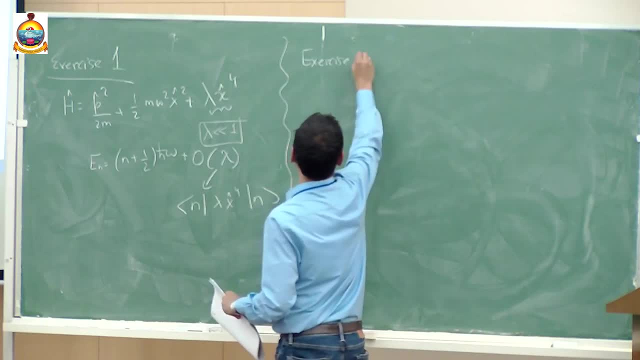 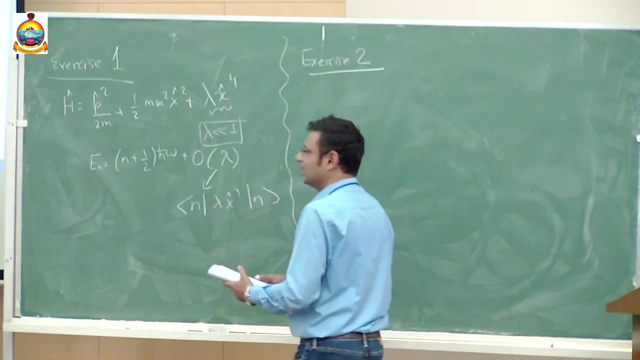 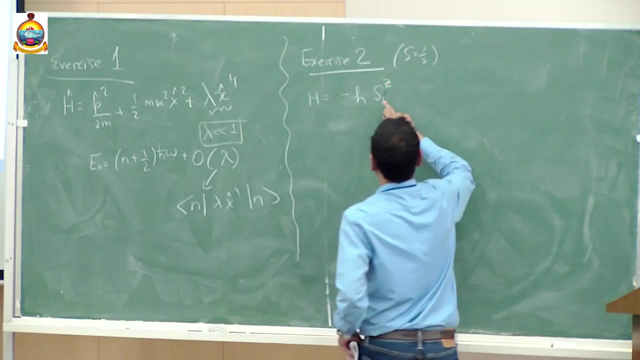 Subtitles by the Amaraorg community. So then you can do this right. So exercise 2.. Exercise 2, is you remember? so spin half. and it had a very simple Hamiltonian, sorry, which was this. I put a label 1 for a certain reason. now, 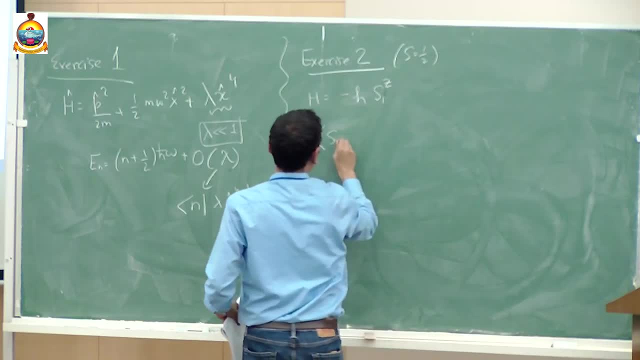 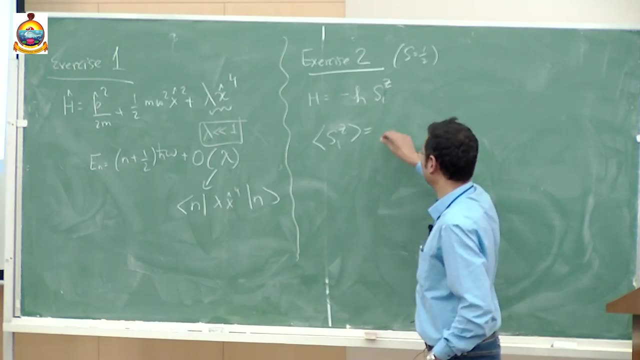 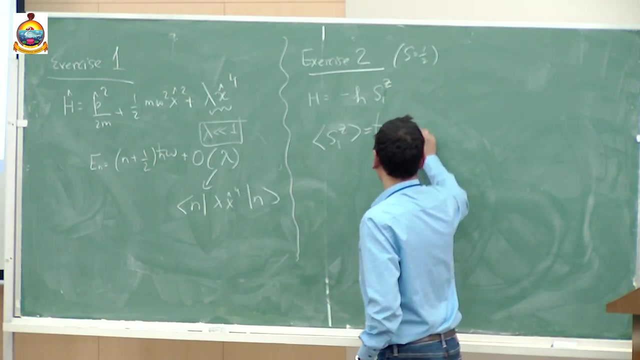 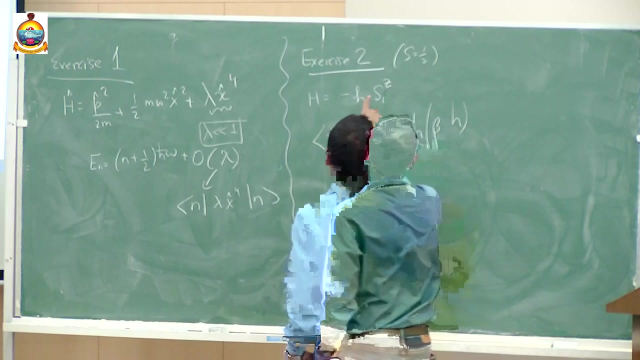 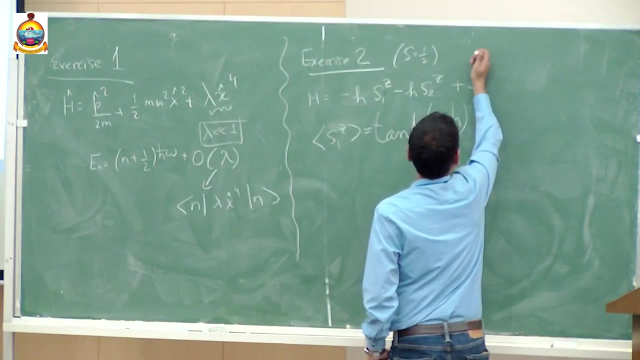 So then we calculated for this that S1Z expectation was. can somebody recall what the result was? So this is some very standard result. yeah, tan, hyperbolic, I hear murmurs- right, So this was the result. good, Now two spin halves. so then there is another term here. now I add a third term here, sorry, 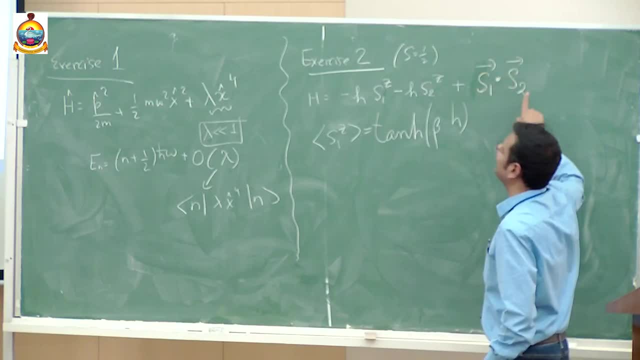 S1, dot, S2, with a plus sign outside. So this is like an anti-ferromagnetic interaction between spins. Right This term. So you understand what this term is right. So this term is just in terms of these quantum operators, it is just S1Z, S2Z plus S1Y, S2Y. 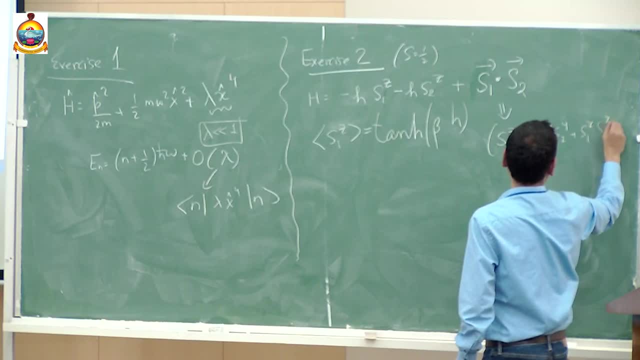 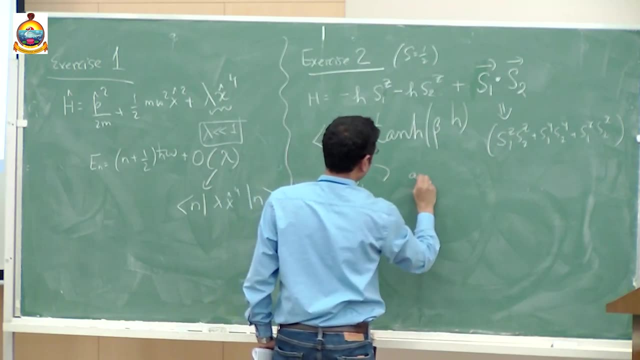 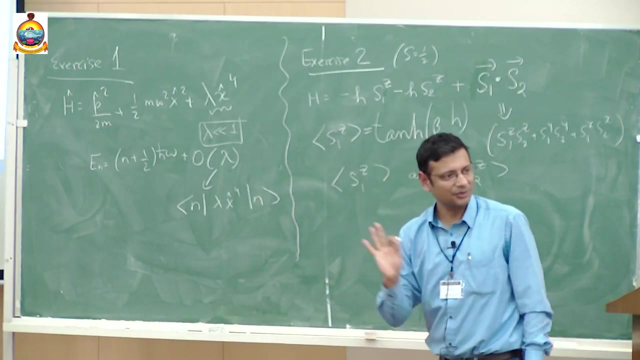 plus S1X, S2X. So please calculate the partition function for this and please also calculate what is S1Z and S2Z right? Good, So again you understand to do this yourself and then try to understand the various limits. 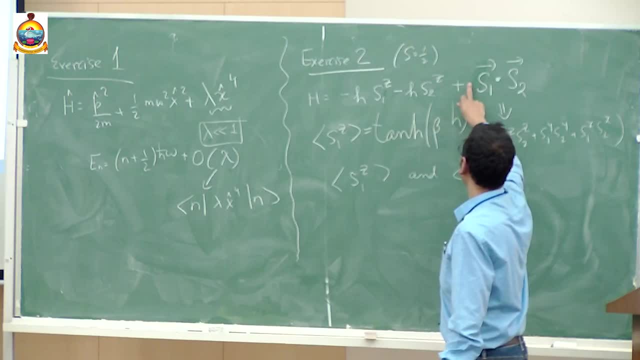 of this beta and H, and there is also another factor here, J, if you wish, But I have put J to be 1. What defines small and what defines large, and so on and so forth. Okay, So these, but so far, so good. 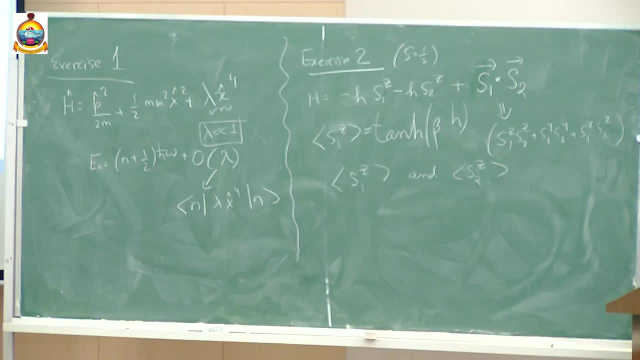 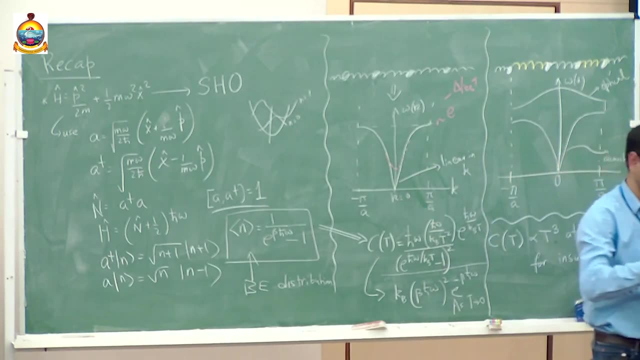 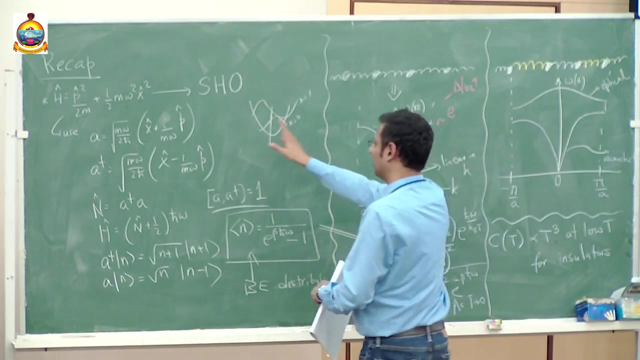 Anybody has any problems. So afterwards I realized that there was some confusion. There was some confusion with this derivation, and why Now, today? let me give you an alternate derivation, very quickly. So it is a very small alternate derivation, but right. So now I will erase all this, right. 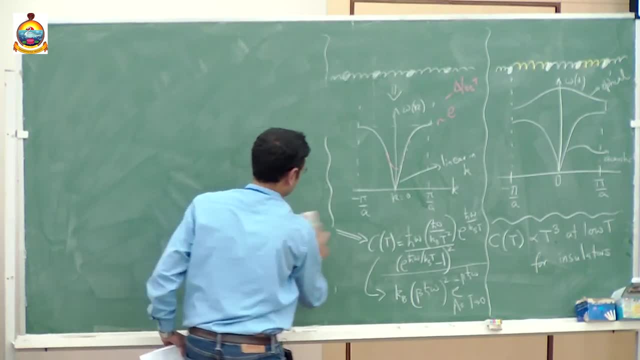 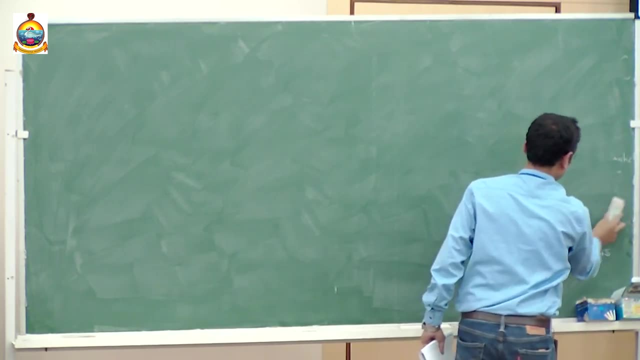 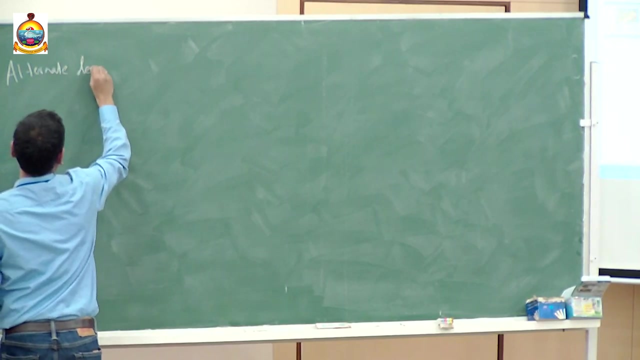 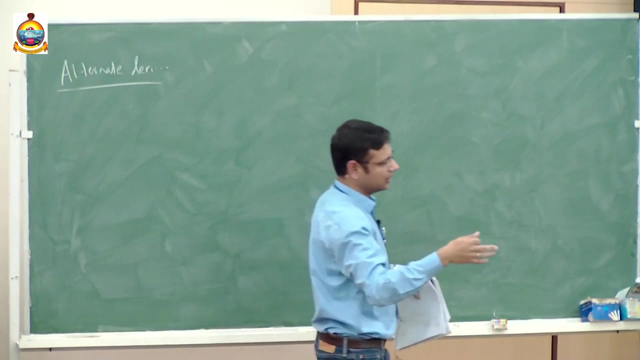 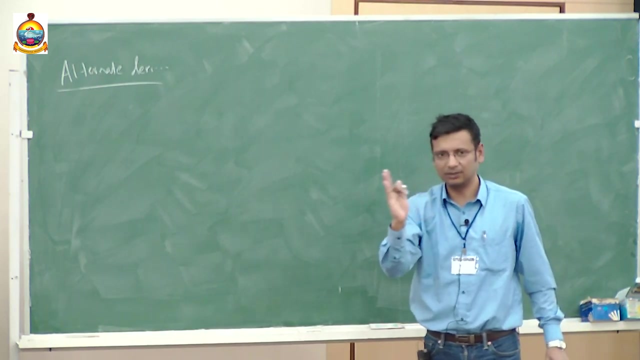 I yeah, okay, Let us do a alternate derivation. Okay, Alternate derivation for for whatever we were tackling yesterday. So I said that the situation that we are imagining is that there is a crystal and basically the atoms of the crystals are doing small fluctuations about the equilibrium, right? 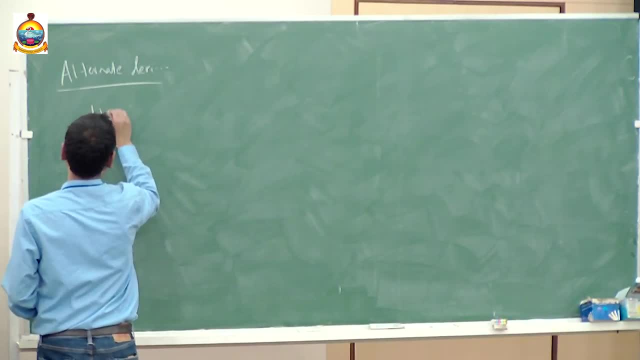 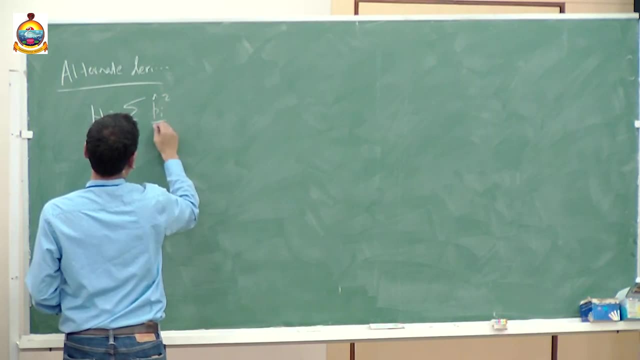 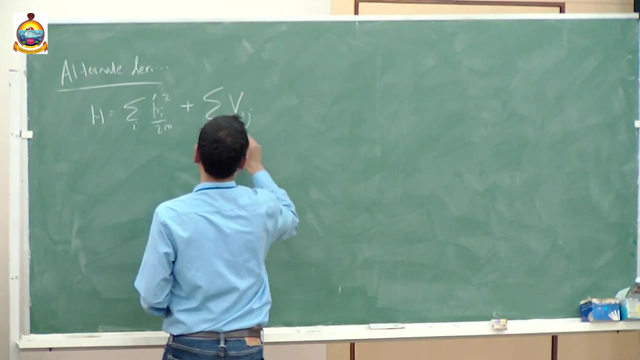 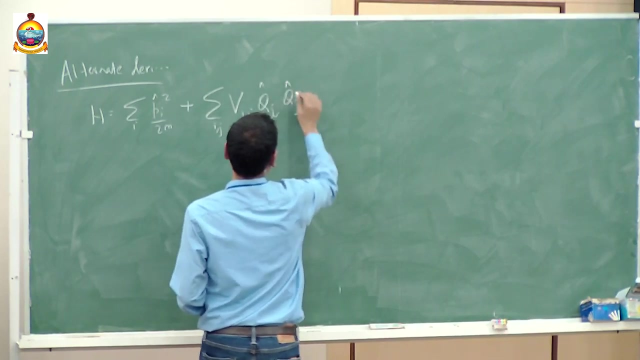 That was the model. Now, because the key word is small fluctuations, I could therefore write a quadratic theory. So, basically, there is a kinetics, Okay, Okay, There is a kinetic term, right, And then there is a potential term, And these- okay, these fields are, if you wish, the displacement fields. 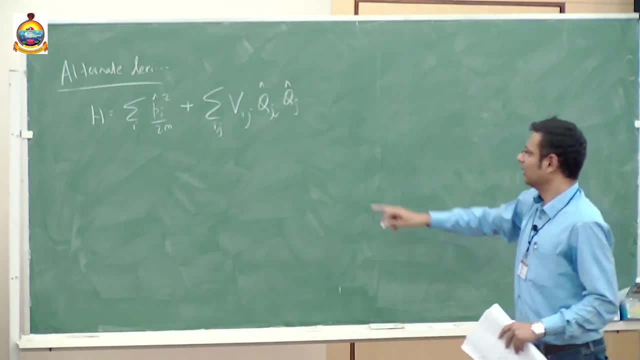 So the displacement from the equilibrium position right Now. of course I stopped at quadratic order. So first question: why is there no linear piece here If I expand around the crystal positions? why is there no linear piece? Yeah, because it is at equilibrium. 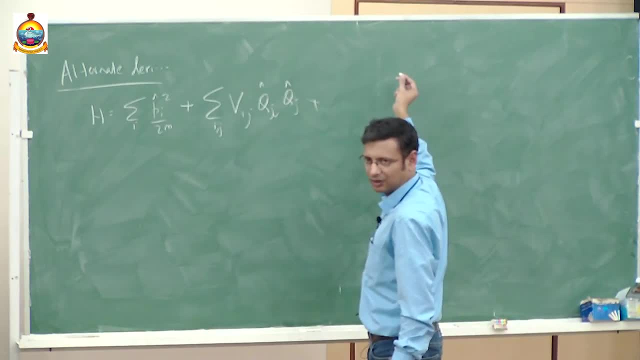 So the first piece I will encounter is this, And of course I will encounter higher order pieces: right Order, so this is a shorthand: Q cube, right, So three Q terms, Q4, and so on and so forth. right, 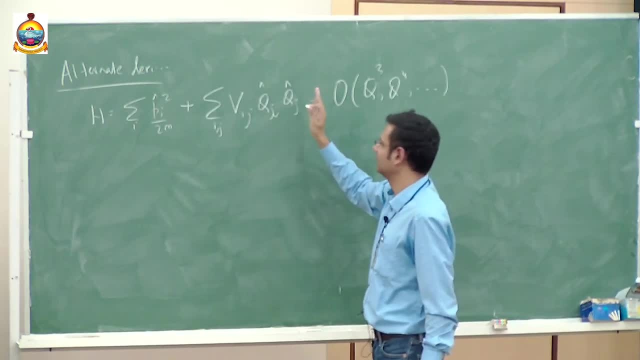 But in the sense of a Taylor expansion. this is the first term I will stop at right, And this theory is a is a free theory, right? So we can write them in terms of normal modes. So let me very quickly tell you what I will do. 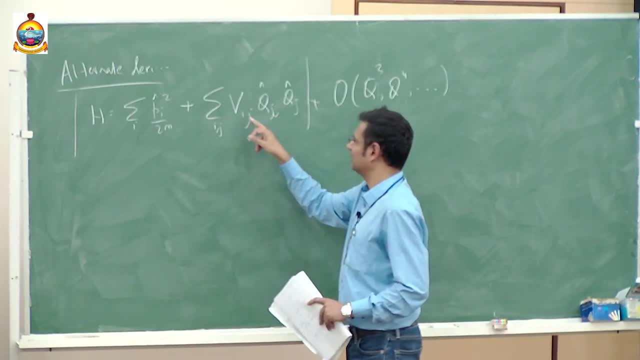 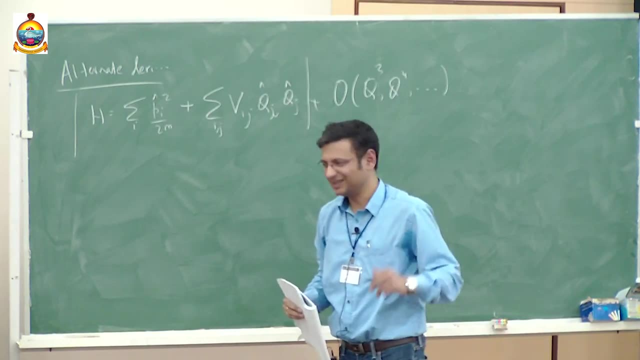 Okay, Okay. So what I would do in terms of this? and basically, I will just recast this as a problem of matrix diagonalization, and in the last two classes of PK, you have heard many things about matrices and their manipulation, So you are all masters of matrices. 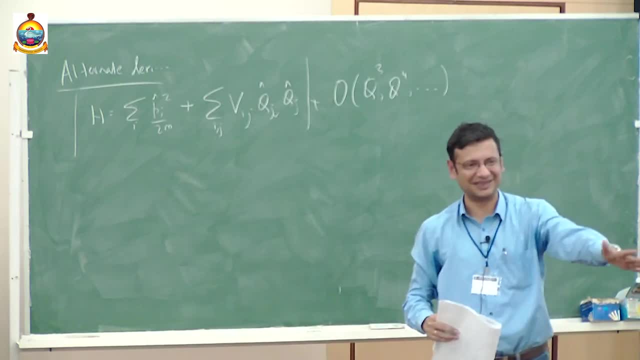 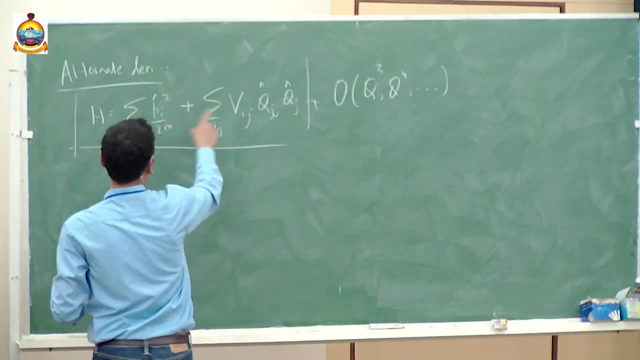 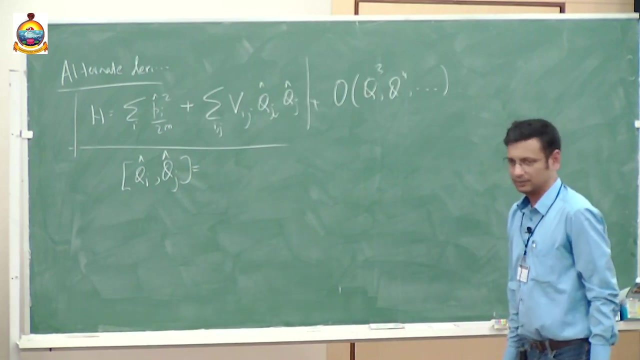 So from now on, I will try to cast everything in terms of matrices and then everybody would understand, right. So right, okay, good, So here, of course. first question is: what is the algebra of these classes? So what is this? What is on the right hand side of this? 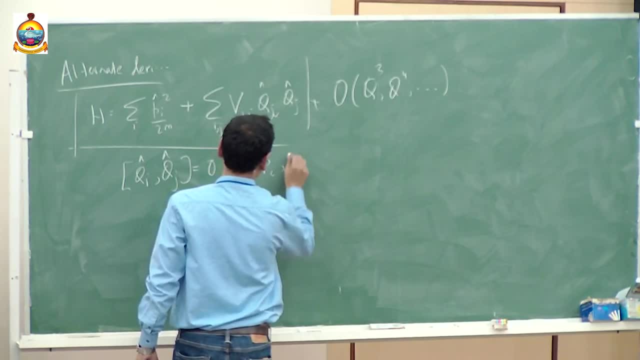 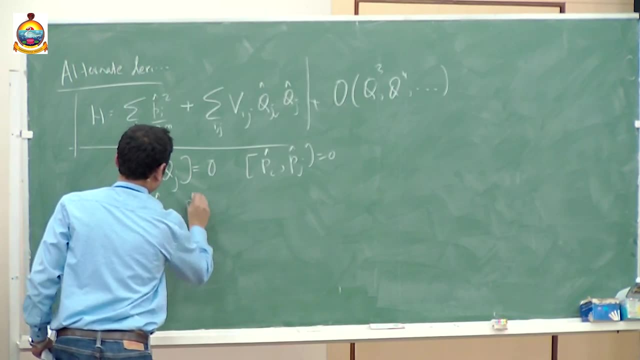 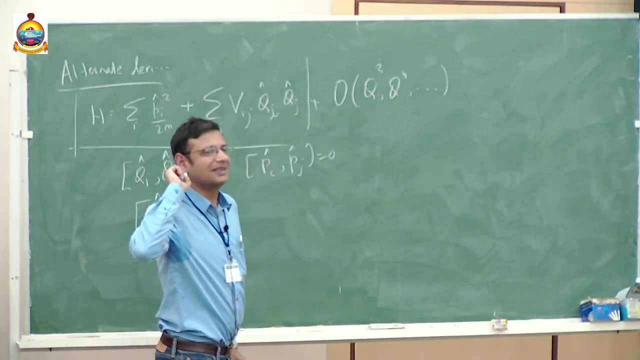 Yeah, that's correct. So, similarly, this is also zero. right Now, what is this? I didn't even finish it. yeah, What is this? Huh, No, But there is also something Before delta. What is delta ij? 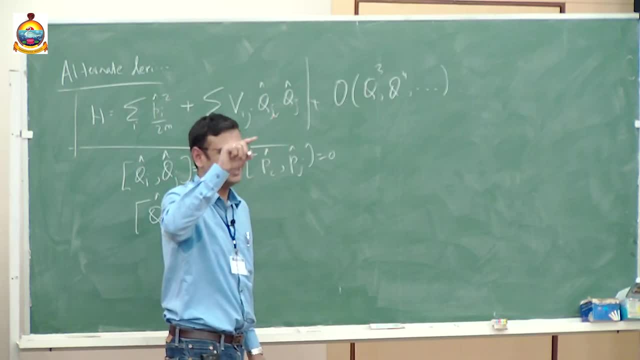 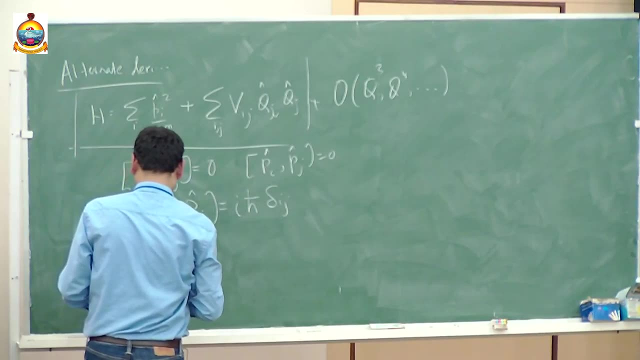 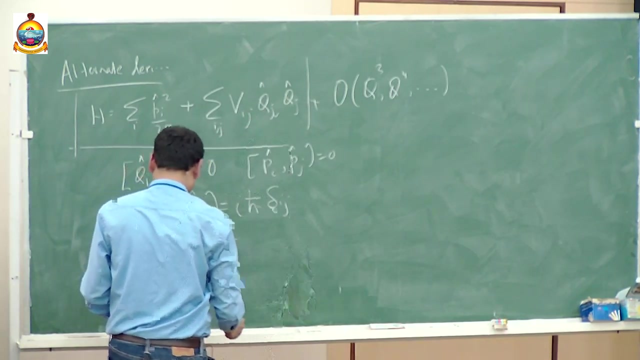 Huh, Right, right. So please don't forget factors of i and stuff like that. right, i h bar delta ij, right? So the format is this. So let me just do this casting So: Q, scaling these displacement fields by square root, m in the denominator. 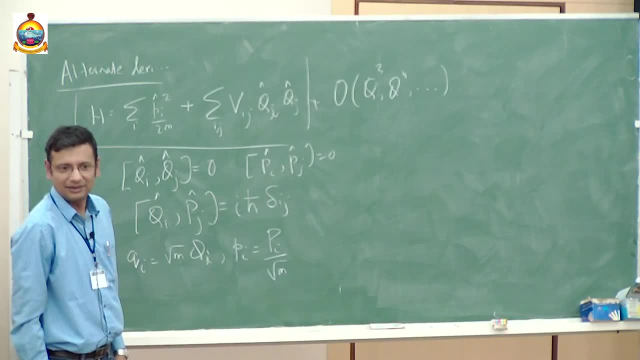 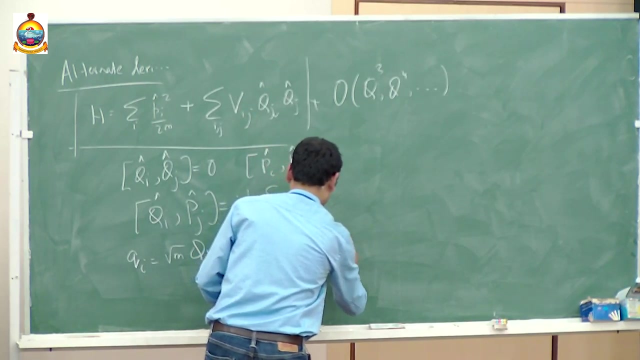 Why didn't I put something like an m, for example, in the denominator right? Because I want these new variables to also be new coordinates. New coordinates and new momenta right. Some redefine, And okay. the last thing is I need, instead of vij, I'll define a uij. 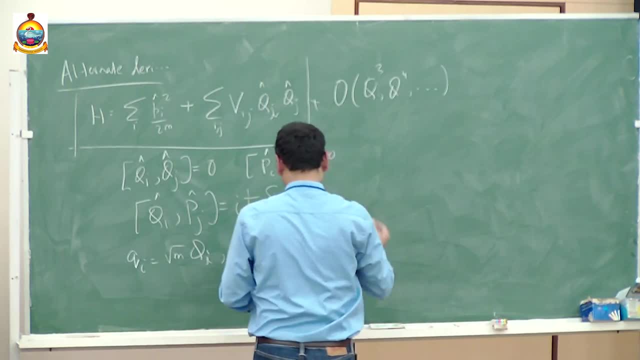 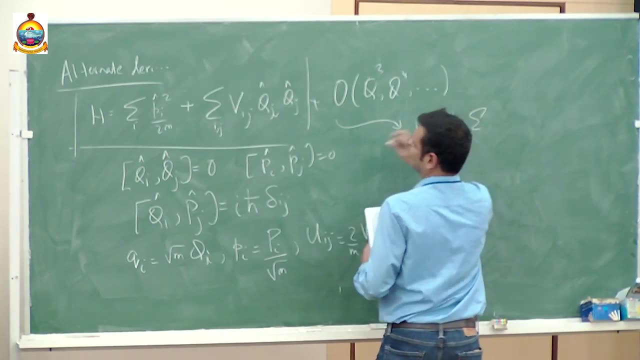 And this is very straightforward. So if you do all this, then your Hamiltonian just becomes slightly simpler. that's all I mean. it doesn't have these factors of m and all sitting. That's the only reason I did it, Okay. 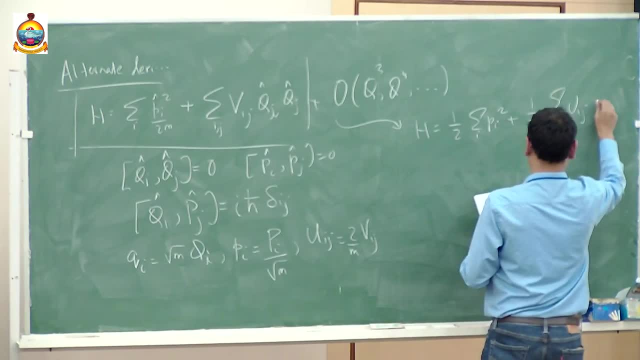 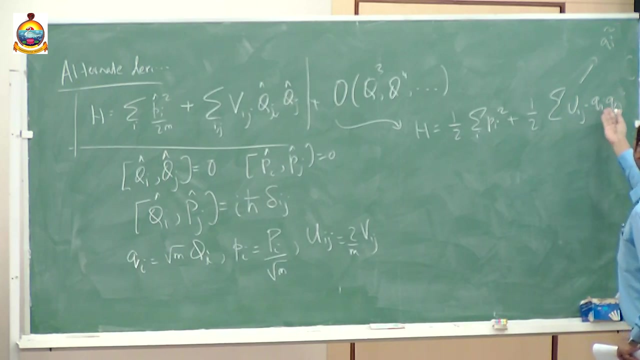 Okay, So this is your Hamiltonian. Now you can see what's going to happen, right? See, this thing is yet not in the harmonic oscillator form, right? This is not in the form qi square, right, But this is exactly in a matrix form, right? 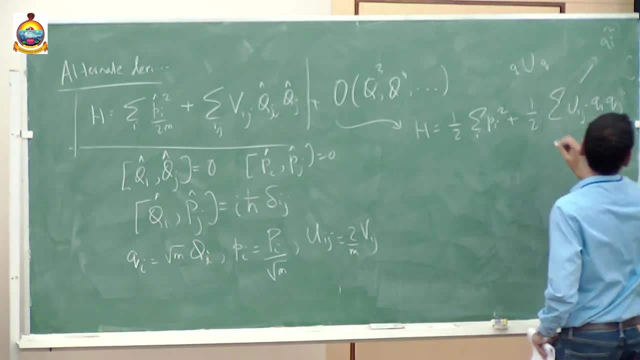 If you think about it. So there's a q, there's a u and there's a q, And this u is a symmetric matrix, right? This u is a symmetric matrix. So then of course, you can do a similar. You can do a similar transformation and just go to another basis where there are some tildas. 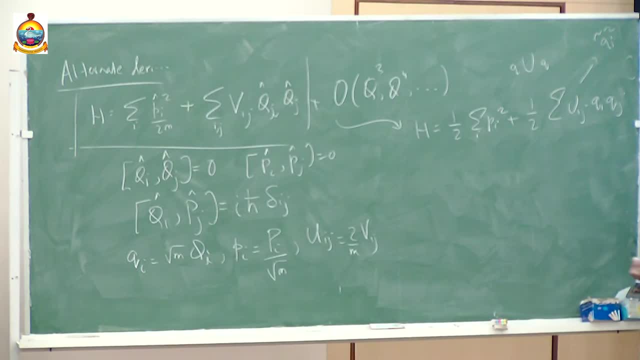 and then the matrix sitting in between becomes tight, right? So that basis is your normal mode basis. That's it, End of story, right? So hopefully this is less confusing for the people who got confused in the first approach, right? So then we just write that thing. 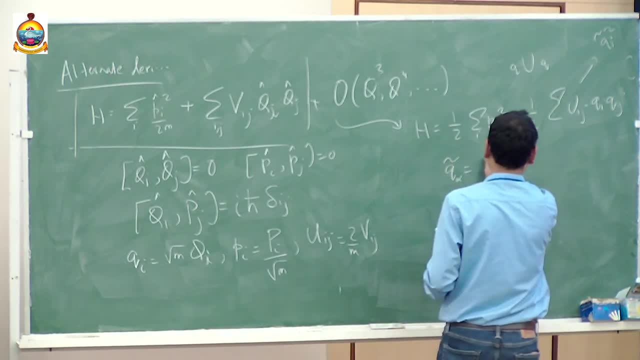 So there is some linear transformation, yeah, which you know how to get, which just depends on this definition uij of this matrix Okay. So there's some linear transformation here which is like that. There's some linear transformation like that. 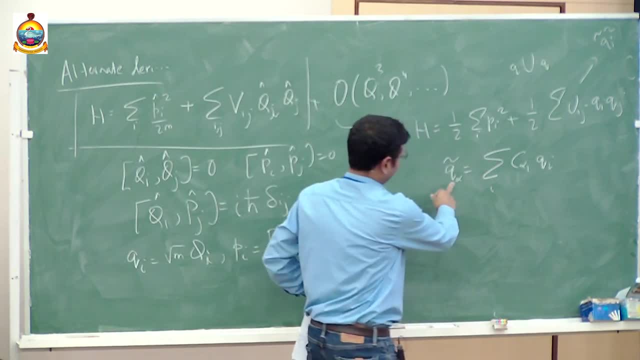 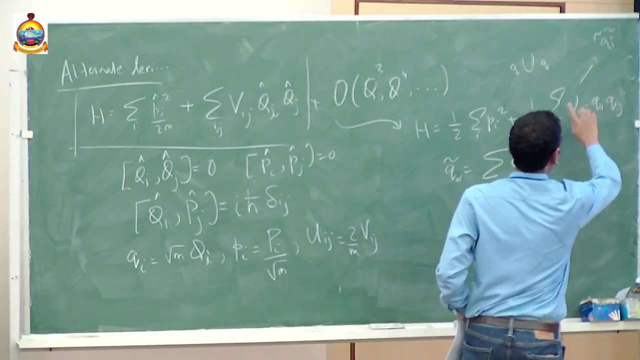 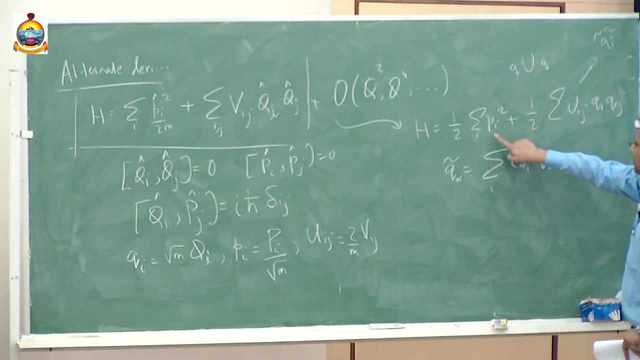 Good, Okay, First question: If I want to go to this q alpha tilde, right, Of course, then this thing becomes quadratic, right, This thing becomes quadratic and in terms of q alpha tilde, whole square, right. But should I do something here? 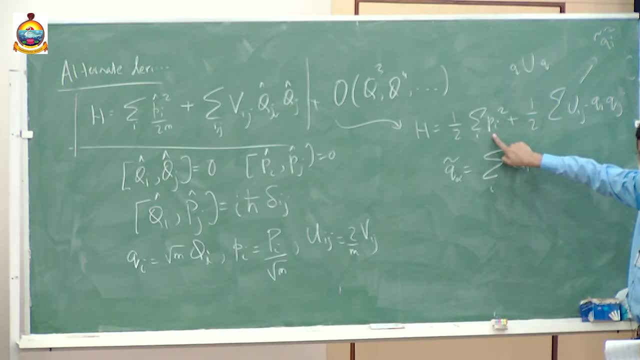 What do you think? This is already quadratic. but should I do something here? What do you think Do I have to do? i don't know. sure will be preserved, are you sure? so try to see the commutation relation of this object with pi. you should try this, and it won't be preserved. so i have to. also, i have to. 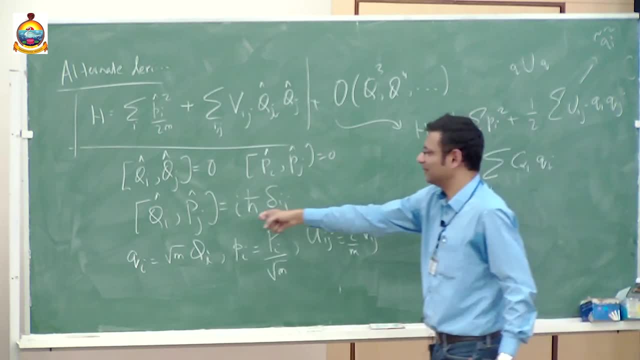 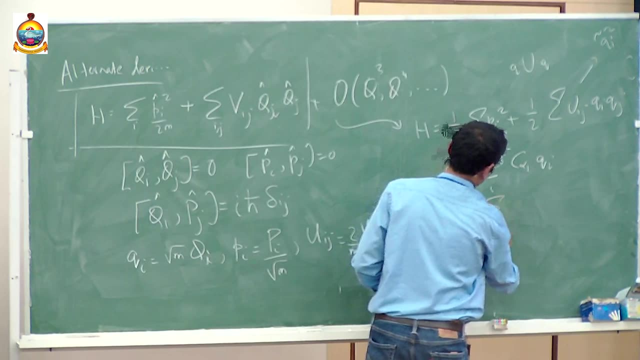 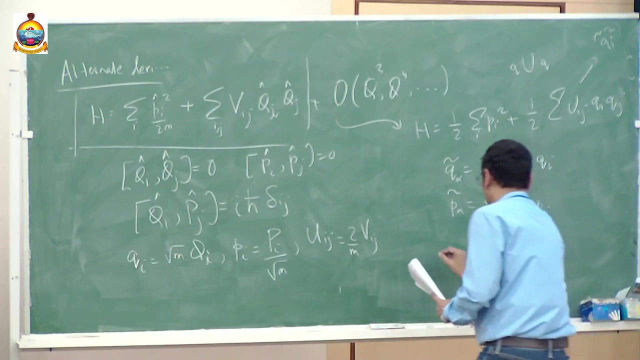 also transform my pis, because i want to again preserve my commutation relation, right? so yeah, so you just do exactly that, but you already know this. so then you do this right, and then that's it then the general hamiltonian that you get. so of course this matrix would have: 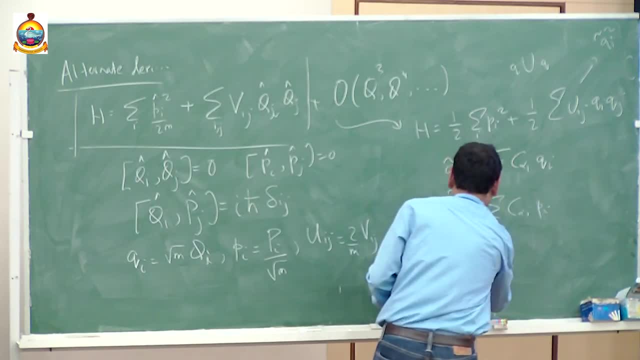 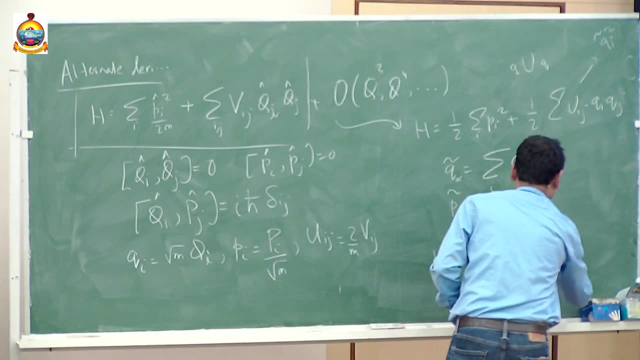 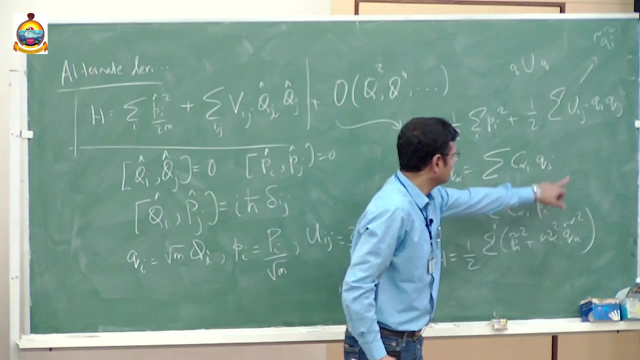 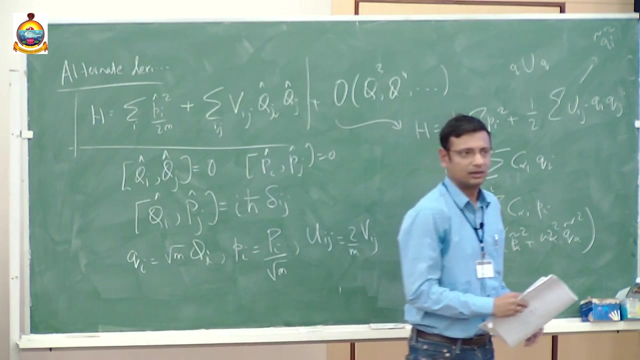 all real eigenvalues, right, because it's symmetric right. so i said that the eigenvalues are real. but why am i also insisting on the fact that the eigenvalues are all positive? uh, does somebody know? i mean, why am i insisting on that? why are all the eigenvalues positive? because i've written some real number, whole square, so that's a positive. 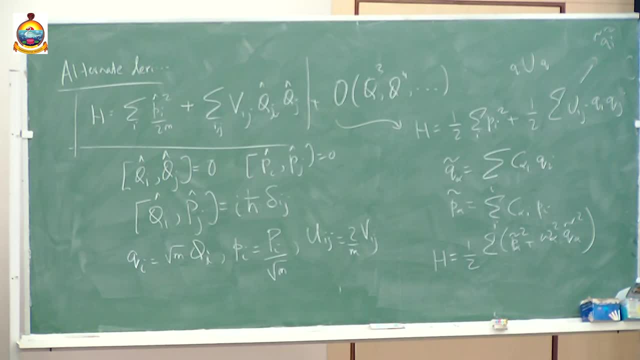 number. so why are all the eigenvalues positive? sorry, no, i mean, it's just, that just gives you the reality condition. why is it positive? i mean, just think a bit, what are we originally doing, and it just comes out from there. no, no, i mean, this is just some mathematics i'm doing here, right? so then see, of course. 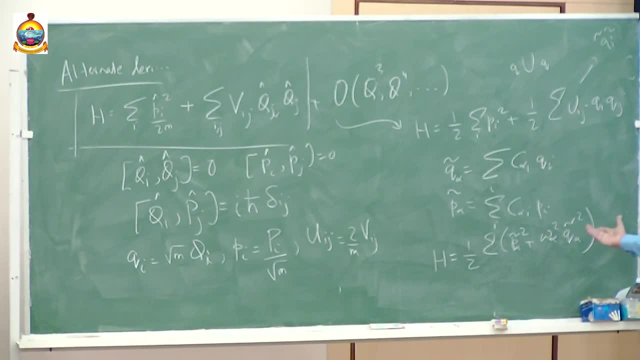 the eigenvalues are all real that you can get from here. i'm asking another question: why they're all positive? no, no, i mean, come on, i mean no, that's you yourself understand. that's not a satisfactory answer, right? so why are they positive? very simple question. just think a bit. 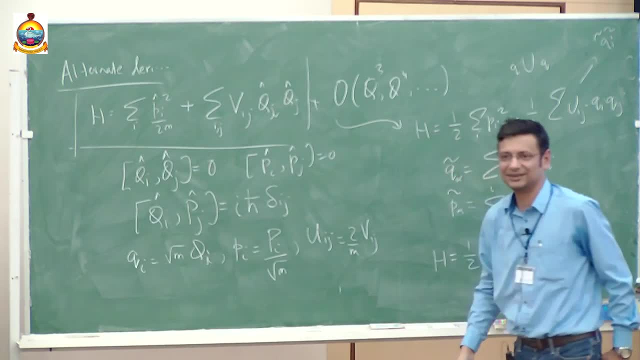 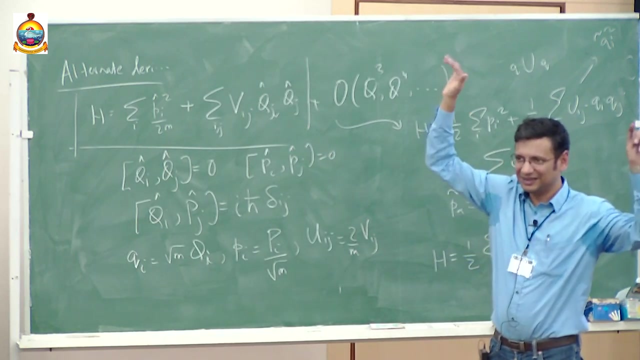 look at this thing, what are you trying to do? and then it's immediately clear. so you are expanding about some state. what is that state? no, no, no equilibrium or the minimum energy solution. and you're expanding around that, you're perturbing around that. so of course, all the directions should be restoring. so all these 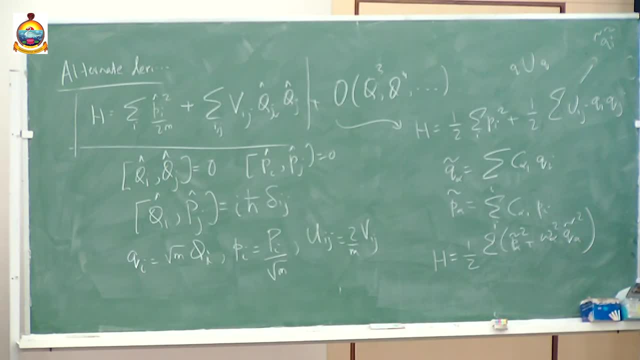 numbers should be positive. if any of these numbers is negative, in fact, that's a good point, see, suppose, suppose you took a problem and you said that this is my equilibrium and i, let's now ignore the square, some of these numbers, you get them to be negative. 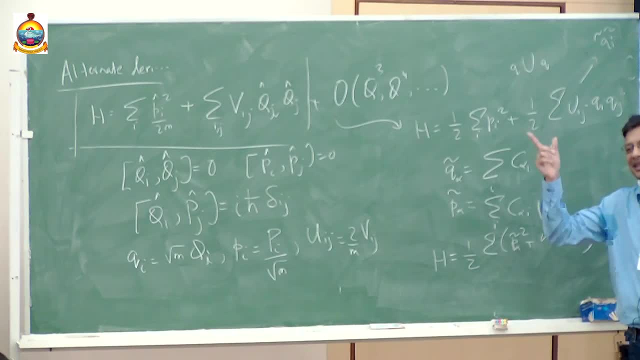 then what does it immediately tell you about your? so that's actually a good check of even your calculation, right? i mean, somebody say you start with the wrong state and you do an expansion, then automatically the theory will tell you that your expansion is one of them is negative. 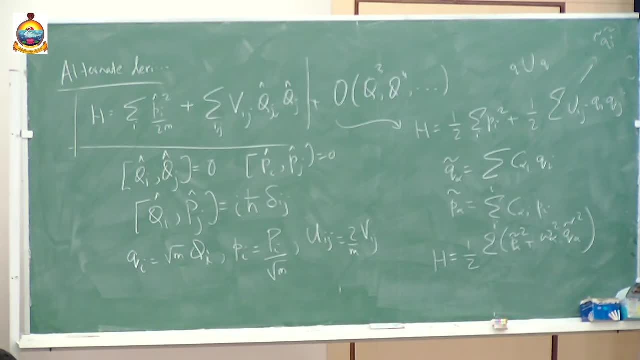 that's enough to tell you that there is some other state which is lower than the state, right? so please remember this, because sometimes, when we do a lot of mathematics, we don't- uh, yeah, we tend to even forget some simpler things, right? but yeah, this is a very simple fact, okay, good, so then we are back to square. 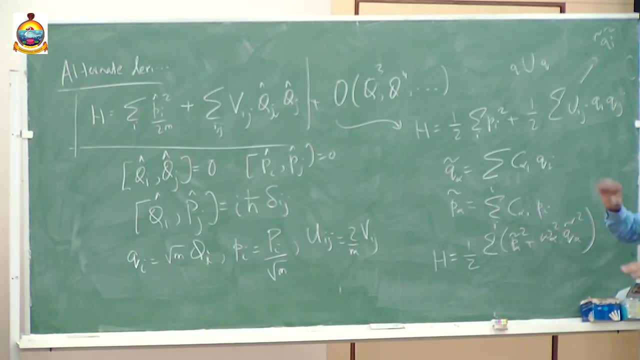 one. then of course, you see, i'm back to the problem. i started with bunch of non-interacting harmonic oscillators because now this is one harmonic oscillator, right, exactly like- oh sorry, i erased that, oh no, there it is, etc. etc. and i can get independent harmonic oscillators. 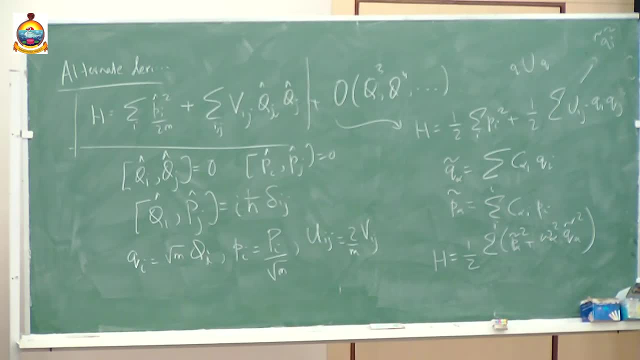 each with this frequency, omega, alpha, right, yeah, so right now. then, as you see, right now the thing is, when you say now, if you, if you can read that, no, no, no, no, no, see, this is a diagonal matrix. so when you do the similarity, transform the diagonal matrix, the identity matrix will stay identity, it's an identity matrix, so think. 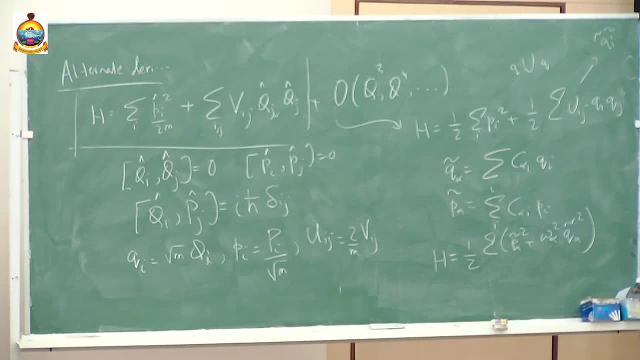 of doing the similarity transform, so it'll stay identity. you can check it yourself. it'll stay identity. yeah, okay, good, so everybody is clear about this. okay, the source of your confusion is c. let me remind you these c alpha i's are not arbitrary numbers. there's. 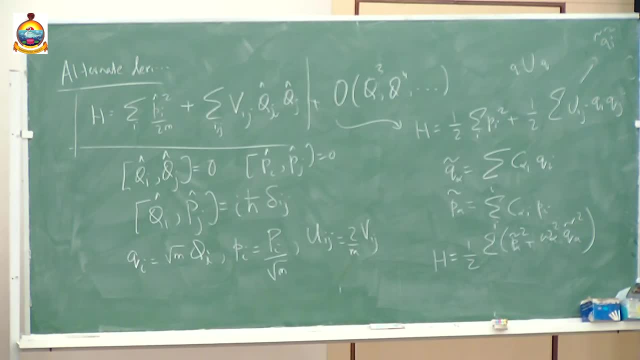 some constraint. i mean, just think of your linear algebra and then it'll come out. they are not arbitrary numbers. okay, good, that's the crystal. that's the crystal, because qi and qj are deviations from the crystal. that's the ground state, right? so here the ground state is easy to guess. but i was 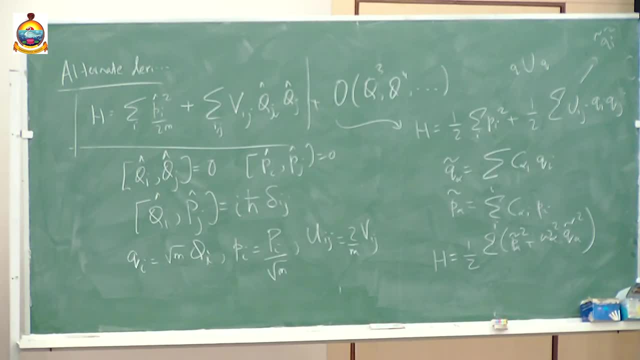 just making a general point, correct, correct, correct. that's the ground. of course, quantum mechanically, yeah, of course, of course. quantum mechanically that's not possible because p, i and q, i cannot be simultaneously zero. that actually has an interesting consequence. so the minimum: see, classically the ground state has zero energy, but the minimum energy for 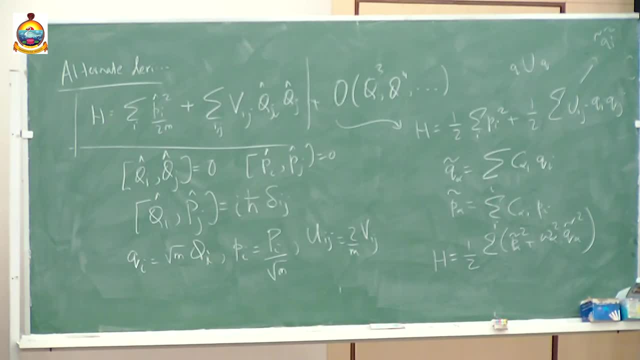 this quantum system is the zero point energy right now. if you have a system in which the interactions between the ground state and the ground state are the same, then you can see that the interaction between the atoms is so weak it's even weaker- zero point energy fluctuation- then that system would not even form a crystal. so an example of that is helium. 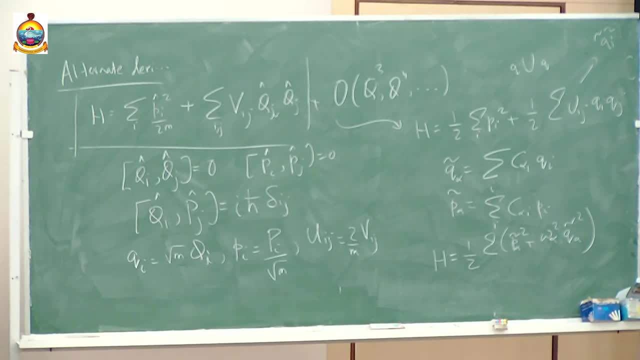 you go to a very low temperature and it won't form a crystal. so that's right. it won't come out classically, because classically you expect it to form a crystal. okay, good, okay. so now i go here and i erase this. i hope everybody has learned something from this: classically. 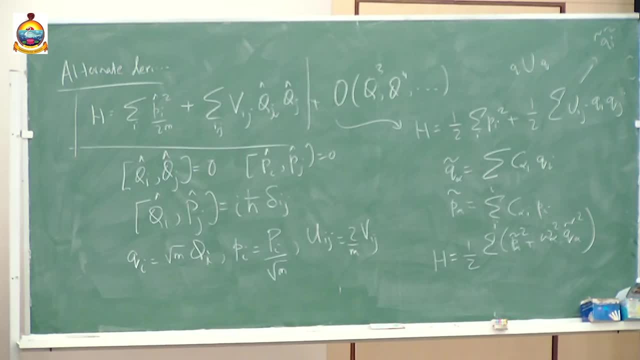 i hope everybody has noted down these exercises. please do them this for your own benefit, not fine, not for my benefit. no, that is of course not known. probably, if you go to extremely small temperature, probably will crystallize, but it's some very small number if. if it's non-zero, yeah, okay. so now, 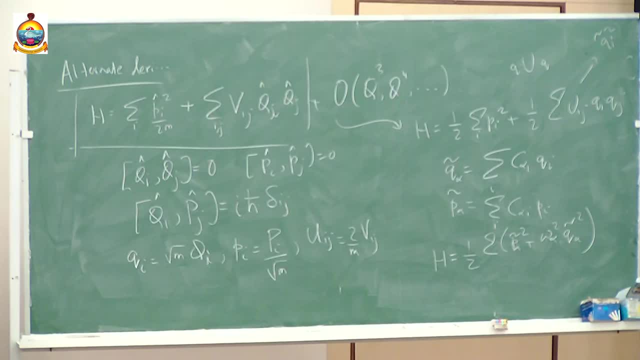 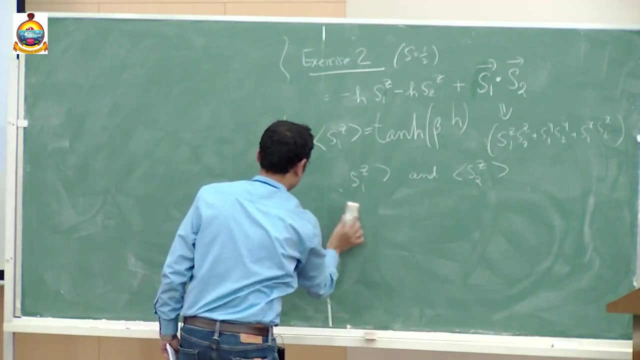 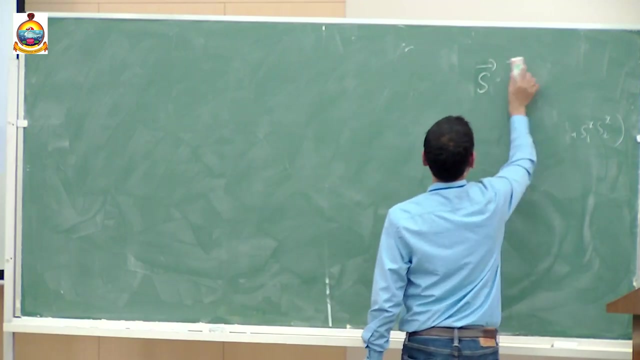 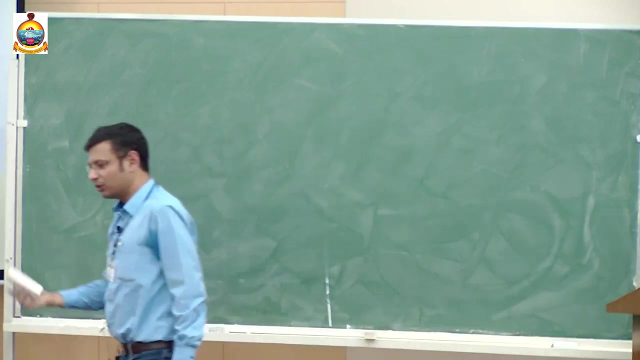 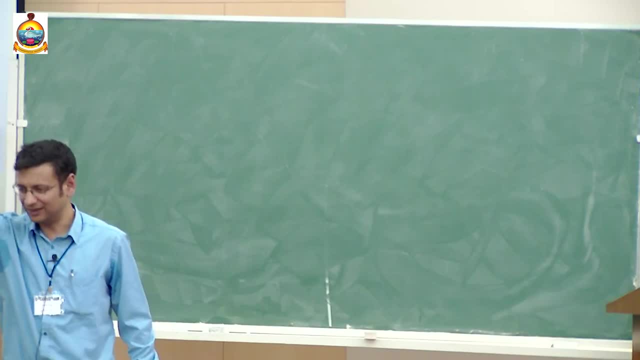 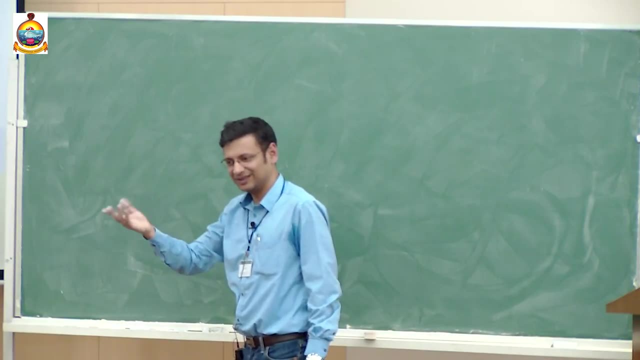 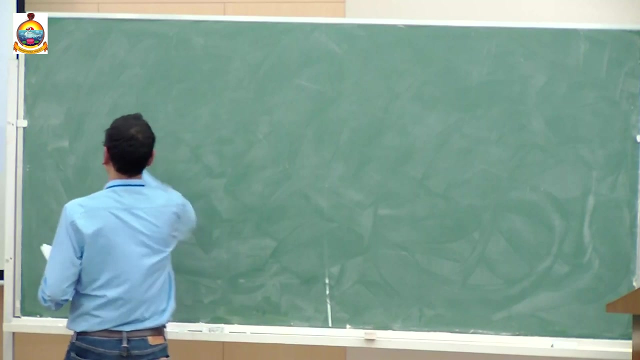 i'll discuss sort of 2d ising models and mean field theory and then in that tutorial section first will discuss these two problems and if you have any other problems, okay and yeah, okay, so now coming back to the specific heat. so now coming back to the specific heat. 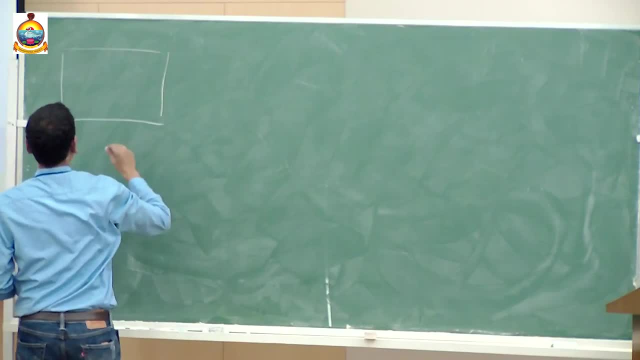 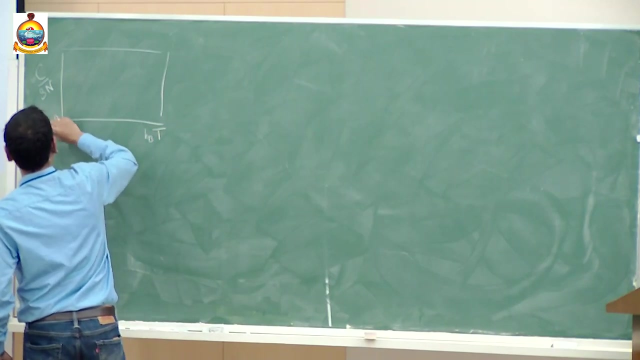 so now coming back to the specific heat: heat. So let us see So now. so basically, this N is the number of. I will let me draw the coordinates here. Let us say k, B, T is 0 and this is also 0 and this is 1.. Why am? 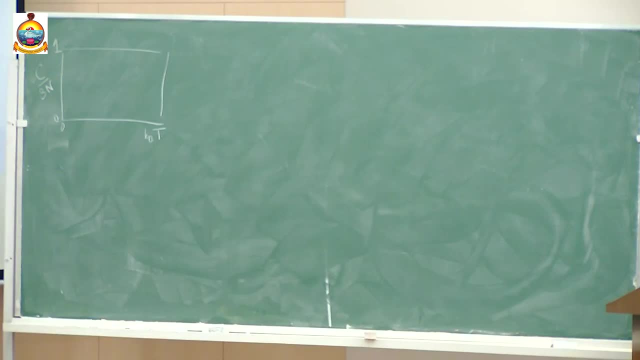 I drawing it like this. So let us say you have a crystal in which there are N unit cells, Then, classically, what do we expect the specific heat to be? Classically, we expect the specific heat to be 3 times N times k B- T, sorry, k B. So let me also divide by k B here, classically. 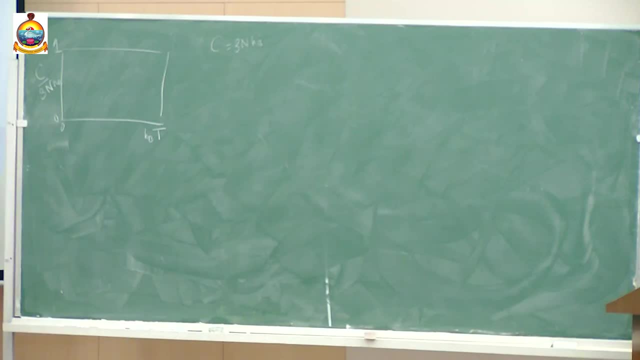 Because you can have, like in a solid, you can have polarizations in any direction, and so that is the factor of 3.. And then the factor of k B comes, because you have a half k B from kinetic energy and half k B from potential energy term, and there is N because these are sort of N unit cells. 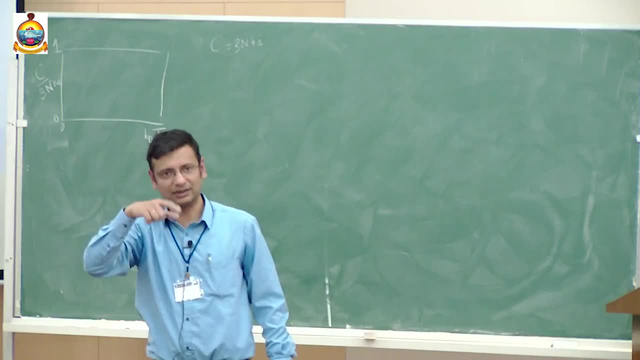 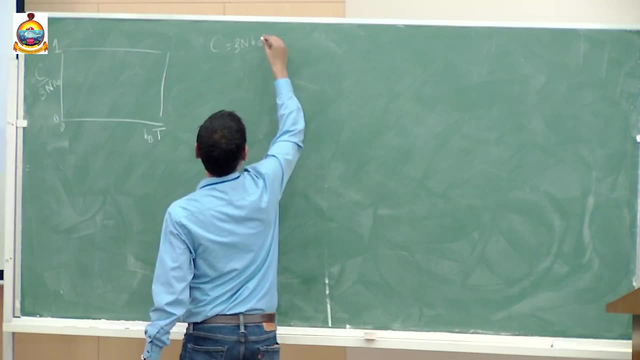 Now you can have a unit cell which has more complicated structure inside. It may have a 2 point basis, 3 point basis, 4 point basis, whatever. Then let us say the. whatever the number of points are in your basis, you also can multiply it here. So if you have a simple 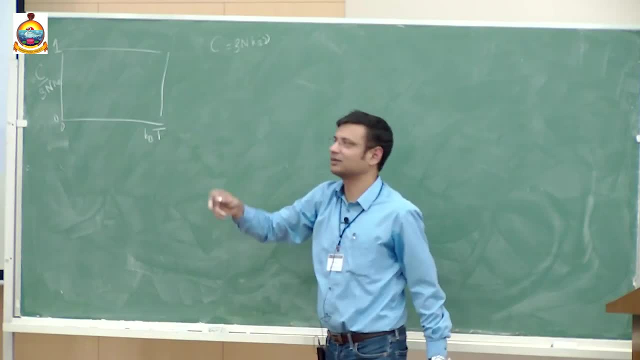 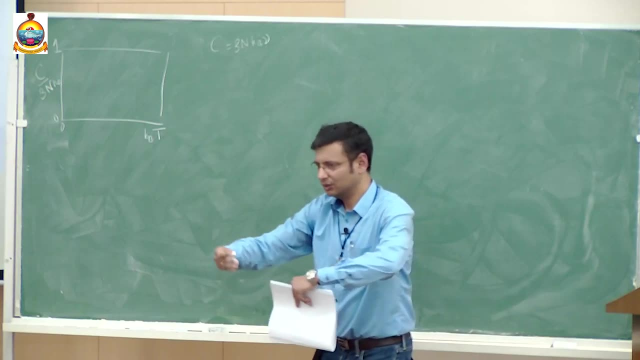 crystal, then this number might be 1.. If you have a more complicated crystal, this number might be 2, so on and so forth. right, This is just the number of entities inside your unit cell to define the Bravais lattice. 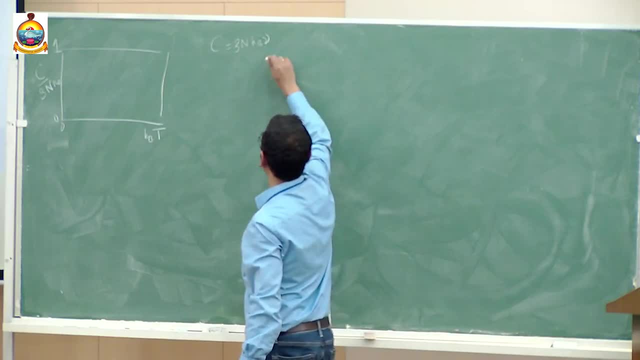 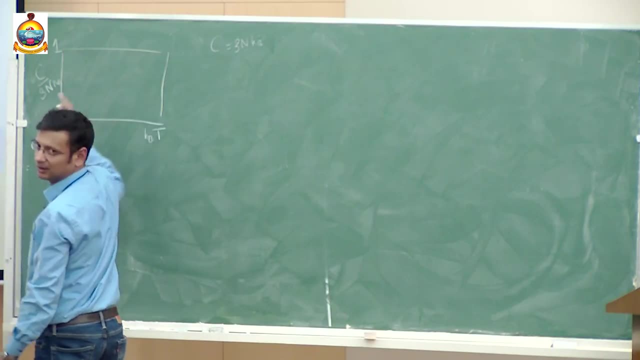 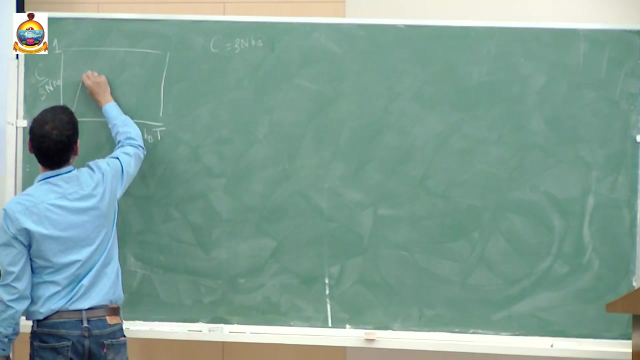 That is it, ok, Good, So this is what you expect classically. So let me just erase this for convenience. now, ok, So then classically, everything should just remain at one right. But what people observed experimentally very soon was, if they did the actual experiments, they saw something like: 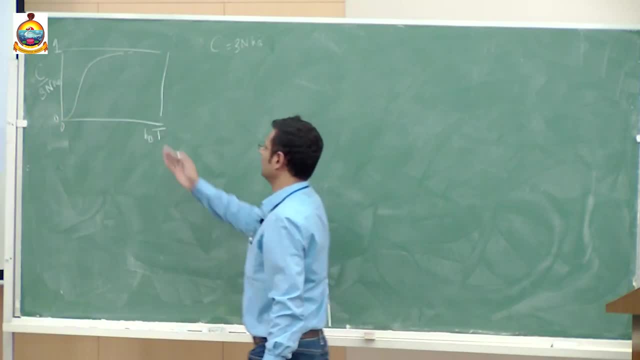 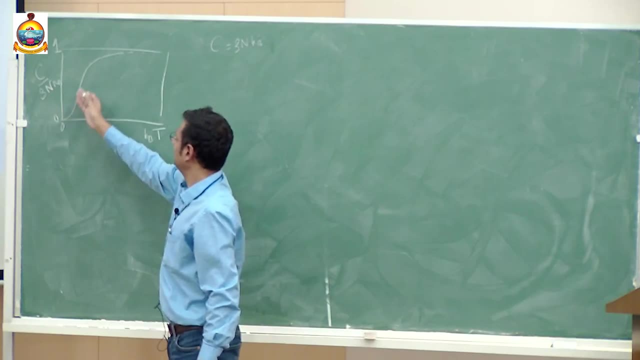 this behavior like this. okay, so, at high temperature, it seemed that it was approaching one where i have divided it by this like this, but at low temperature, it was strongly deviating from this classical result, very strongly deviating from this classical result, and it seemed to be in. 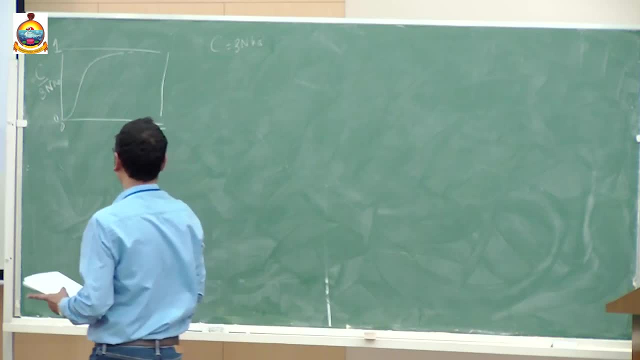 fact approaching zero. okay, so, that was the observation. and then people really tried to understand it. people like einstein, people like drew day, so on and so forth. right, okay, good, so then, uh, let's see what they. oh, i should not have erased anyway. okay, so so let's see what they. 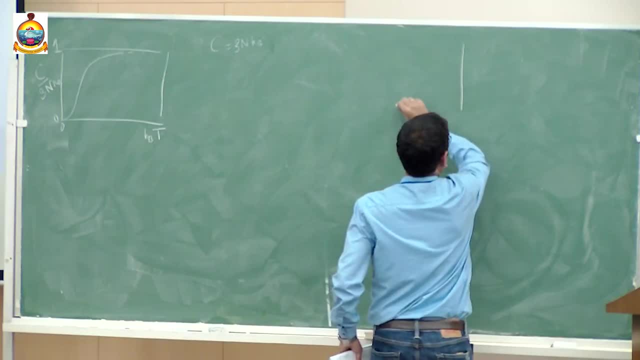 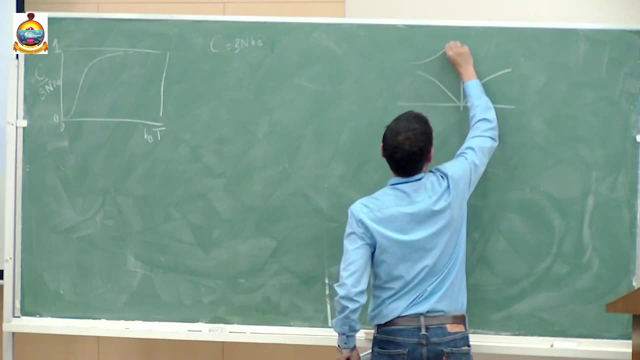 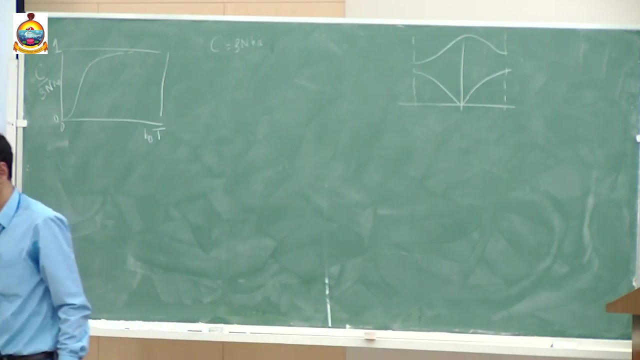 did so. so i said that typically in your system, if you look at the phonon dispersions, you might have things like this. of course it actually looks even more complicated, but you might have things like this. so the first attempt to explain the specific heat of a solid was made by einstein. 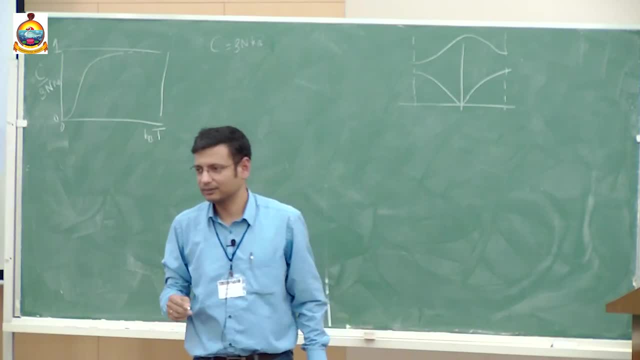 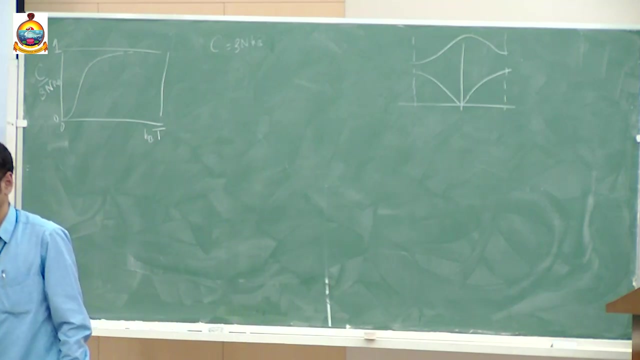 and he, that is true. yeah, that is true. that is exactly true. that's true. no, but if you think of the problem really classically, for a quadratic theory, the specific heat, independent of temperature, is always a kb, right? i mean, you just calculate the partition function and just see it. 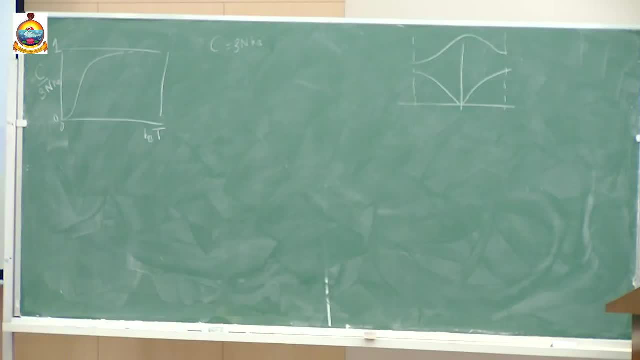 it's always, it's a constant, it's independent of temperature, right? yeah, because even at very small temperatures you can still do lots of fluctuations in. yeah, so you solve it and you'll get it. that's the equi partition theorem, right? so? so there is some crucial thing missing, and of course, now we 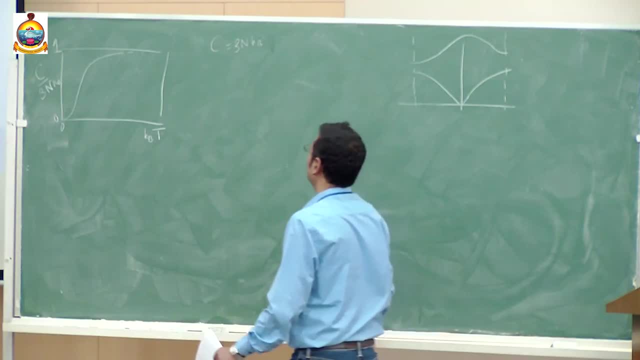 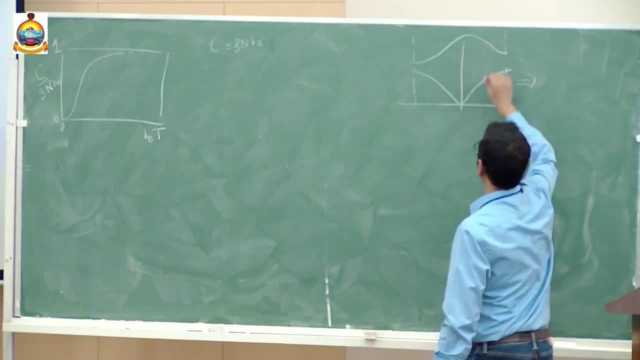 know what it is, but at that time people didn't know it. so right, okay. so yeah, i think i'm really impressed here with the theory of the equilibrium, because it is kind of interesting that i want to. okay, so what einstein did was: i mean, he started with a model which is an approximation of 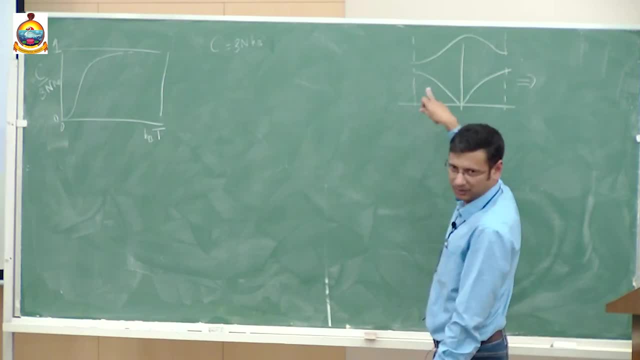 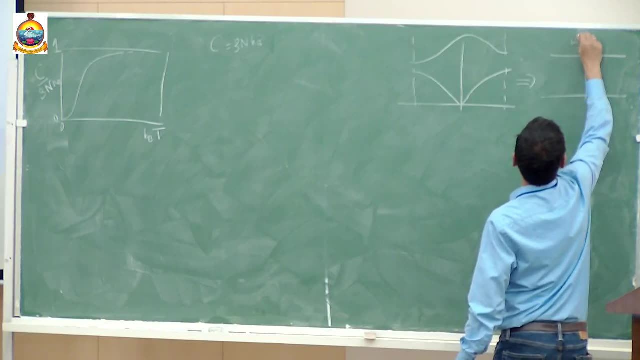 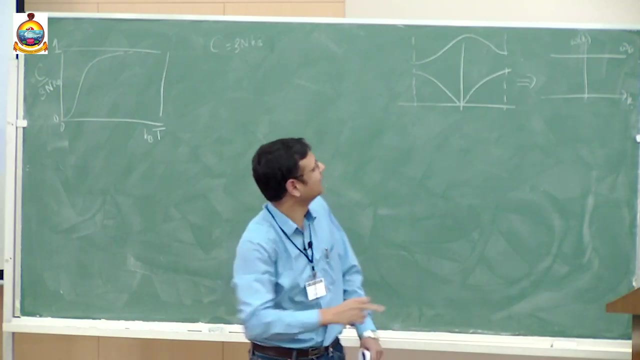 this complicated thing. of course, in a real life situation, you saw that it is even more complicated, right? so einstein started with the following model, where he said that this is my dispersion, literally, so everything is at omega. e e is for einstein. he did not call. 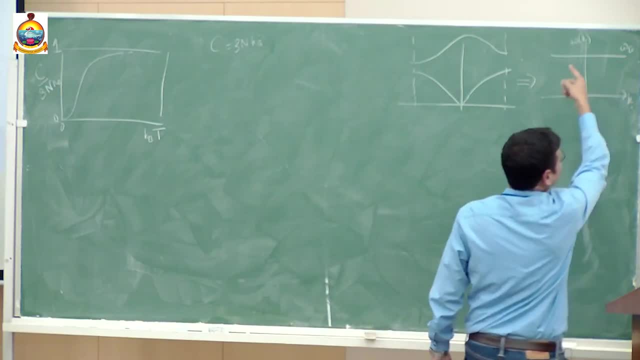 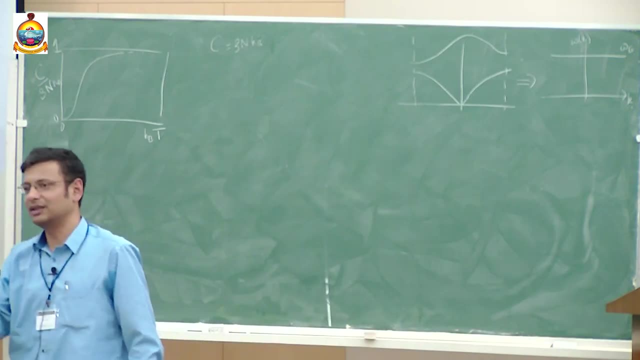 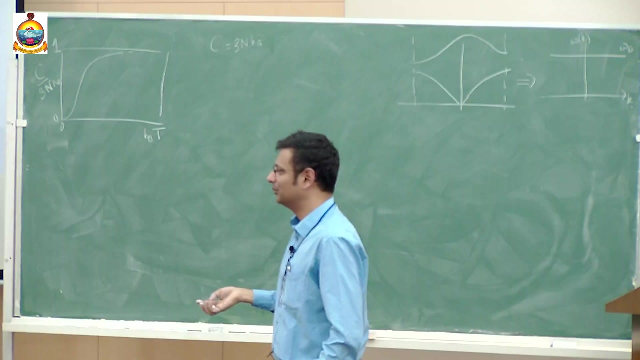 it that, but let me use this nomenclature. so basically, he just said that this is my spectrum, that's. it just said that. so basically there are n modes in my crystal and all the modes are oscillating with the same frequency, omega e. now, this is a very simple problem to calculate. 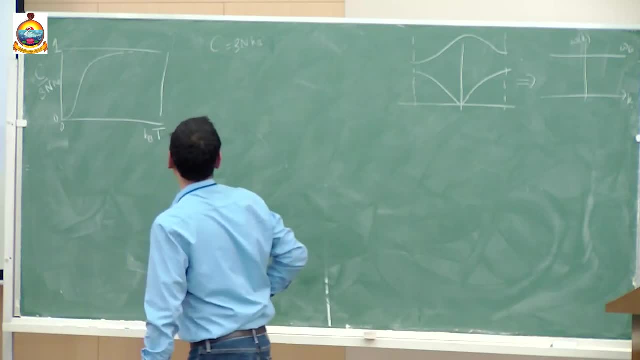 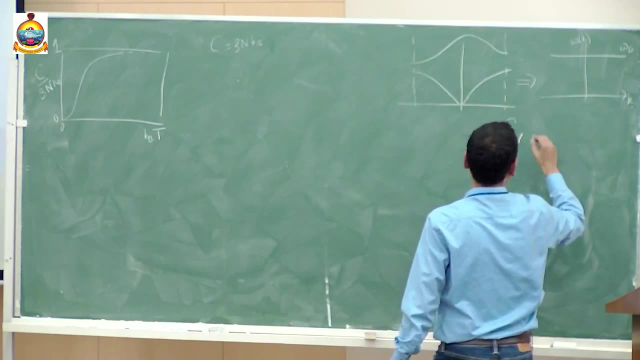 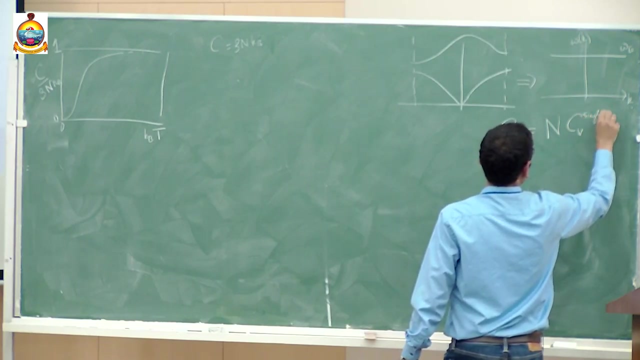 so probably in your notes somewhere you have the answer written for a single harmonic oscillator, right? so the answer for the specific heat here for multiple harmonic oscillators is just n times answer for single oscillator, at that omega E. So this is the property of that oscillator. 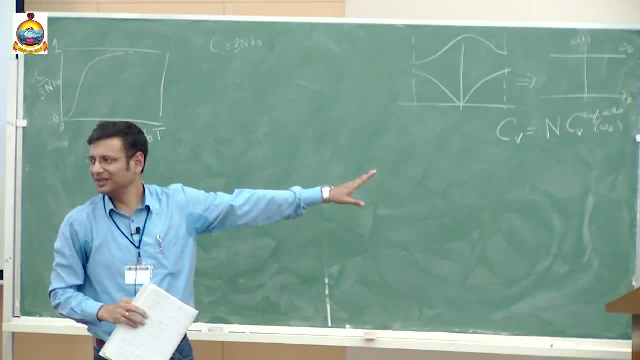 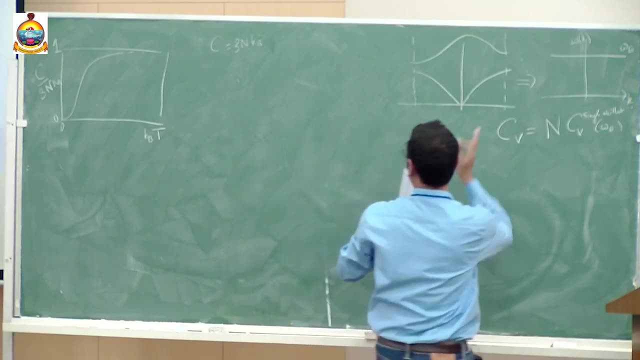 right? Is this clear to everybody? I hope I do not need to do any calculation. So there are these n oscillators here, all of them, or may be there are factors of three and all because they have three directions possible. but that is ok, I mean. so you see the important. 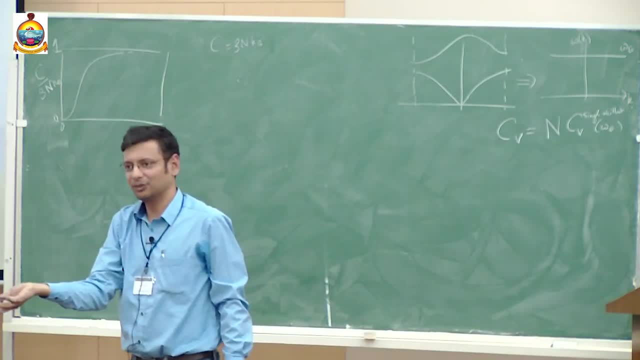 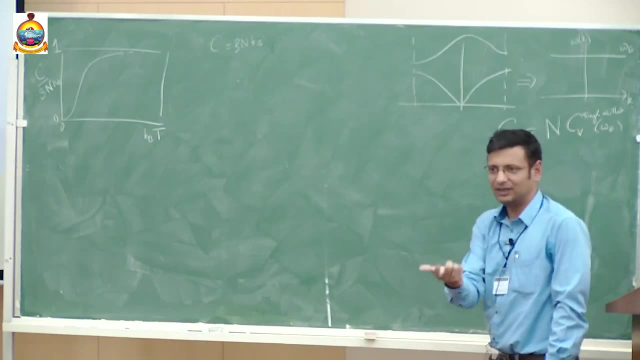 thing is that there are these oscillators here, all of them are oscillating at omega E, So, and they are not interacting with each other. So, of course, what is the total specific heat? Just n times the specific heat of each individual oscillator, and we already know. 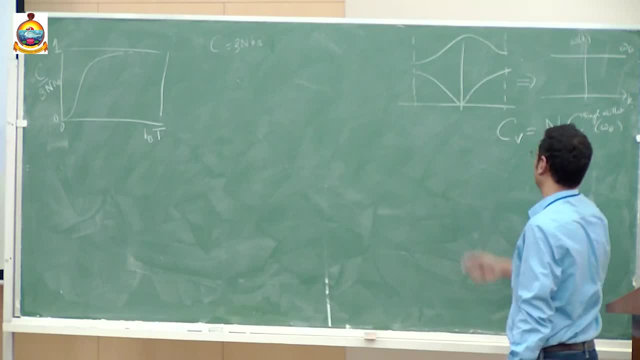 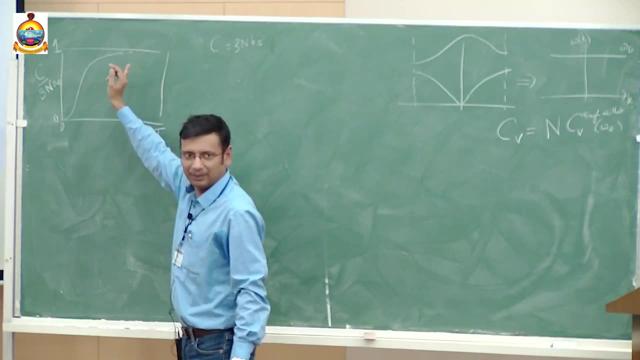 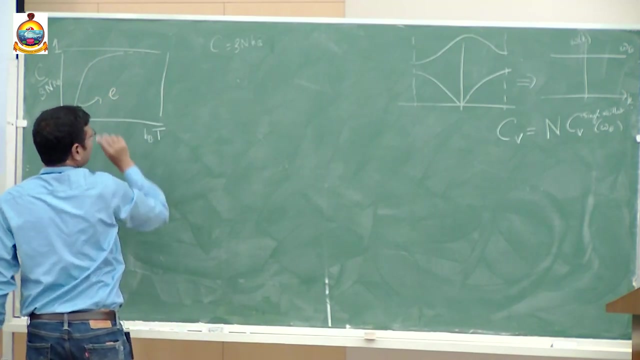 the functional form of this. I wrote it down there and I erased it. but yeah, So see, that thing, as you remember from last class correctly went to the classical limit when temperature was high. right, good, So this part is correct. but that thing, how did it go to low temperature? 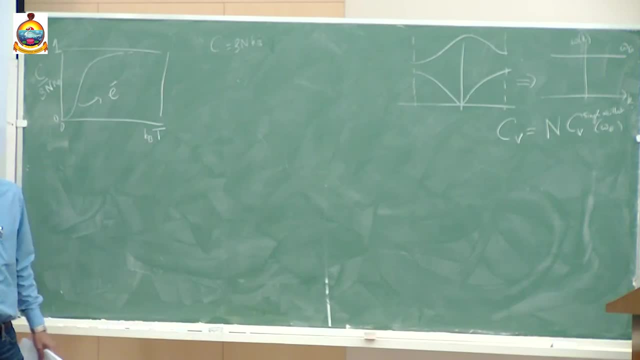 What is your guess? How does it go to low temperature? It is going exponentially, So how should it go at low temperature? What should I write here in the exponent? So the oscillators are oscillating at omega E. There is only one possibility. 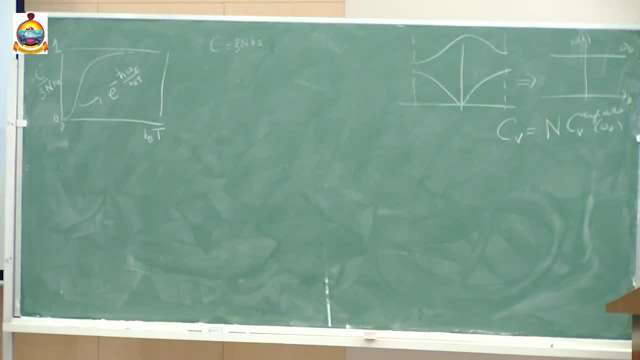 This is how it goes right. this is how it goes, And in fact we know experimentally. so it is at least going to 0.. That looks nice, but experimentally it was soon realized that this was too steep a decrease. it does not go like that. So then we were again back. 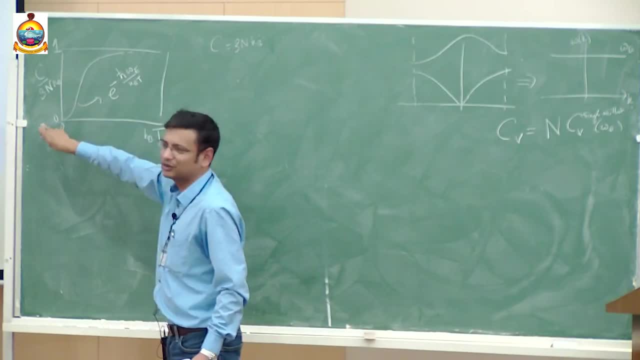 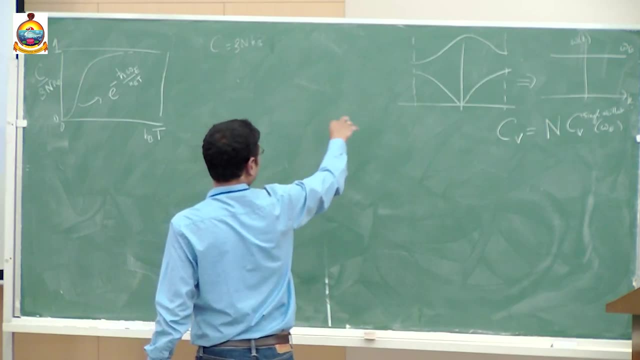 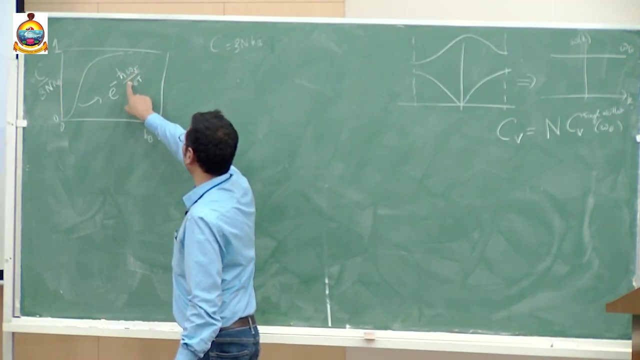 to square one. at least Einstein's theory explained that something is going to 0, but it is not going to 0 correctly. So then we needed some other kind of approximation which correctly captures the physics. So just when I was writing h cross, omega, E by k, B, T, I realized 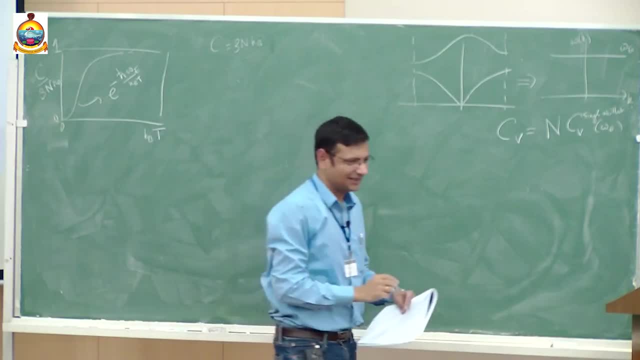 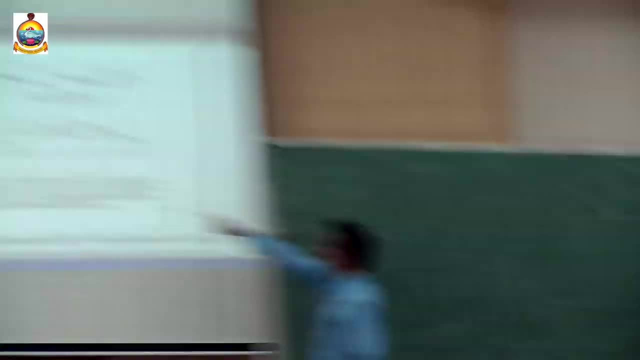 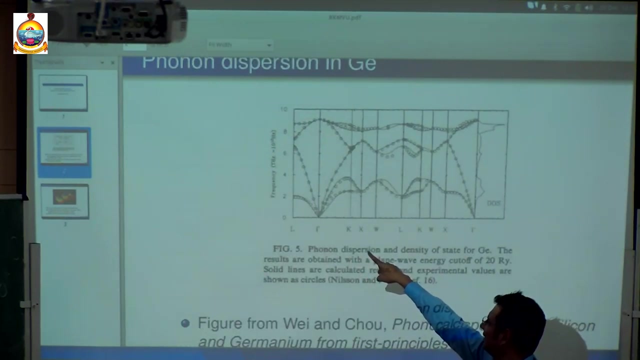 I realized something which I did not point out to you, So let me go to that experimental graph again. Let me just go there. So do people notice what is the y scale here, Terahertz? So does it tell you anything about the bandwidth of this problem in terms of temperature? So, 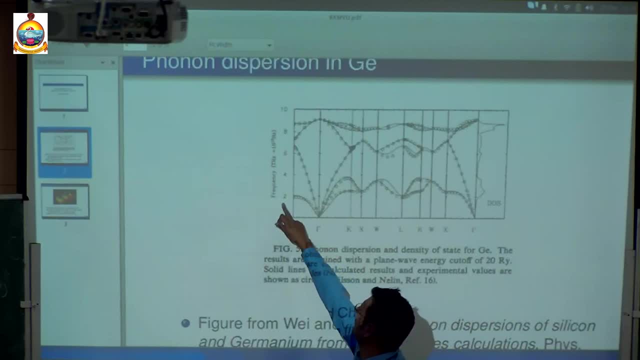 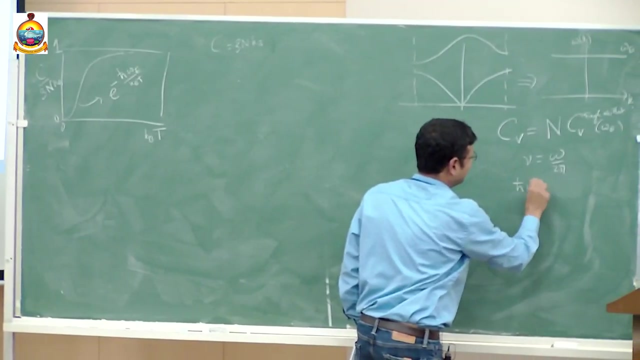 let me rephrase it. See, there is a frequency here, and this is the order of that frequency. Now you can take any frequency, and from that frequency you can get the correct omega, and from that omega you can get an energy unit, and then you can convert it into a temperature unit. 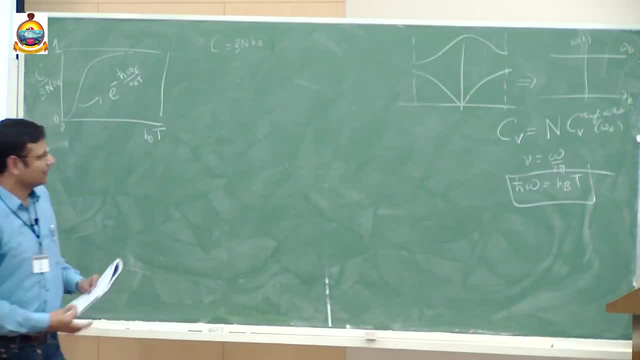 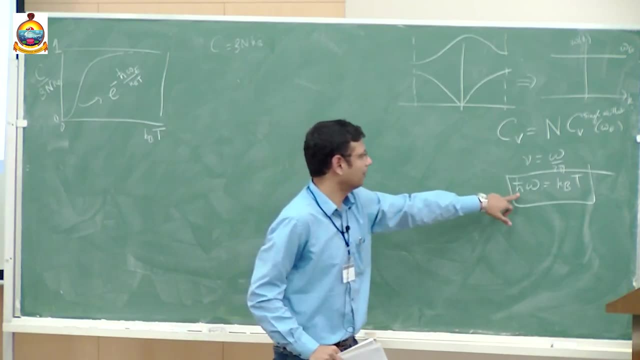 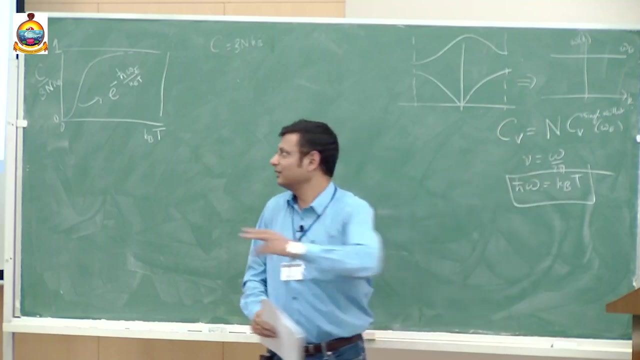 like this. So now, if you have something like a terahertz there, whatever the numbers are here, if you do this calculation yourself, you know all the information here, right? If you do this calculation yourself, or let us say, one terahertz, and then you just see. 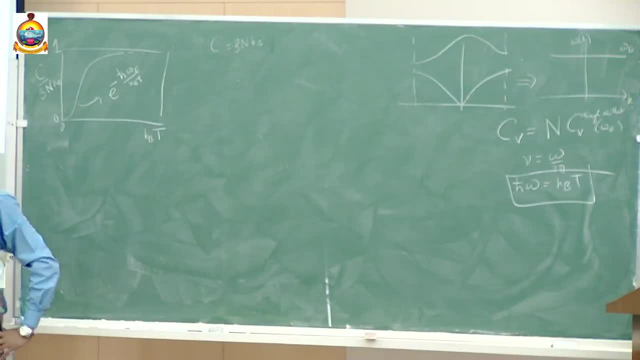 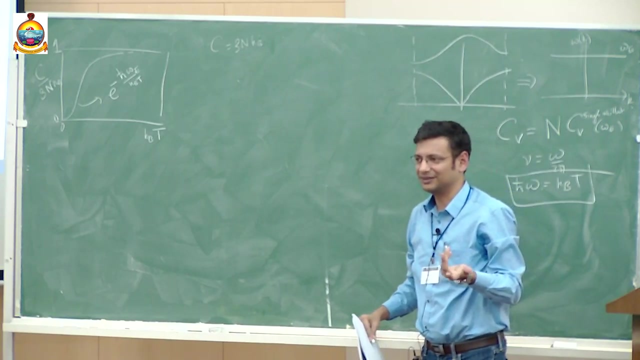 these numbers. Typically, these numbers would turn out to be of the order of 100 to a 1000 Kelvin, So that is a very useful calculation. to do So immediately. just by looking at the experimental data, you know that this width is roughly of the order of 100 to 1000 Kelvin. 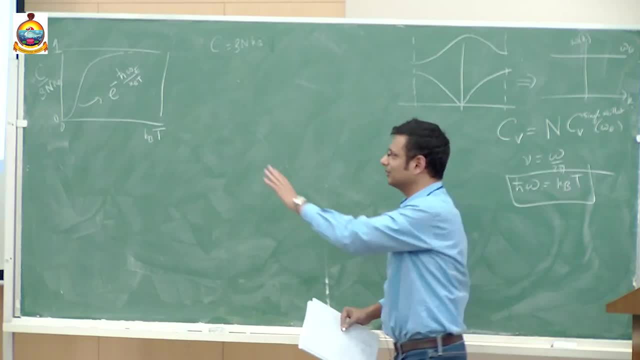 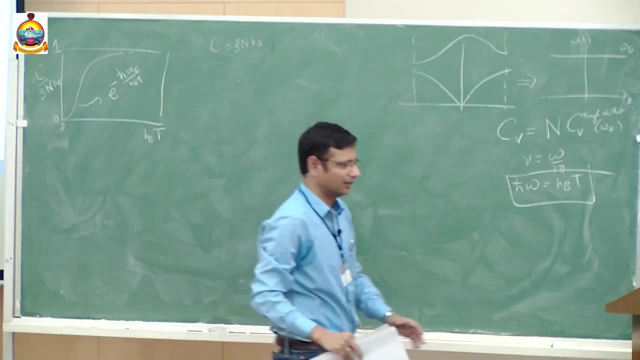 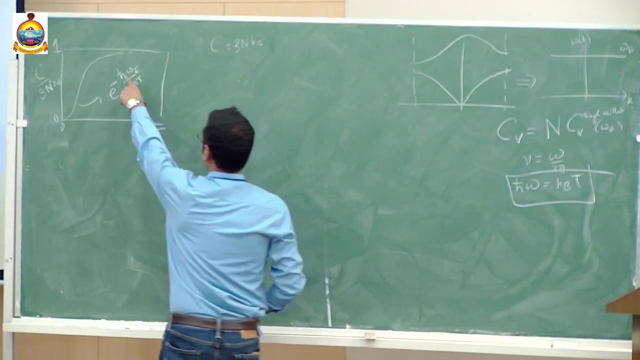 right, any microscopic theory, right. so these kinds of things you should appreciate when you see these kinds of peculiar numbers. okay, good, so that is all that i wanted to show. restress again, because when i was writing this i just realized this, because of course, you can convert. 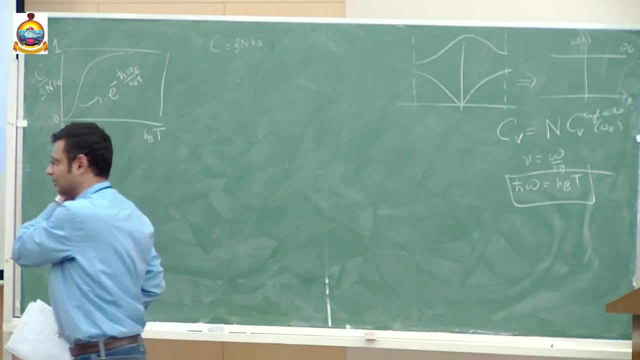 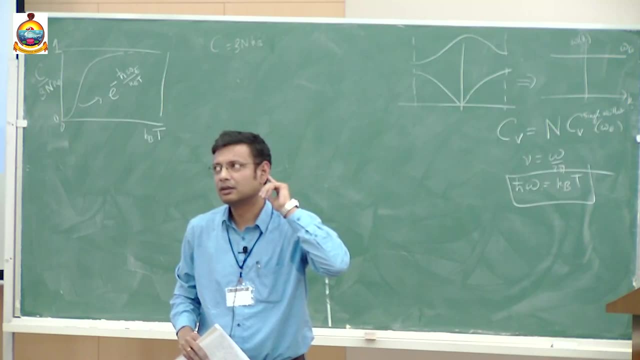 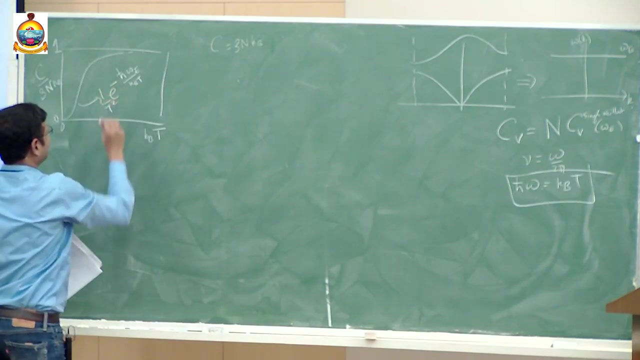 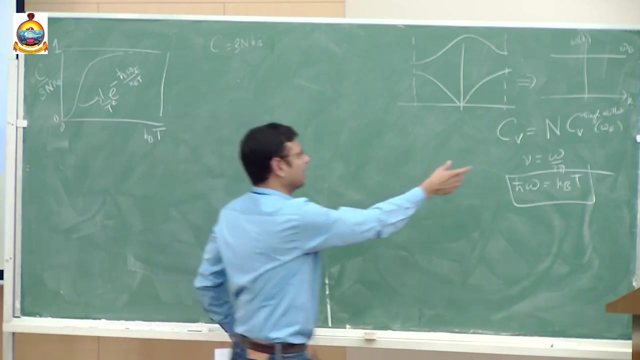 it into, uh, temperature units, right, okay, good, where with c? oh, here, of course, of course you're absolutely correct. that is there. but you see, this is an exponential factor. this is the dominant piece. no, no, of course, yeah, yeah, so yeah, whatever is your answer here, you just multiply by n and in einstein theory you'll just get that. yeah, but 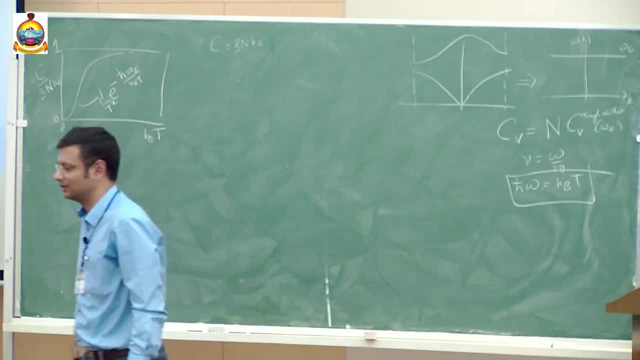 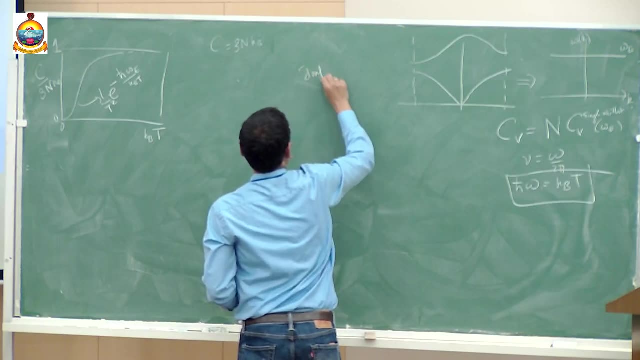 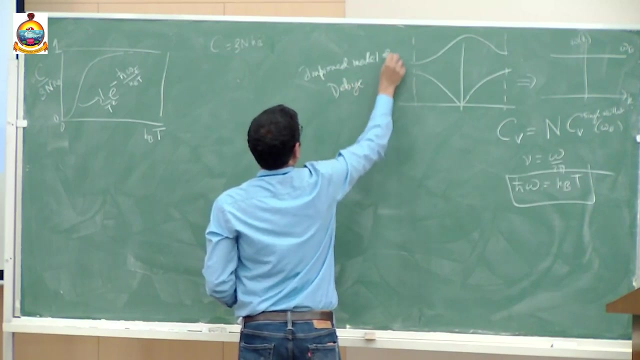 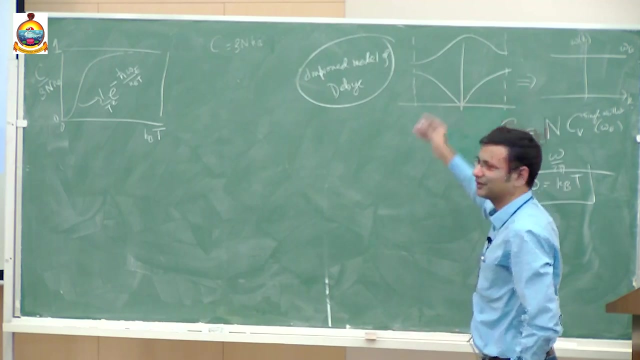 the dominant piece is still exponential. you're correct, there's a one by t square. yes, okay, so now we move to the improved model of dubai. see, can somebody tell me why einstein did not get the right specific heat at low temperature? answer is very clear from here. 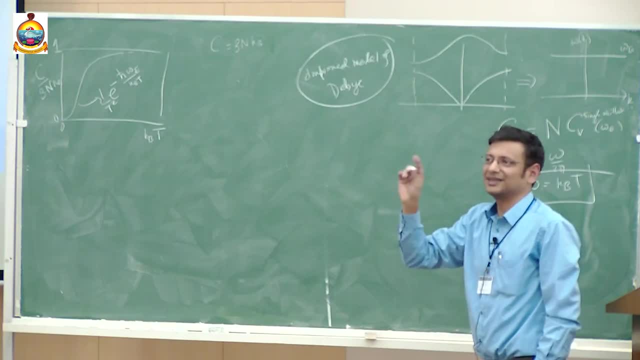 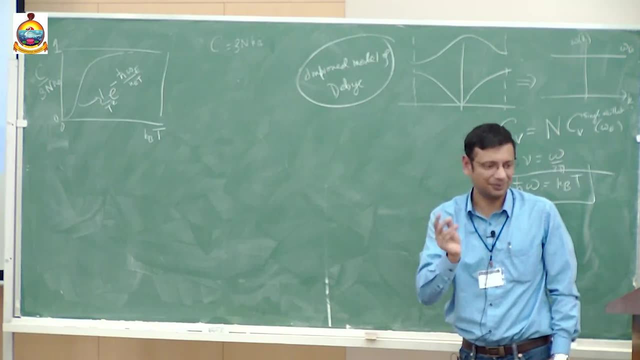 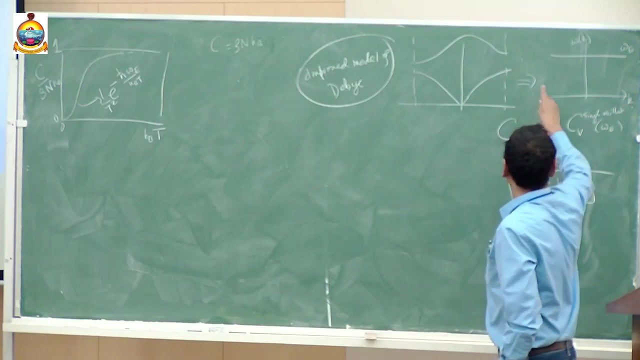 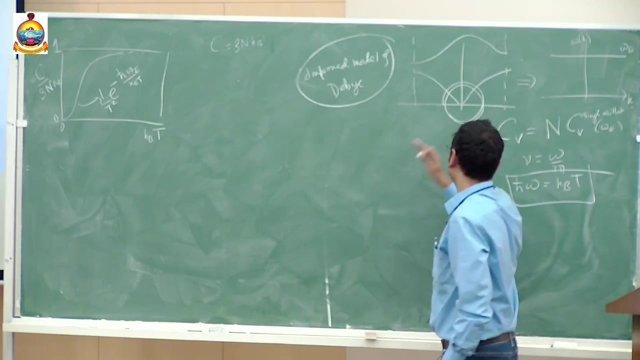 no, no, that's correct. all frequencies are same, but they're not the same. yes, correct. so einstein missed all this weight. this is the thing that significantly contributes to specific heat, right? so einstein, in his approximation, missed that, but dubai did not miss it. in fact, approximation was built on this and therefore he can. 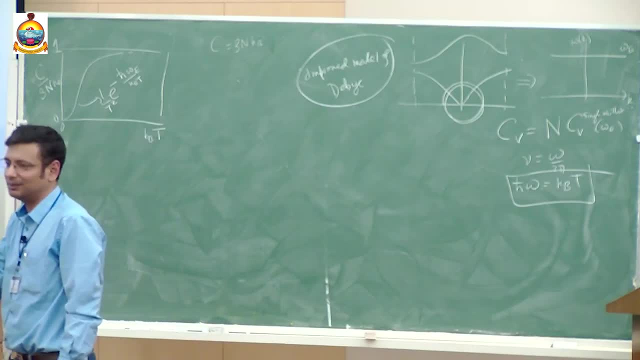 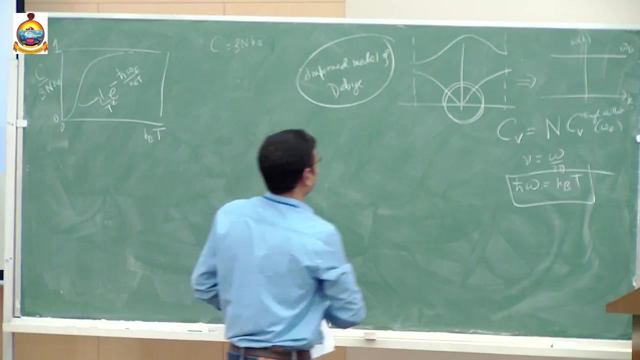 got the correct T cube. Of course, the prefactor that Debye got you should not literally take it, because he used some model and the prefactor is specific to that model. But the fact that he got a T cube is independent of that model because, as I said, at low temperature your 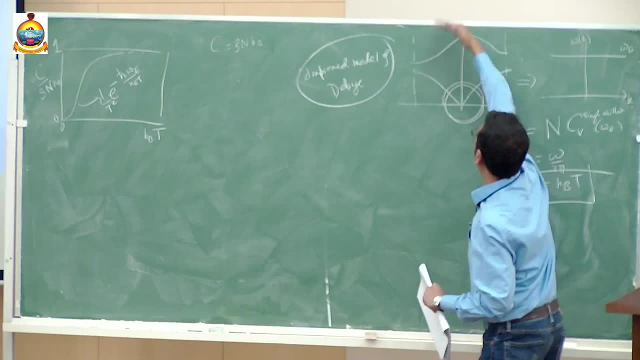 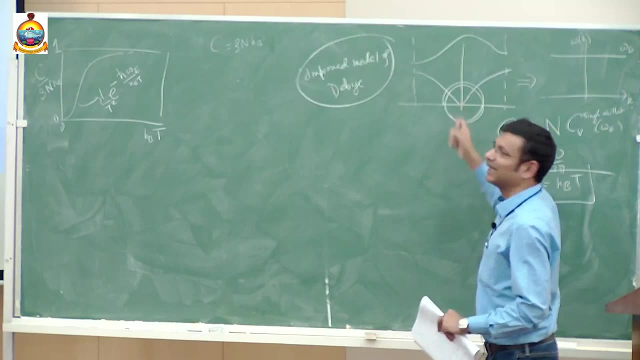 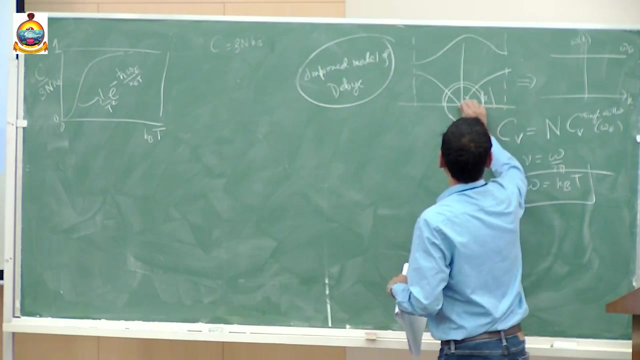 system just cares about this part. It does not care about all this thing sitting here and Debye's model had the one essential feature correct, that this is gapness. and the second important thing is that this is linear. omega is linear in K. So any theory in which you 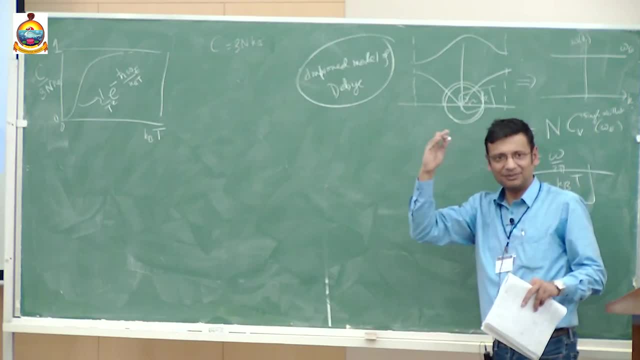 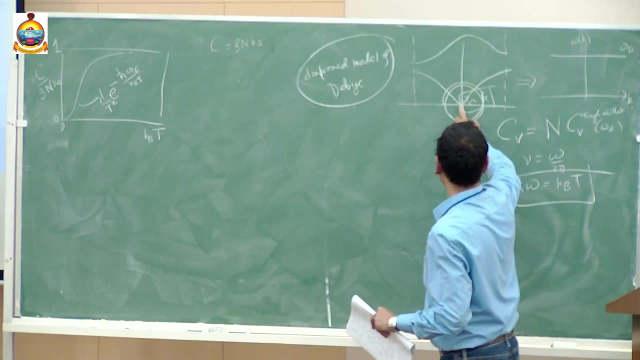 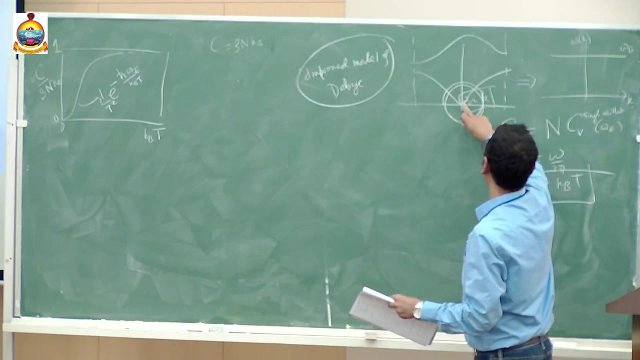 incorporate. this would give you the correct low temperature. That is it. Please remember this. This is an important thing: Any construction you make which has gapness and has the right word for dispersion, Right, right dispersion. i mean if you started with the dispersion which went as k square for 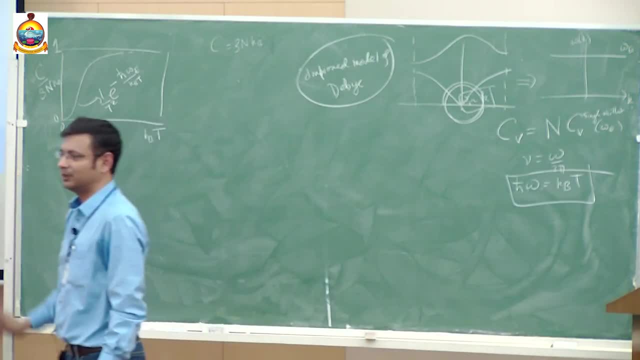 example, free particle dispersion, then you would not get the t cube correctly. then you will get some other power. in fact, if i am not mistaken, you will get t to the three by two. okay, so so that's important. so these two things are important. good, so what did debay? 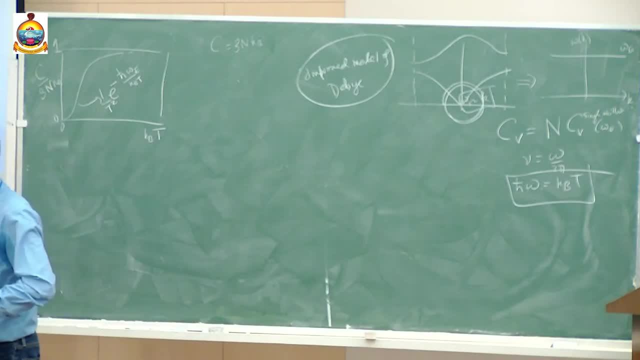 do? debay said: okay, i don't know about the very complicated things about the crystal. of course debay knew it, i am just putting it like that. i mean. so he said i don't want to care about the very complicated details about the crystal. let's say we are just looking. 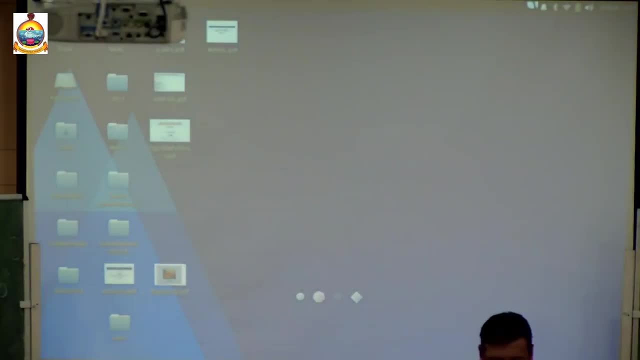 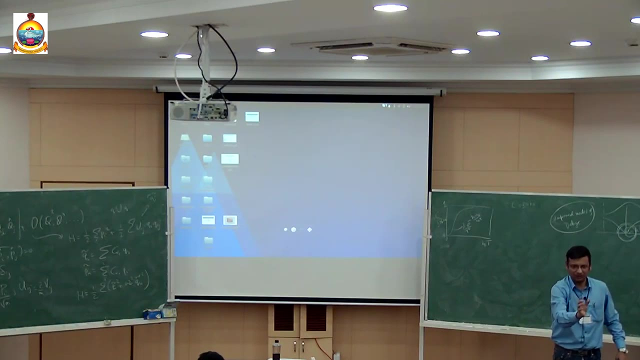 at long wavelength modes in a crystal right, then whatever is the structure of the crystal is not so important, right? because you are looking at the thing at a very long wavelength, right? so the fine details of the crystal are more or less unimportant. then you can replace. 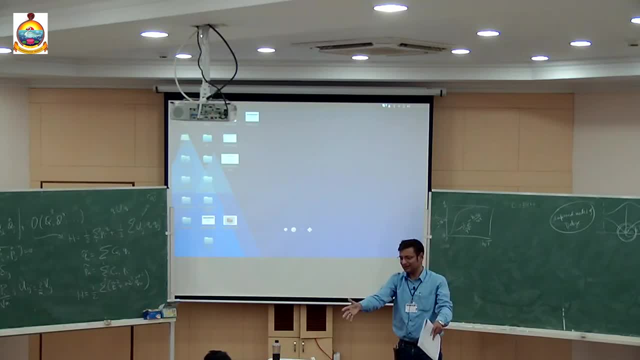 the crystal with the fine details of the crystal, and then you can replace the crystal with just an isotropic solid. and we know that in an isotropic solid you get sound modes right and the sound modes have the property that omega is linear in k. that's the property. 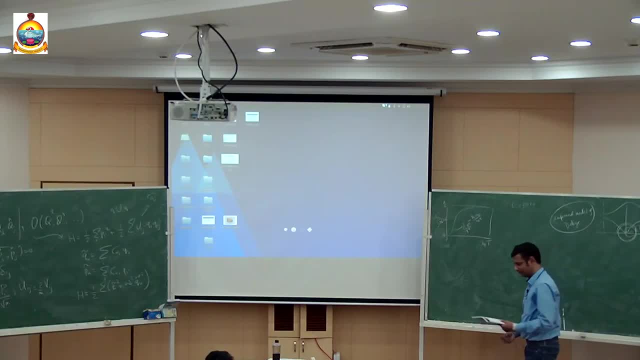 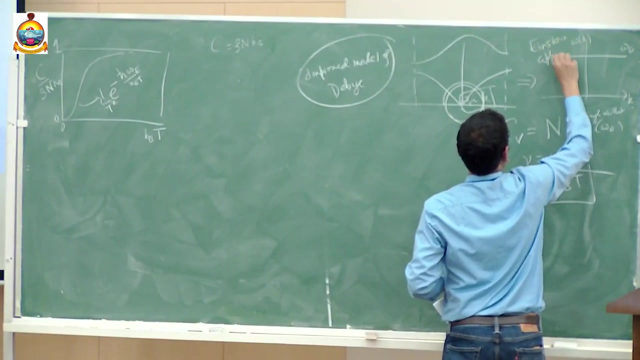 of sound waves. okay, so that's exactly what debay used. okay, good, so debay said that you have an isotropic solid, so debay's approximation is the following: so see, there are series of approximations here. this is einstein's approximation. this is einstein's approximation. the real thing may be very complicated, maybe there. 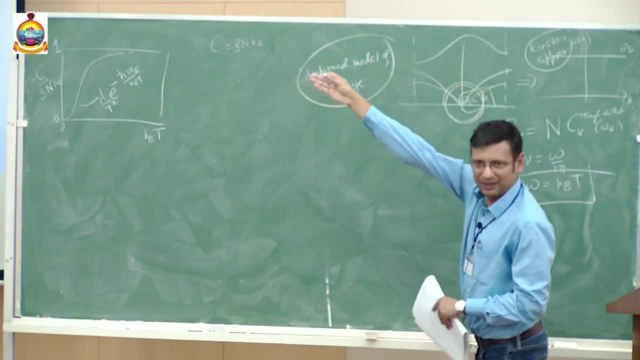 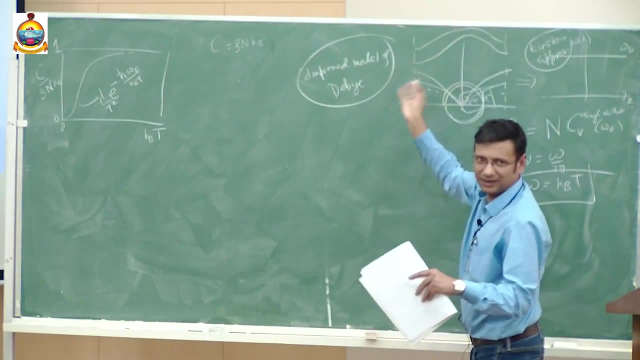 are even like more than one branch. who knows? actually in the picture we saw there were more than one branches, right, so maybe there are multiple branches here, right, and something's here also, whatever right, this is very complicated. so einstein's approximation was this: debay's. 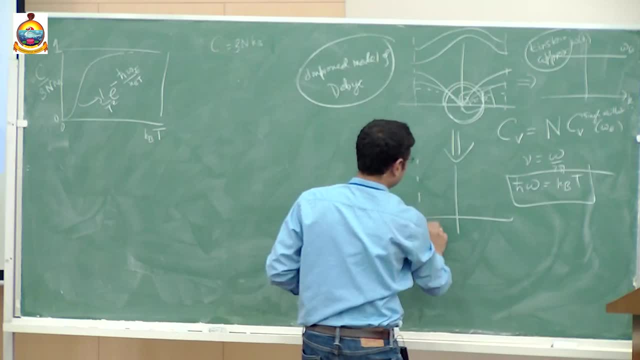 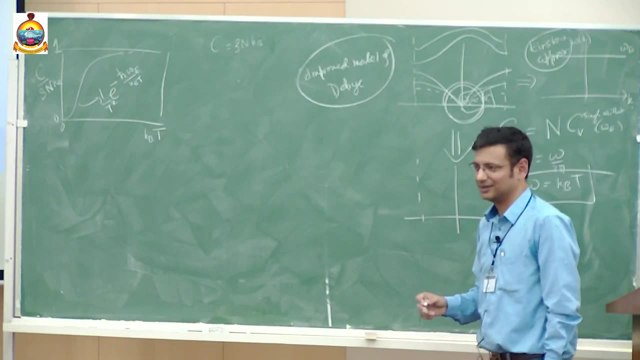 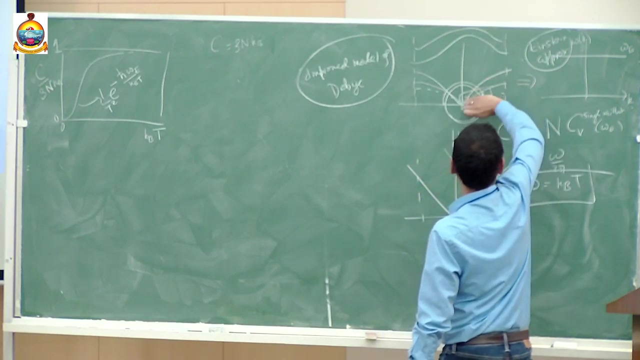 approximation was: can somebody guess, what should i draw here? what should i draw here? what is debay's approximation? i already told you the answer: right. so debay's approximation is: what is the answer? what? correct, linear, absolutely linear. see no curvature even near the zone boundaries. absolutely linear. right, because debay said: let's just replace it by 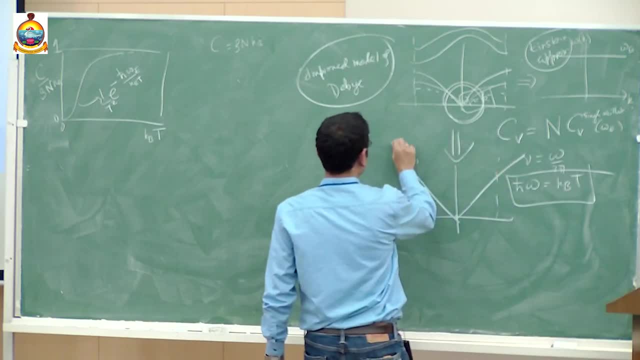 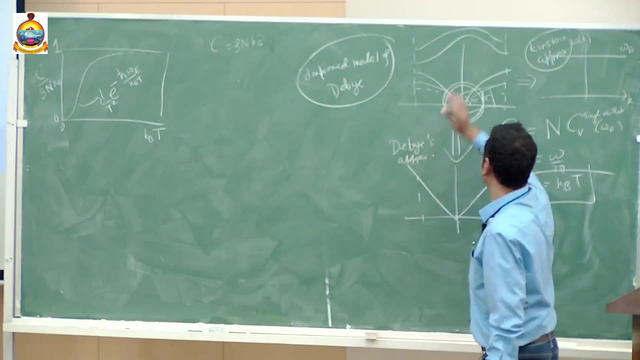 a completely isotropic medium, so absolutely linear. so this was debay's approximation. of course, the key thing to stress is: both of these are approximations, but this would give you some physics, correctly, qualitatively. but if you want to absolutely match numbers, i mean this may fail because, as i have illustrated this, 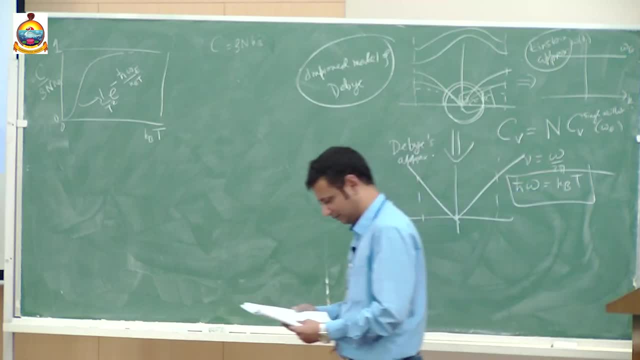 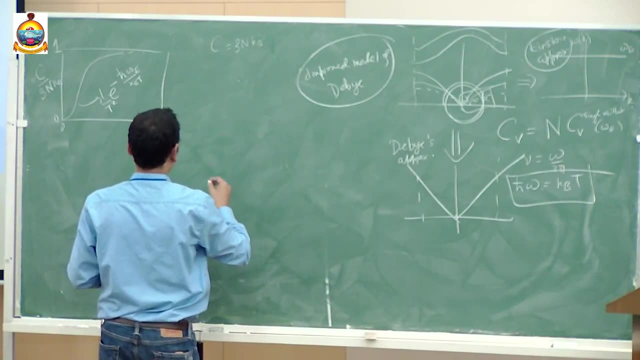 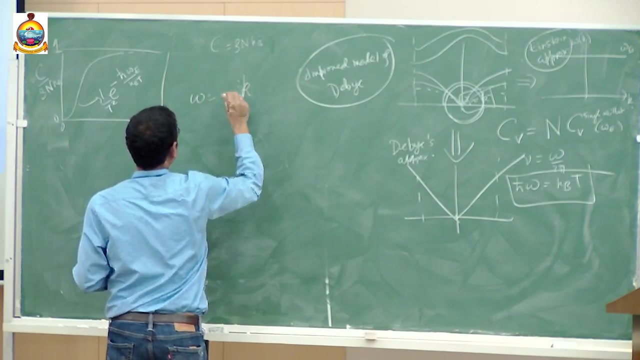 is an approximation, and this is an approximation, okay, good, okay, we are doing sort of okay, right, okay. so now i said that omega is, let's say, some v times k, or actually c times k. so c is the velocity of sound, not the speed of light. okay, 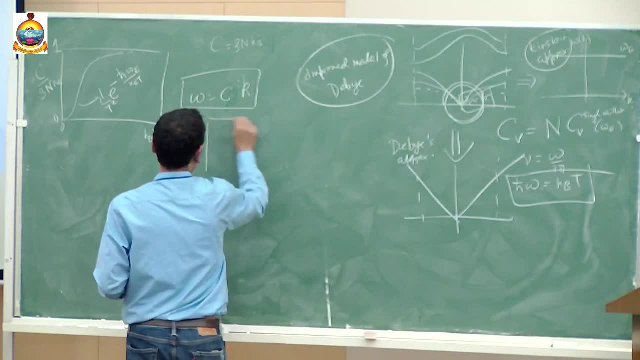 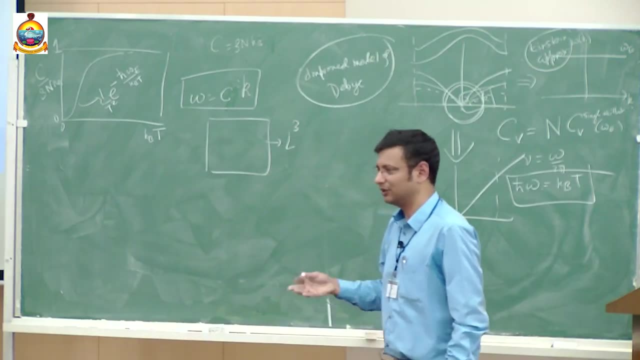 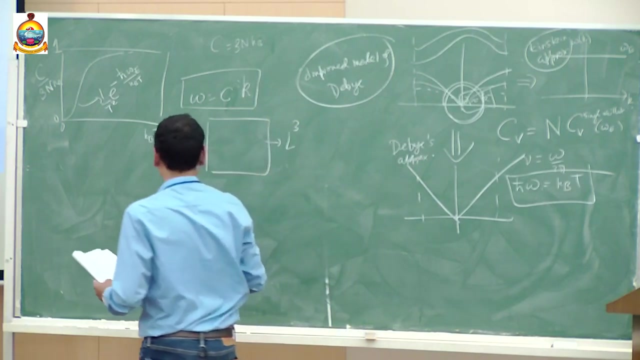 good. so now again we do our standard thing. we have a cube of length, l cube, so the linear dimension in each side is l, and then we take periodic boundary conditions. that gives us a discrete bunch of momenta because of the boundary conditions. and right, we then can. 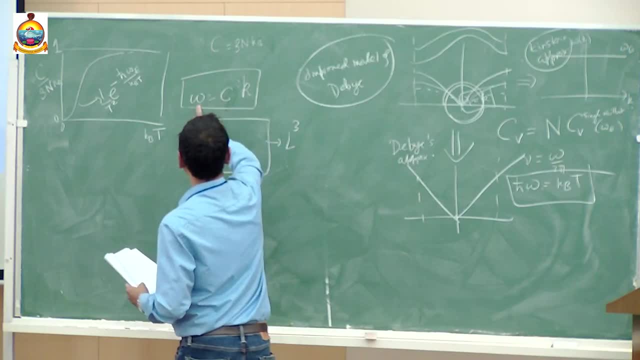 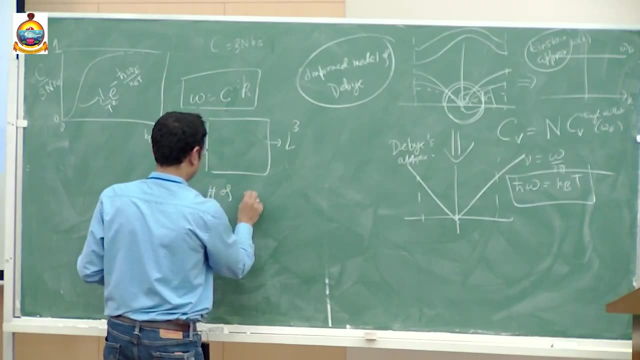 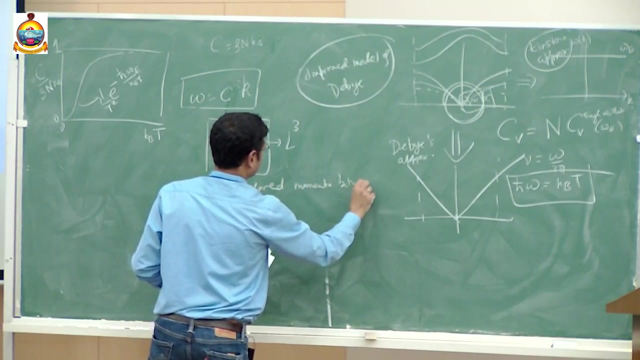 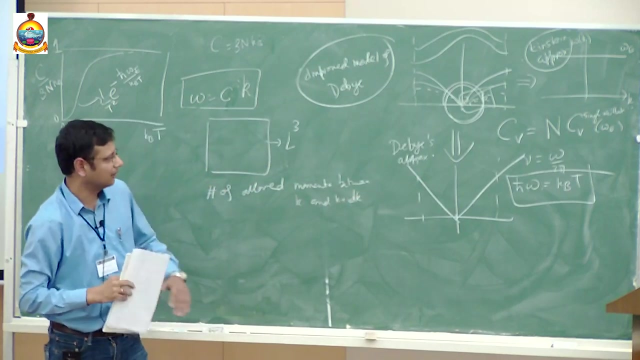 convert from k space to omega space just by using this relation, so on and so forth, right? so let's do those simple things. so, number of a allowed momenta between: see, now the problem becomes very simple, right? i hope you can realize that even before we start our calculation. so debay's say: this is my curve, so i know. 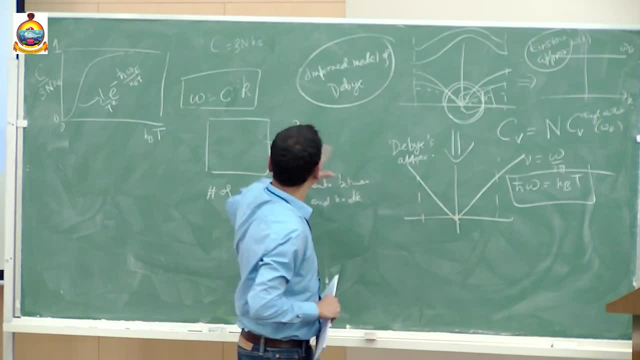 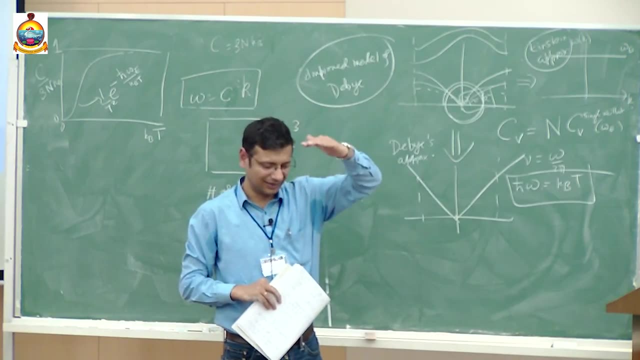 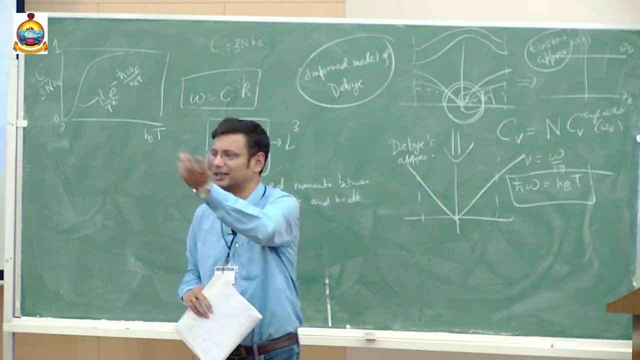 that at each. i know that, given a k, this is my omega right. i know this. and these are independent harmonic oscillators, so i know that, i know its even and so on and so forth. right, so, outside, know what is the average energy for each harmonic oscillator at a temperature T? I will just 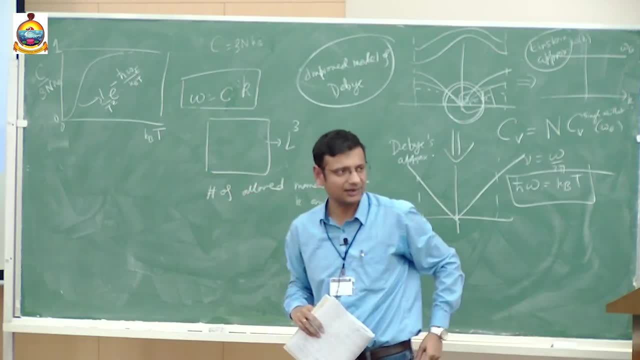 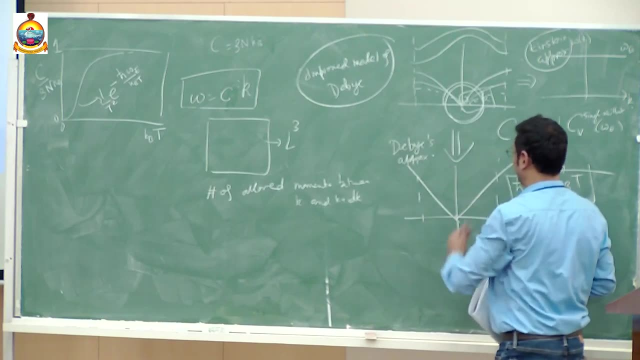 add them up. That is it. And then I will differentiate that answer with temperature and I will get specific heat. So what is the only thing that I need to calculate a bit carefully? See, when I just give you this spectrum, remember I told you that there is this notion of a. 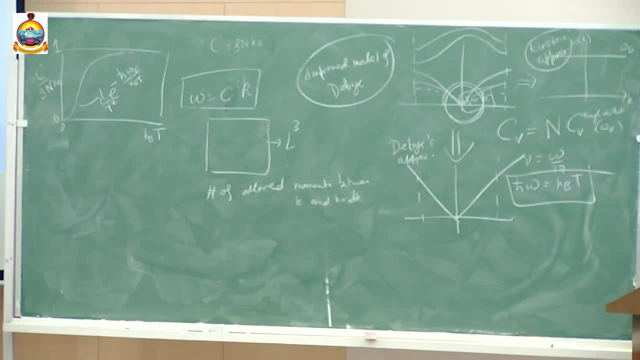 Brillouin zone here. So one way of thinking about the Brillouin zone is that effectively there are only n modes here, capital N modes here, and that is what the Brillouin zone was restricting here. But this was based on a microscopic calculation, So I was sure that 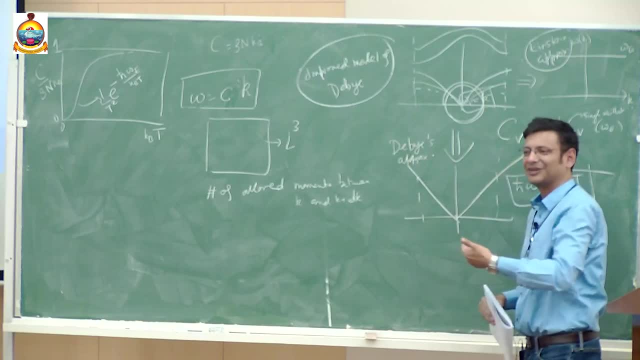 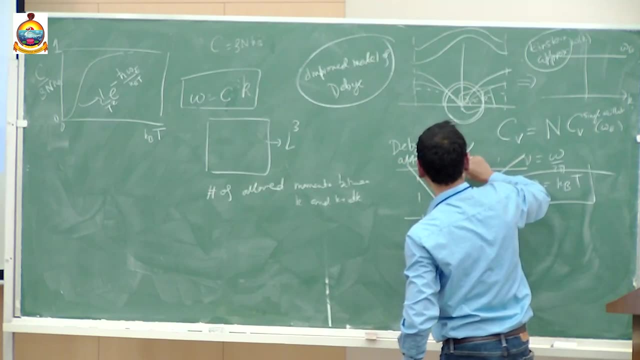 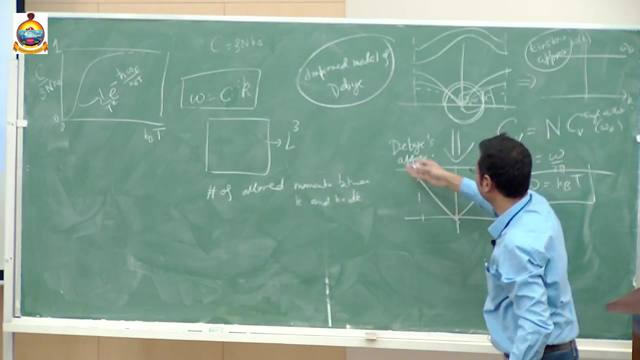 there are n modes here, But now I am replacing it with some approximate model. Now I have to tell you what is an omega max here. I hope you realize what I am trying to do. I have to tell you what is an omega max here. I cannot let this curve run ad infinitum, because then 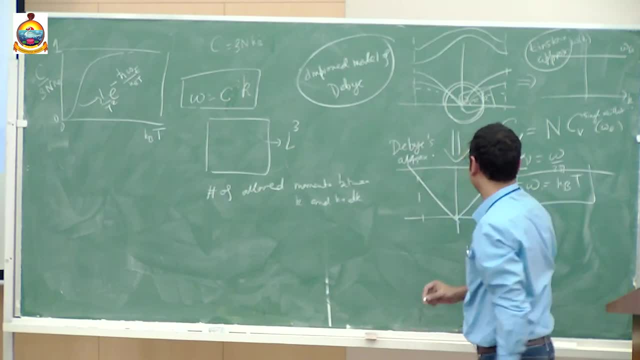 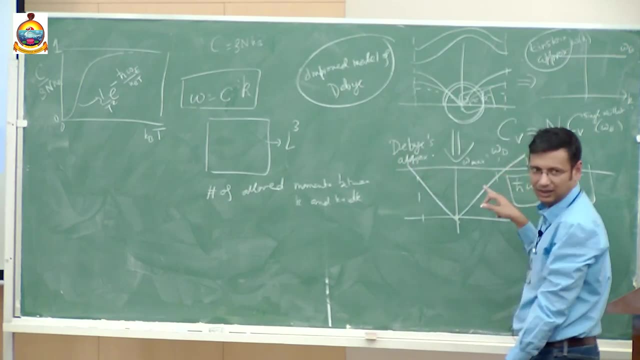 there is an infinite number. That is impossible. I should have n modes So I have to sort of place a cut off. omega max- This is actually traditionally called omega Debye, So omega sub d, And basically the property of this omega sub d is: if I count the number of modes inside, then I will get. 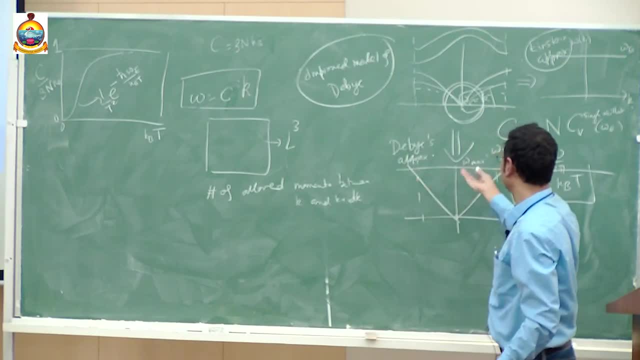 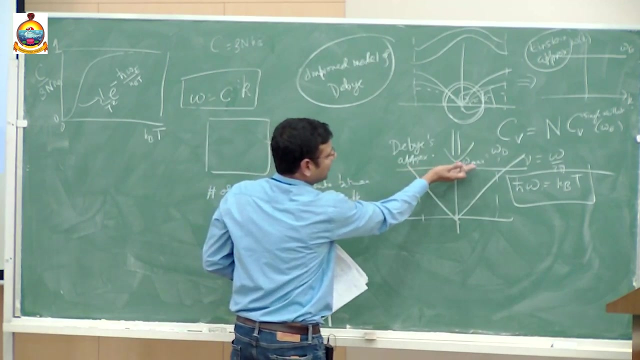 n. That is it. So once I get that omega max, that is what the target is, and then everything else will follow. So that is the only free parameter here. Good, So I hope now it is clear, right, Because I need an omega max Without an omega max. 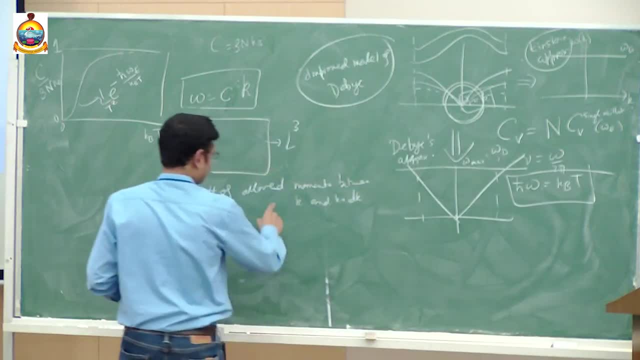 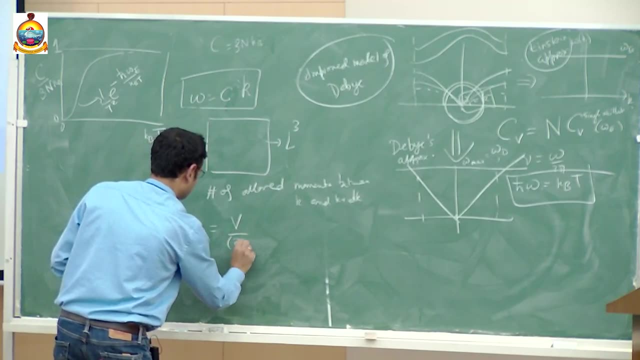 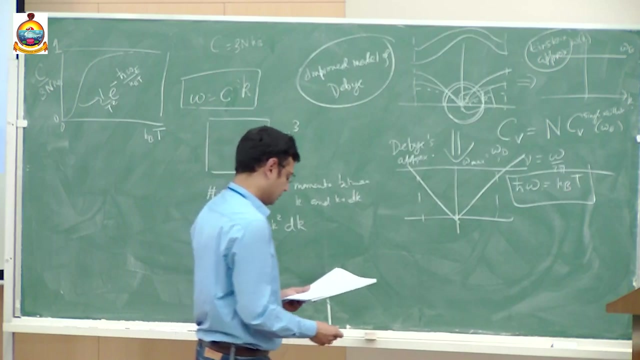 of course, the. So what is this number of allowed momenta? This is simply this. we have seen many a times. This is simply this. And then, of course, if I have a function in k, then I can use this property, And if I have a function in k, then I can use this property. 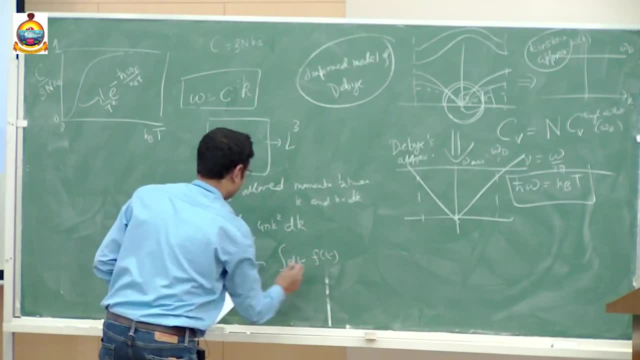 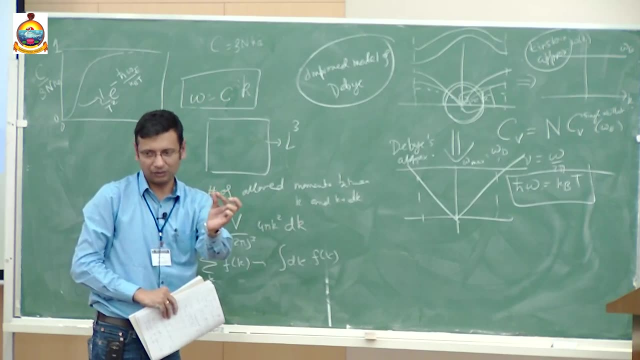 And then, of course, if I have a function in k, then I can use this property, And if I have a function in k, then I can use this property. And if I have a function in k, then I can use this property, And if I have a condition that can be used, I can use that. Now I have 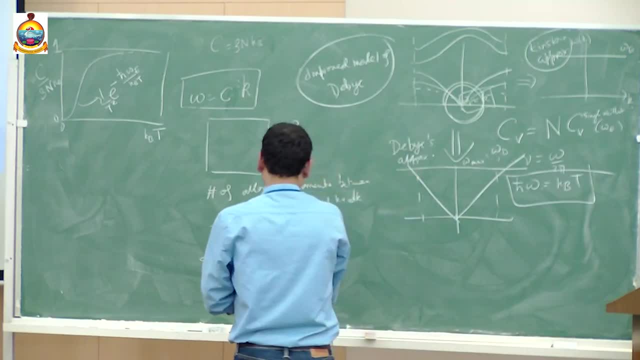 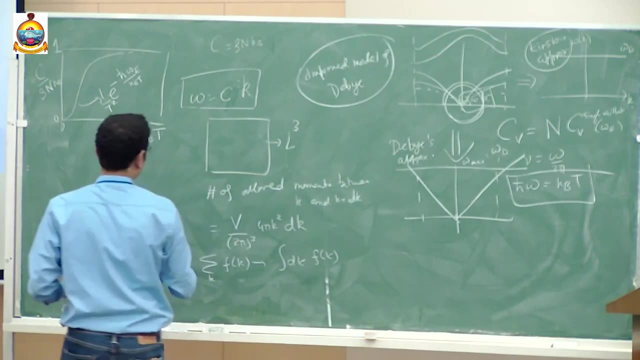 to do the same example from this point: How to move from a point K, How you will move from point K to point integral. Well, personally, I have been doing all of this And I have done this And based on this, 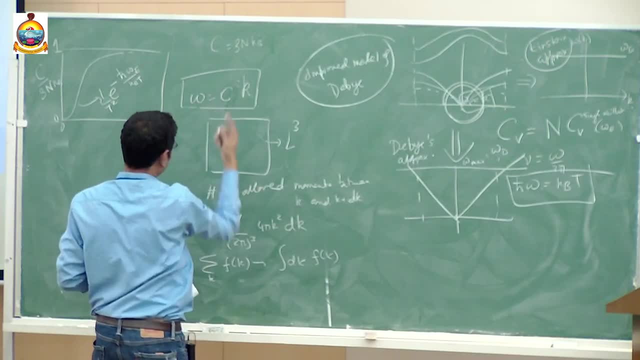 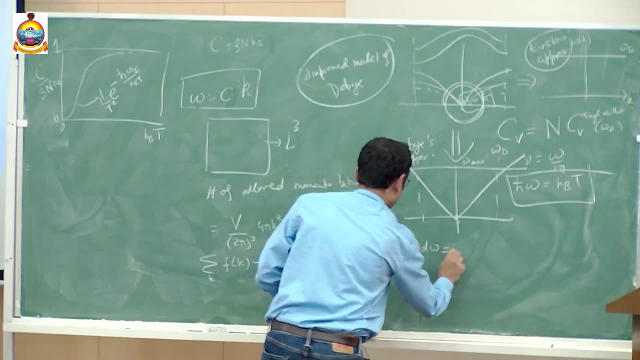 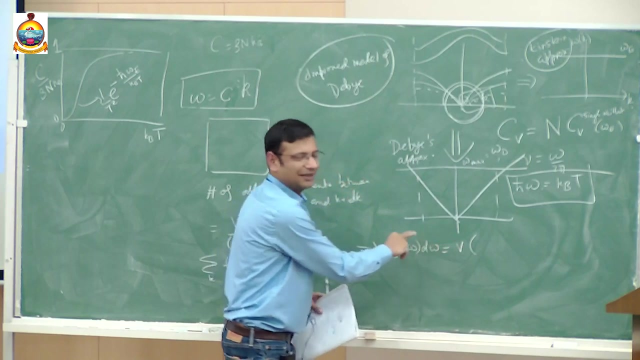 I have to also move. So that is also very easy. I mean, I just use this relation and I can do that. So basically, if you wish, the density of modes is just this. In fact, when I write this, I will also insert: 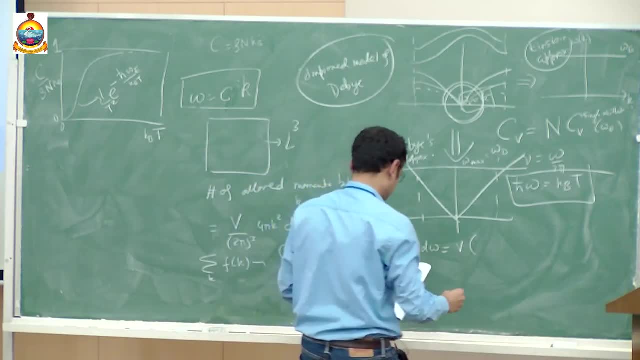 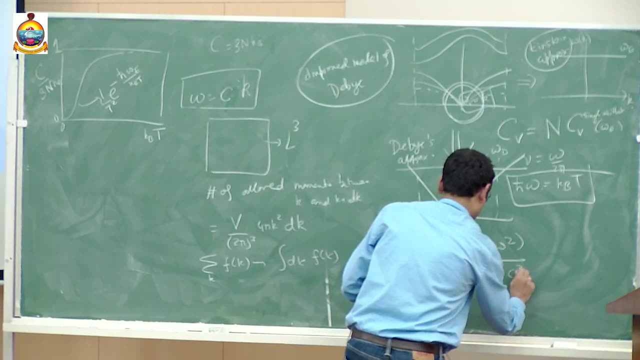 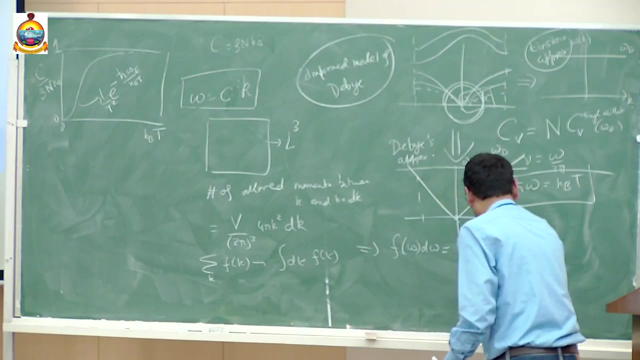 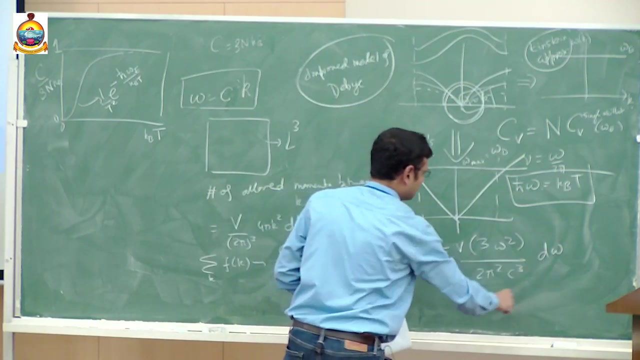 the factor 3 here, just to account for the 3 polarizations. So, as always, I insist you to check my algebra. I may make mistakes of factors of 2 and 3 and whatever, but this is essentially the thing. Now. these are the number of modes that I have Between omega. 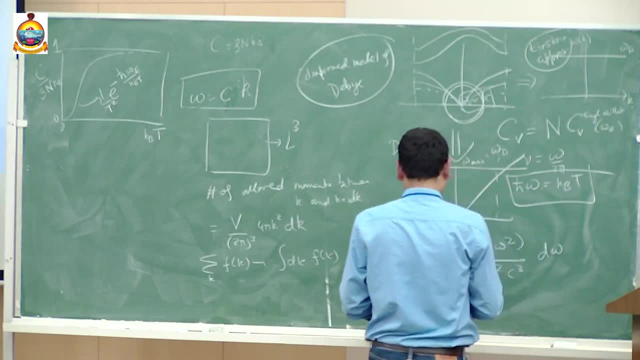 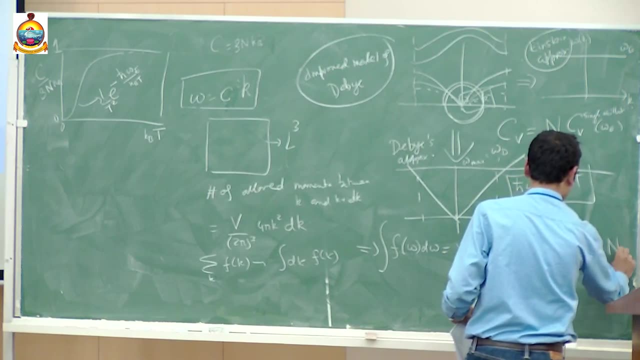 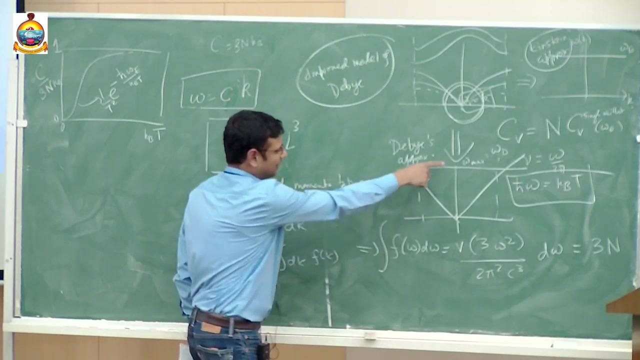 and omega plus dv, Right? So now I need to do an integration here, and that integration should be equal to 3 times n the total number of modes in my system, Right? So can somebody tell me what is the lower limit of the integral and what is the upper limit of the integral? 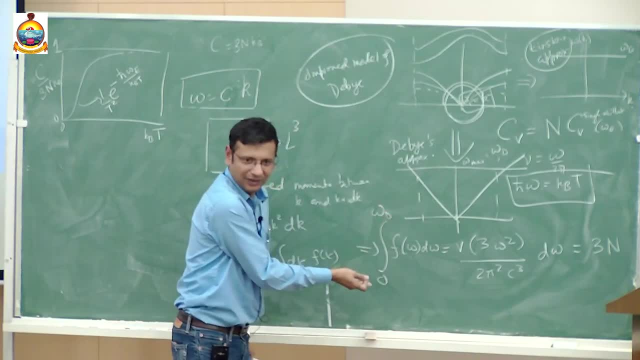 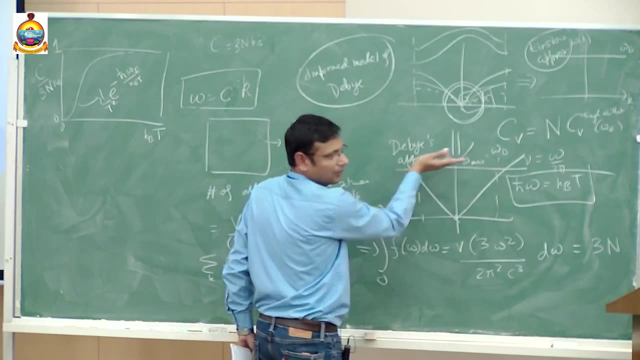 Yeah, 0 is obvious, because we have gap less modes here. we have to start from 0. that is the most important thing. And of course, as I said, we want to cut off the integral integral at omega d. So this count is correct. That is it. So this integral will determine. 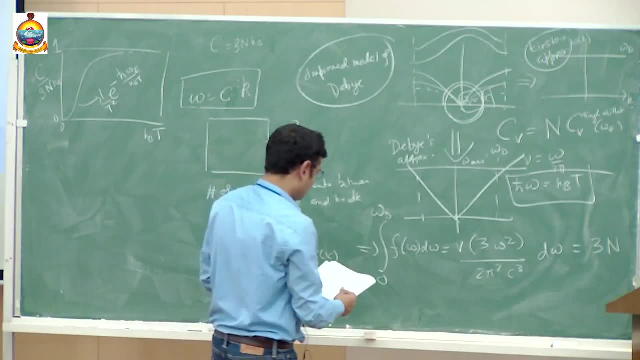 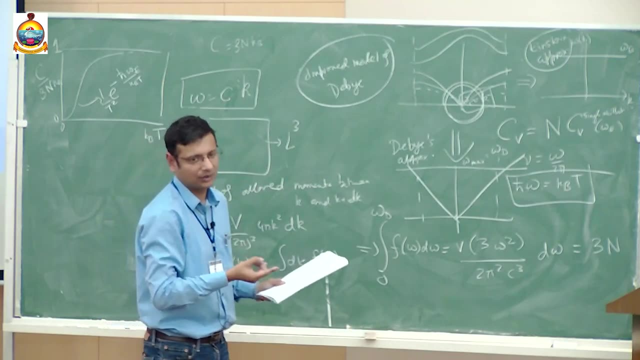 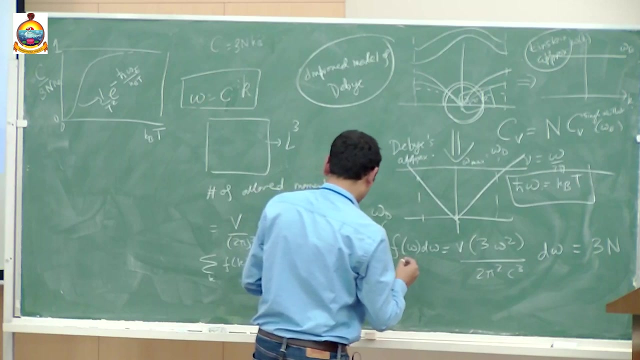 omega d. There is nothing else here, So that I will do So. while doing this calculation, I am adopting basically the notation of Carson-Huang, So if there are some confusing steps, you can always also refer back to Carson-Huang. So now there is another notation I introduce. 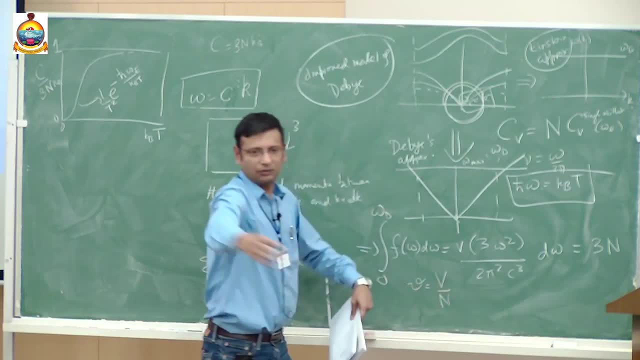 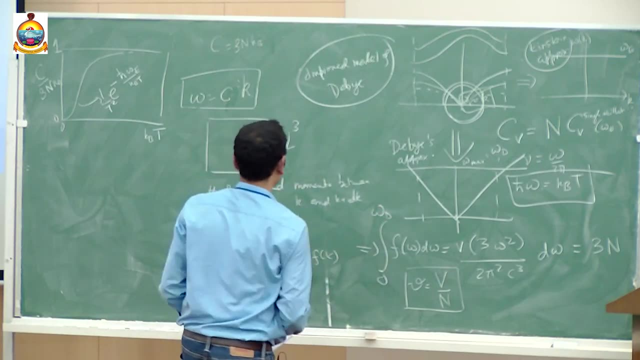 this small v, which is volume per unit cell. So volume of the total sample divided by the number of unit cell, small v. So this is another notation I introduce. So let me keep this here and let me erase that part. Speed of sound: as I said, it is not the speed. 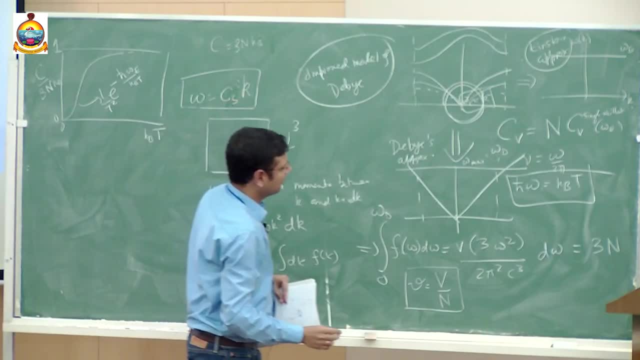 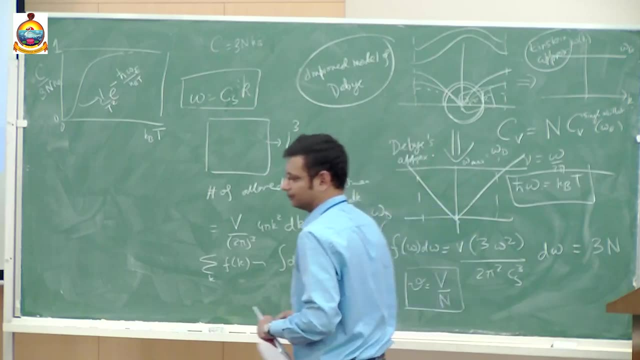 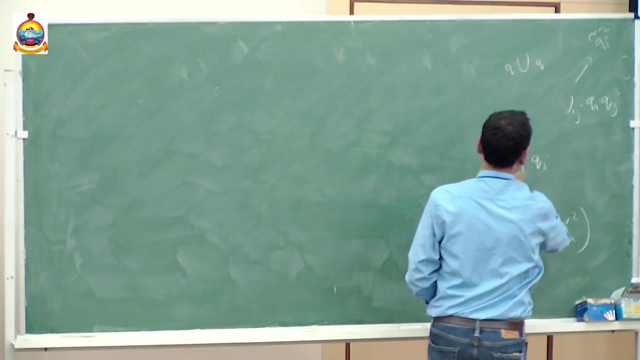 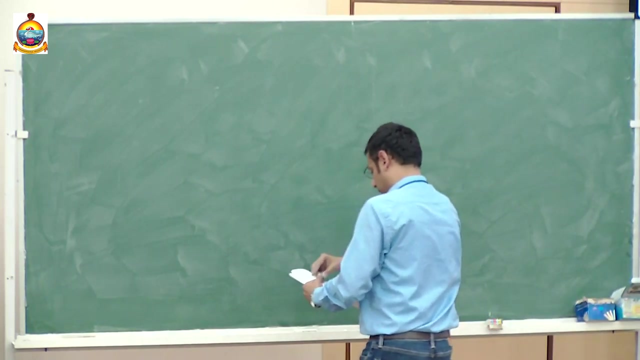 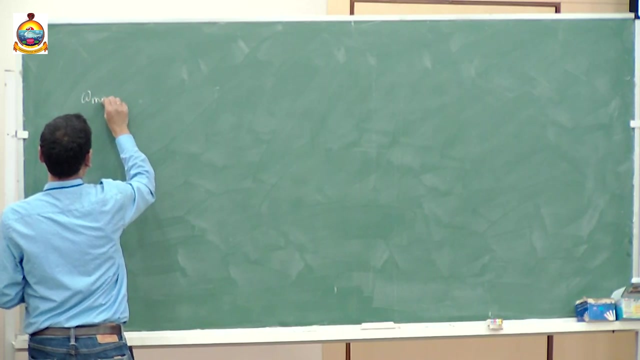 of light. So c sub s. if you wish, So c sub s, Yeah, Thank you very much. So then you can actually do what you can see. So omega max or omega sub d- I use them interchangeably- is the following: 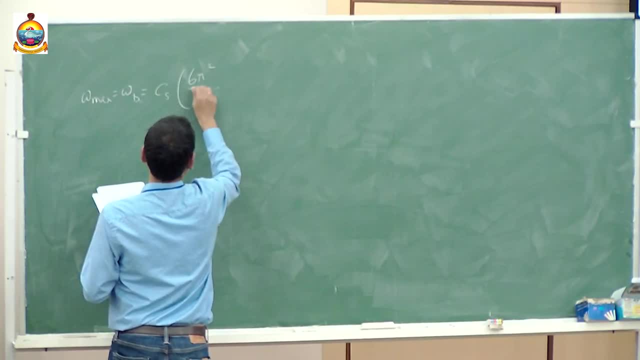 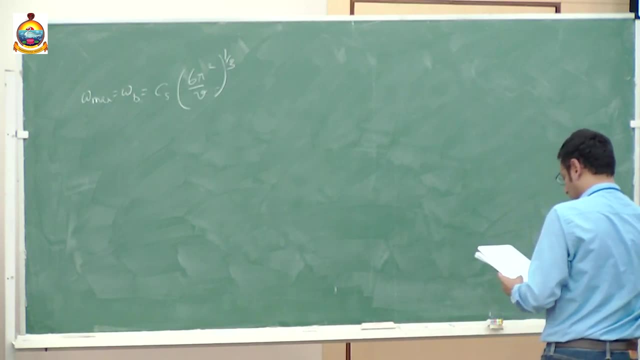 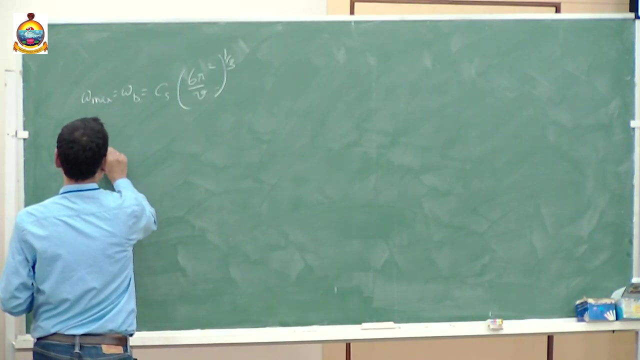 C sub s, 6 by square, by v. Yes, Power, 1 by 3.. So I just solve that integral and I get this answer. So I know omega sub max, Good. So now what else do I mean? I just recall the result for the harmonic oscillator. 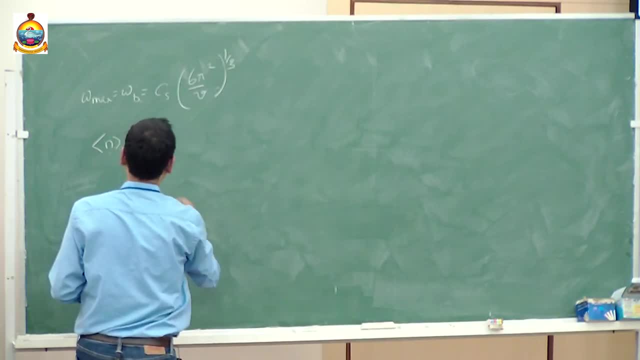 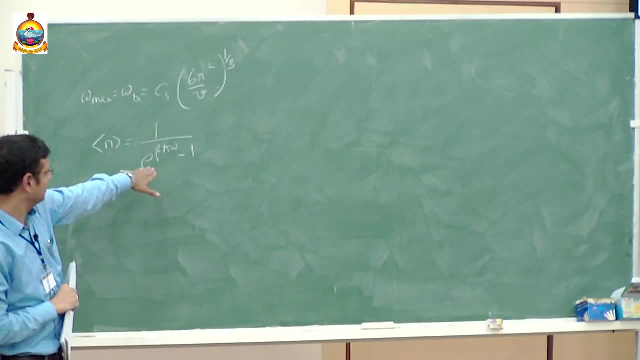 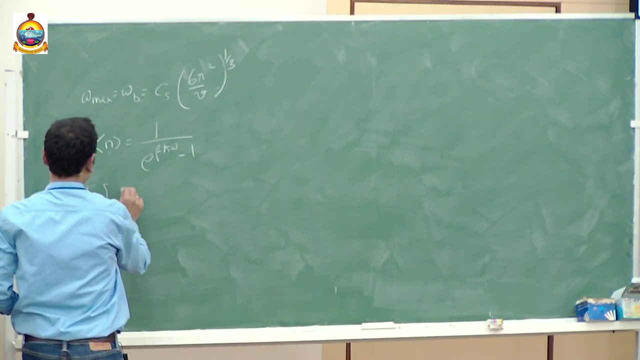 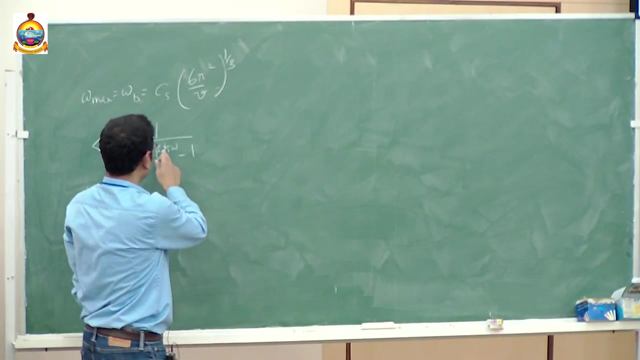 problem that I got. So I remember what expectation value of n was for the harmonic oscillator. It was this. So this you recall from the last class we got this. So this was. So in my case, this one I will take as the value of Greek. 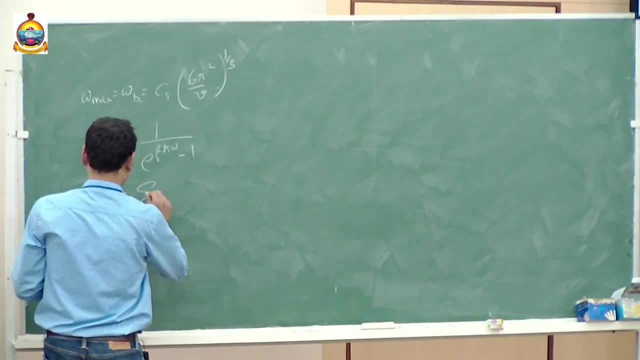 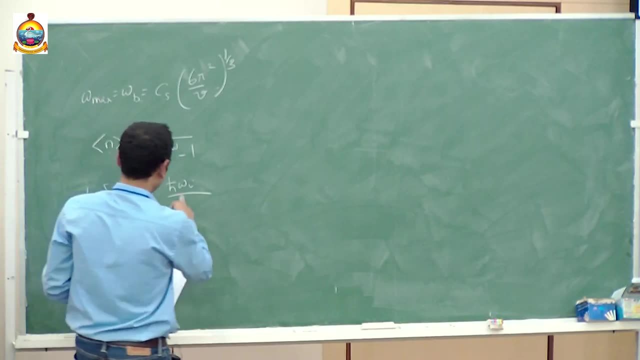 mass 1 by k dusty negative 30.. Yes, From producto, 꼶 of n is equal to 0.. No, I got it here, Jesus Christ. All right, Had I known this before? Yeah, mode, let's say, has a Omega I, Omega, sub I. so this is the contribution from each individual mode. why? 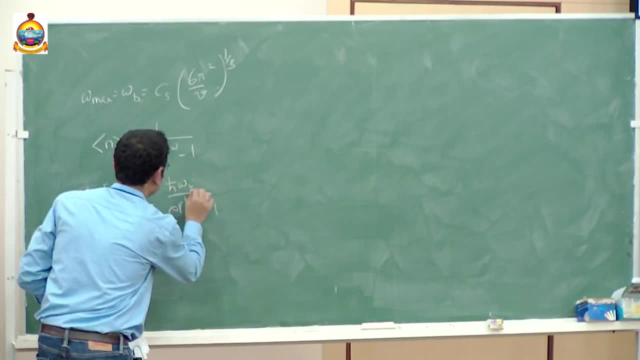 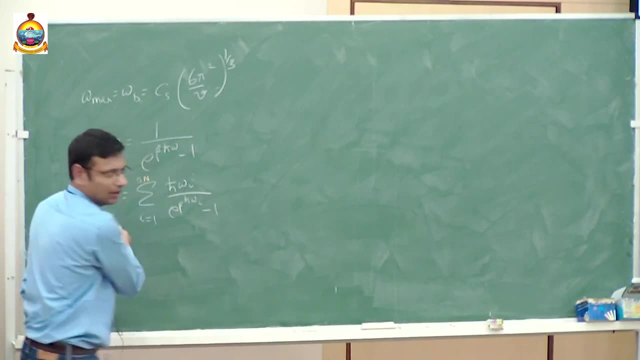 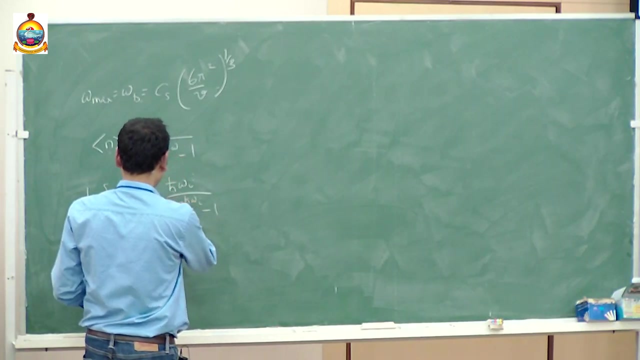 because this piece, this piece is the energy of the mode and this piece is the expectation n. so expectation n times H, cut Omega, I gives you the total energy, right. this is, I hope, completely clear to everybody, right? good, so then the? I do the usual trick. I already told you what is the. 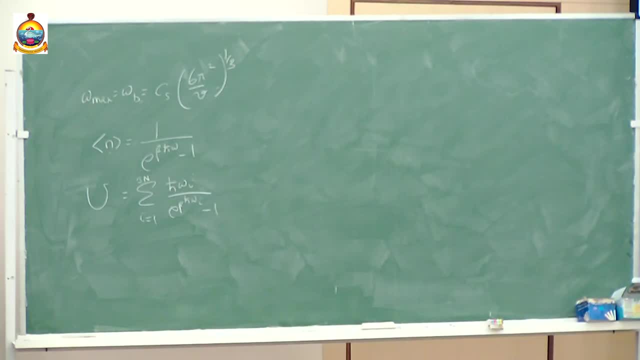 density, F Omega, D Omega, of what is the number of modes between Omega and D Omega, like this: I just use that result and just write this as an integral right. so the integral will of course go from 0 to Omega max. and now comes the integral, which I'll just 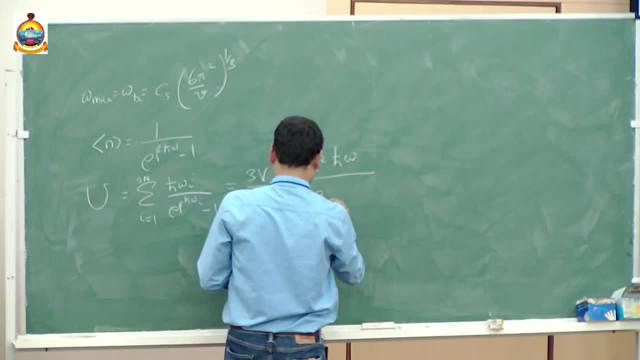 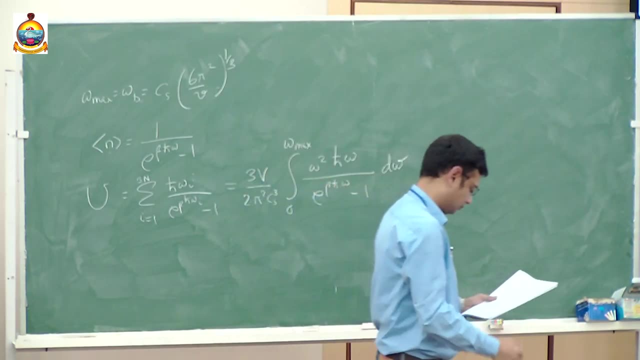 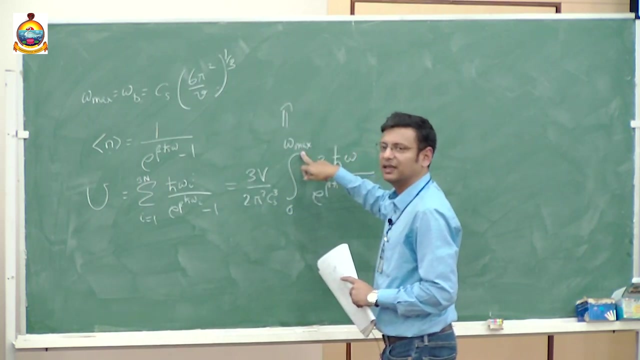 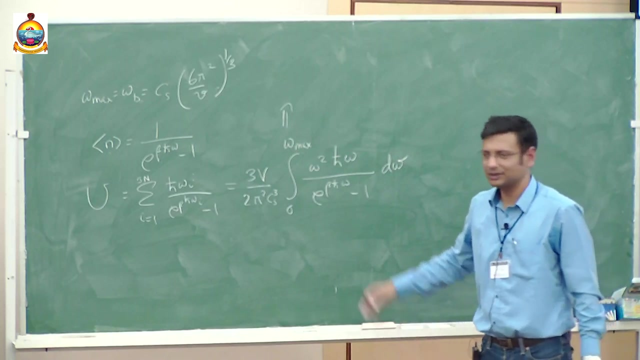 write carefully, slightly okay. okay, so far, so good. also, traditionally- and this is also written in many experimental literature- from this Omega max people define a temperature score, a scale called the Debye temperature scale. okay, suppose I give you the Omega max. how can you get a temperature scale? can just sorry. 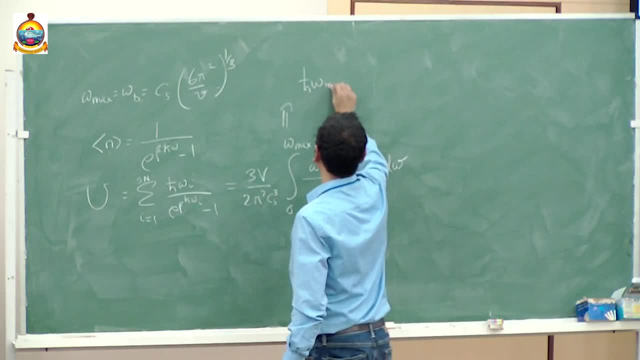 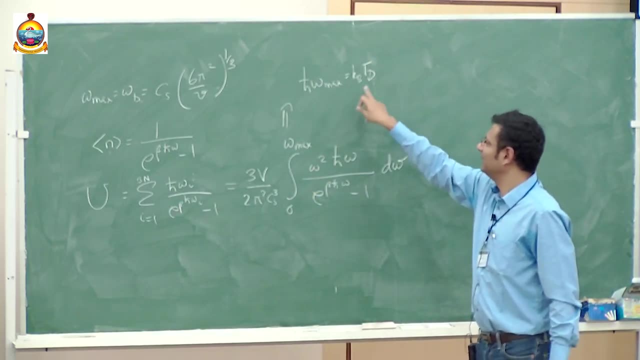 H cross. Omega max is K, B, T, T, Debye, right, and this is actually a number which many experimentalists quote. this is called the Debye temperature and the debug roughly okay. so basically what I'm saying is that the temperature of the temperature, of the temperature of the temperature, 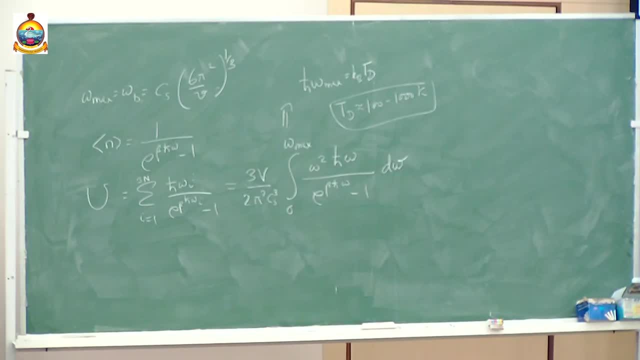 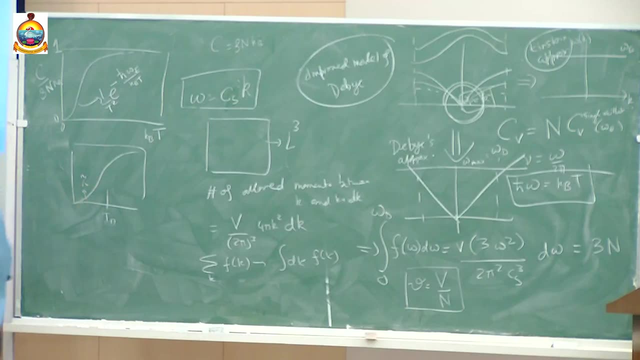 what does this temperature scale indicate by? if you're much below T, Debye. so I just plot this graph again: T cube behavior and so on and so forth. so this is like a relevant temperature scale in that sense. okay, good, so now we need to do some mathematical jugglery, but it's not very complicated. 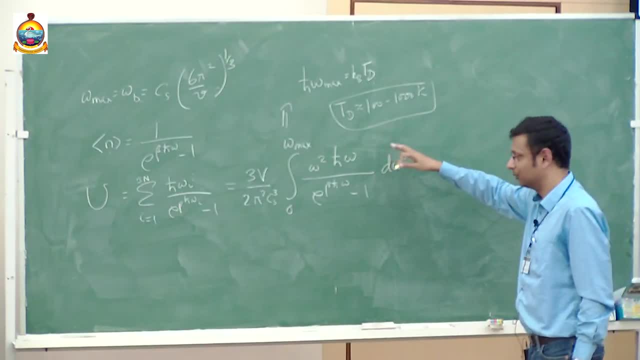 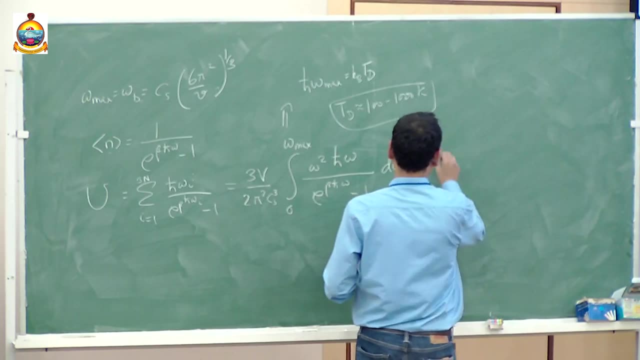 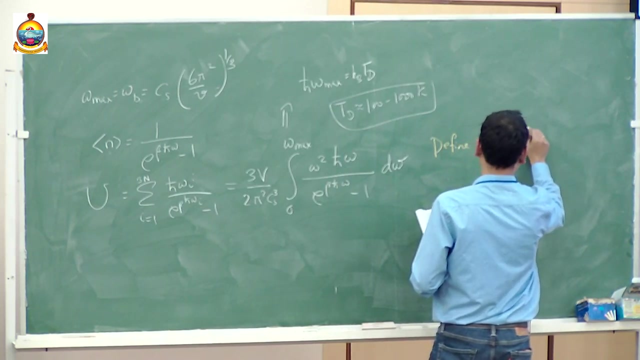 so let's just do that, Carson and Carson Wong, so you can see the steps there. but I'll explain everything. it's very straightforward, okay, so so first I want to define some dimensionless parameter like this: so this parameter is clearly dimensionless, right? this is here to everybody. this is a pure number. this does not carry any units, okay. 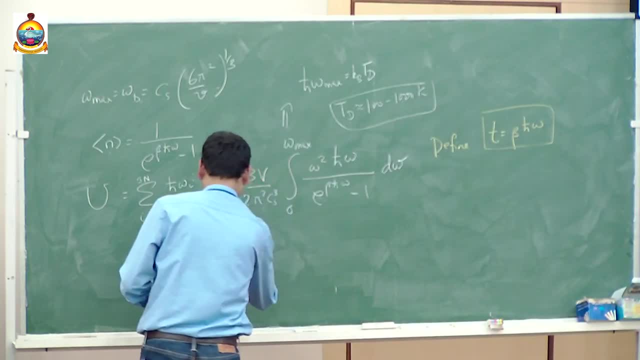 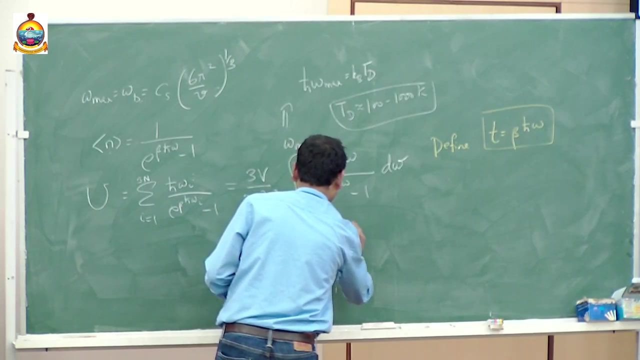 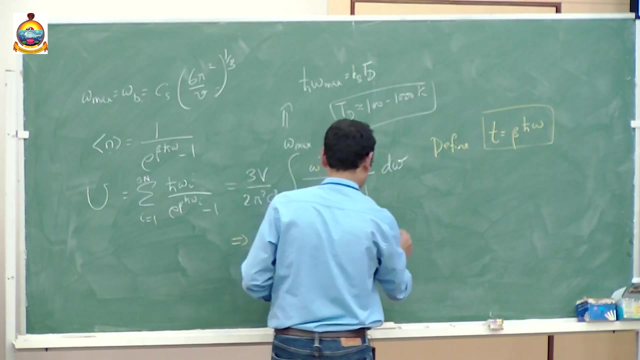 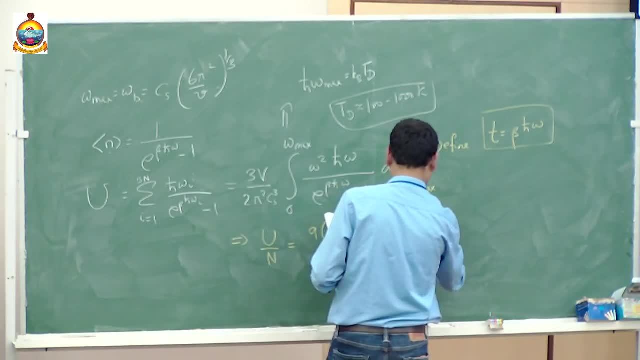 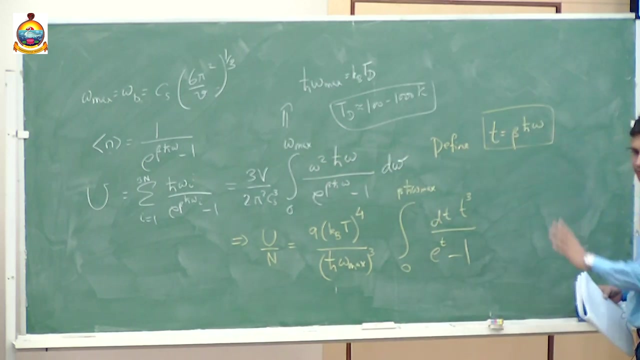 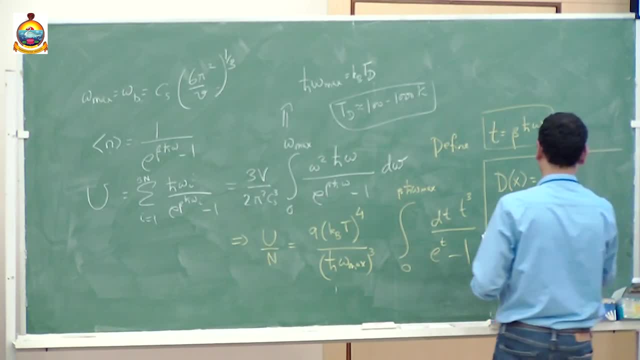 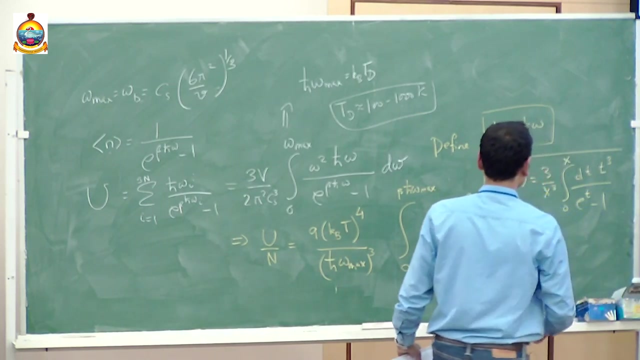 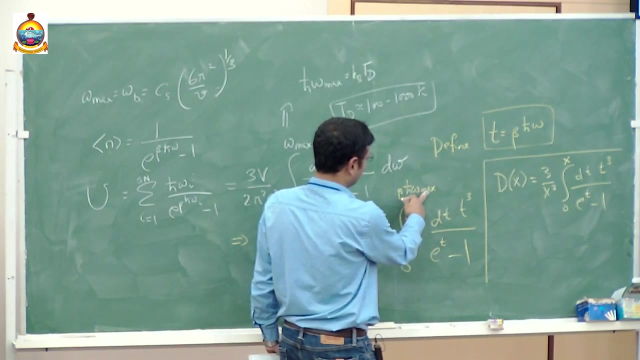 text books. this is called the Debye function, what I am just going to write down. So you can see why I wrote it like this. because look at this limit. This limit is some beta h cut omega max, and that exact same thing is coming as the third part. 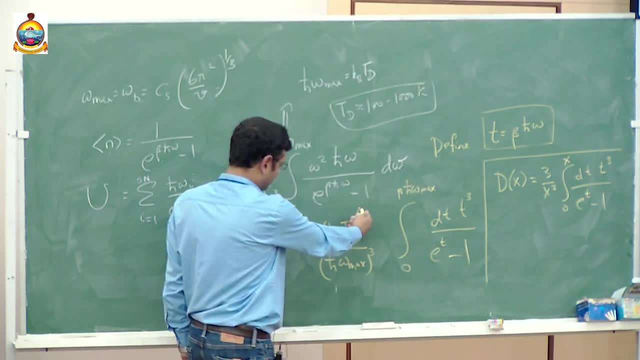 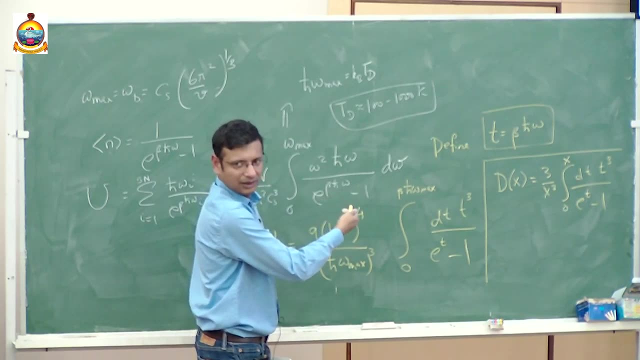 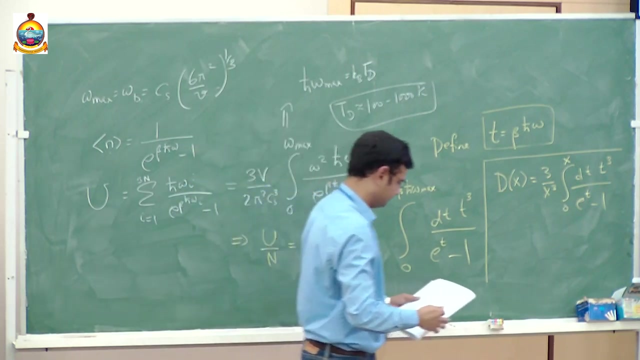 And of course I need to pull three powers from here inside, but essentially it is this form, and then there is some one power of temperature hanging outside. So if I get this form, if I know what happens to this D, then of course I know what happens here. So now we will. 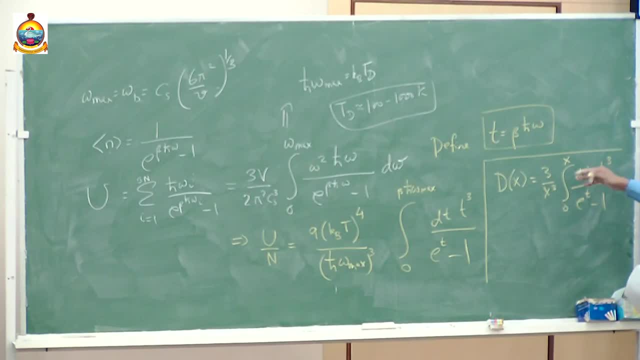 do the usual thing, we will. So this integral is a bit messy. I do not know whether there is a straight forward way to calculate it. For all x, Whatever, it is just a constant temperature. Yeah, that well, no, no, no, there is x here. Please remember that there is x and this x. 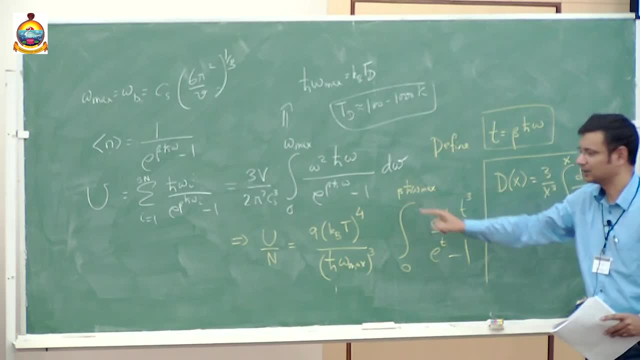 depends on temperature. this x depends on temperature. Yeah, yeah, yeah. So it is not so easy, otherwise I would not bore you right? See, it is a funny integral right. So it is 0 to x and the x contains beta, and there is an x here and there is a t hanging. 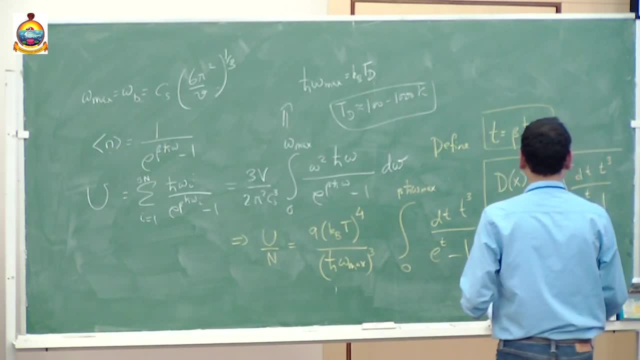 around outside. So let us do the integral in the two limits that we always do things in: x much, much less than 1 and x much, much greater than 1.. So if x is much, much less than 1, what does it tell you about the temperature? 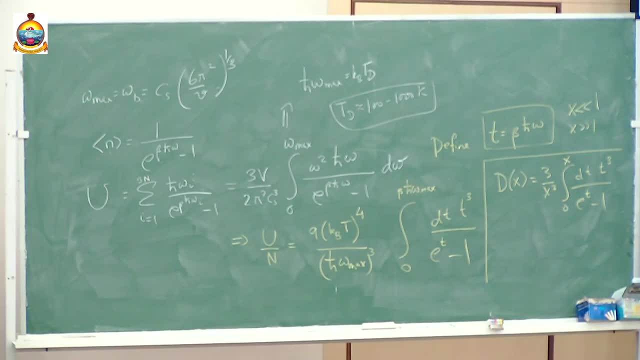 Yeah, If x is much, much less than 1, then beta is much, much less than 1, right? So t is very large and the other limit is, of course, the other way around. good, So if- let us first start with this guy- x is much, much less than 1, then how should I approach this integral? 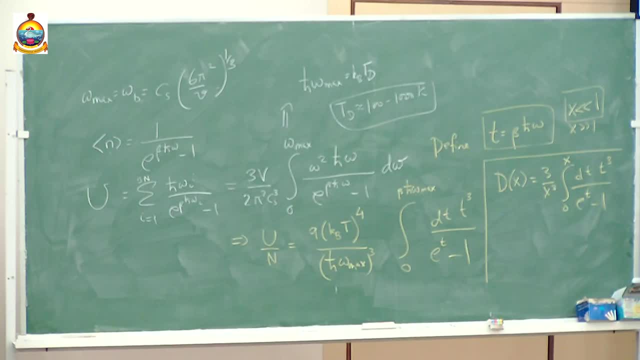 I mean, what do you think? So just try to do it. just tell me the steps and I will follow you. How should I do it? I need to simplify it right, because this is not obvious how to do this. So it is about. 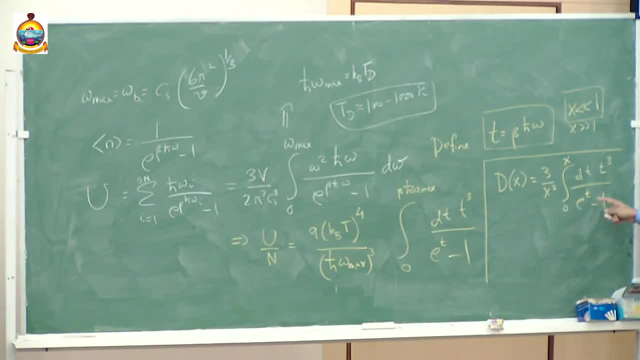 Or whatever order, right? So this is clear, right? See, x is small, that is your integration domain, So t is always small, because t is always small. therefore, e of t, I can do 1 plus t plus t, square by 2, factorial plus. so on, right, I can do that, right? good, So let us. 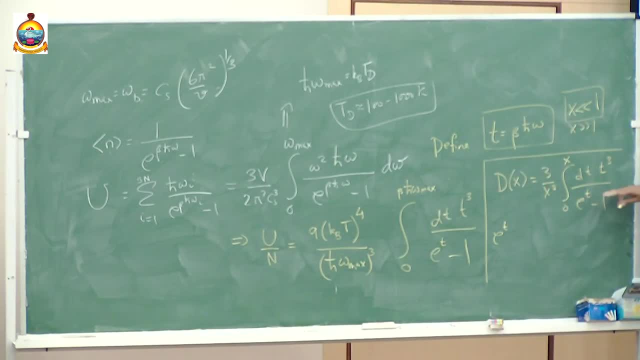 do that, Then it becomes a simple integral, because then there is some power here and then I just take it to the numerator and So let us just do that. So basically it is t plus t, square by 2, factorial plus so on. Let us just stick to this order. Let us say: I just stick to. 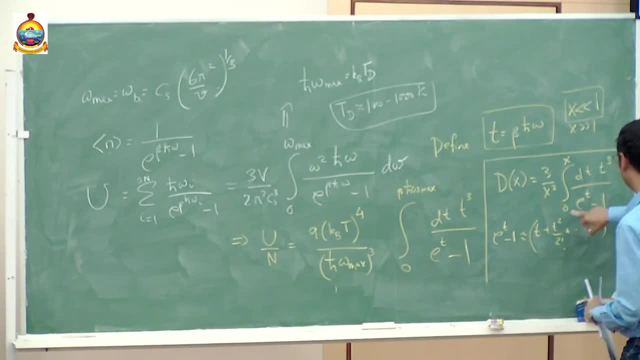 order 1 to t. then you see what is happening here. There is a denominator which is t, then there is a t cube, So that gives me a t square. So when I integrate, that gives me a t cube by 3 and that exactly cancels this object. So I get 1.. I get 1 to leading order. 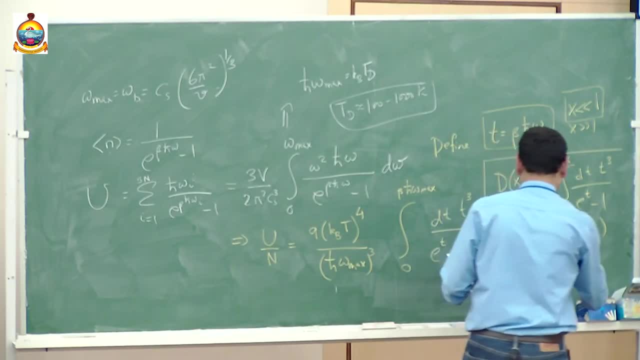 good. So that is, that is good. Then to next leading order. I can just use this and this is what I will get, So I just take this upstairs Right and so on, So then you can calculate this right. So I will just write down the 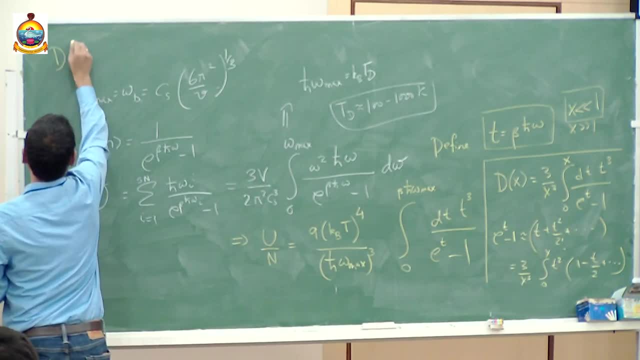 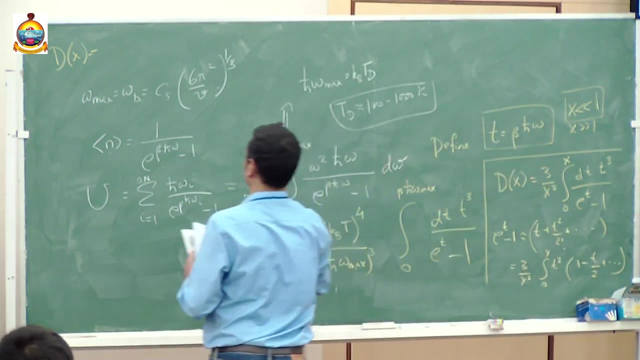 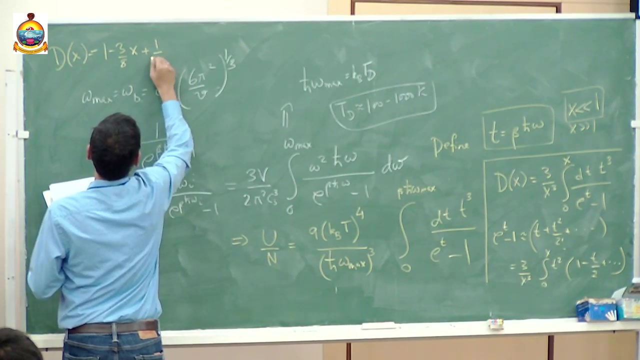 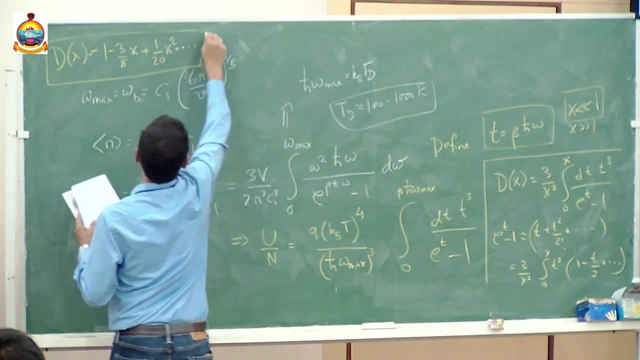 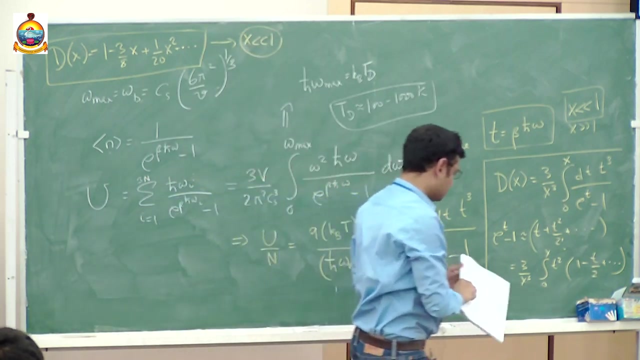 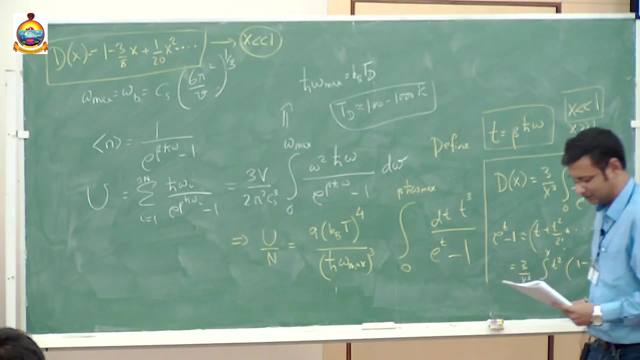 result here for small x, and of course you calculate it to any order by Taylor expansion. let me just write the behavior for small x. ok, good, so far, so good. now please tell me what happens when x is very large? now we go to the opposite limits. so what happens when x is very large? how would 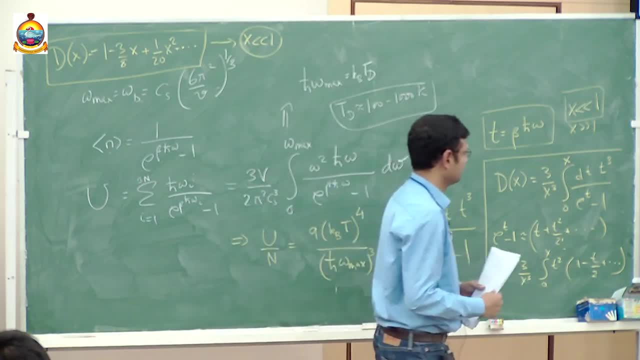 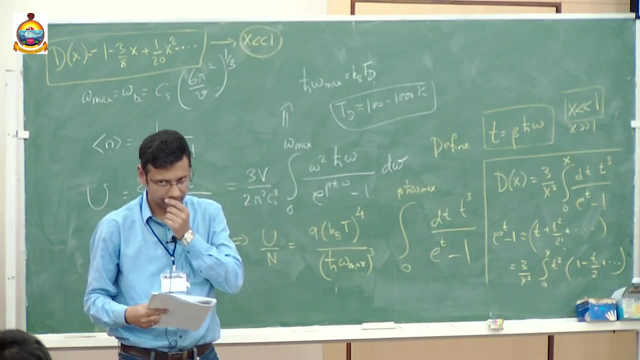 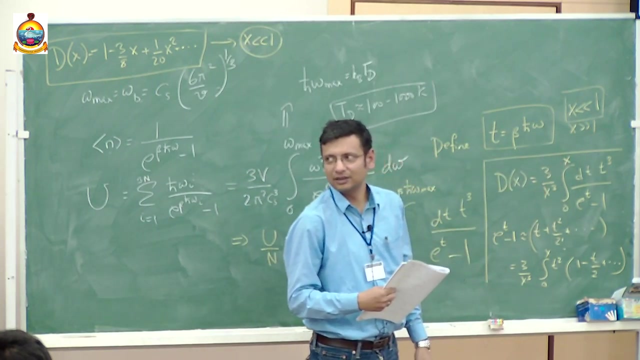 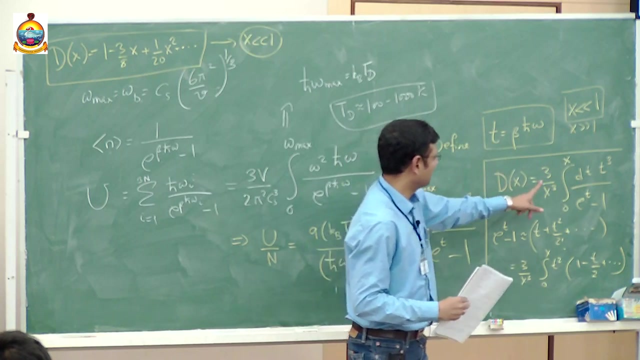 you approach this problem. so x is very large, i mean, what do you expect then? i mean it should be clear: what do you expect? what is the leading form of t? sorry, one, one by one. so if x is very, very large, what is the function i will get on the right hand side? 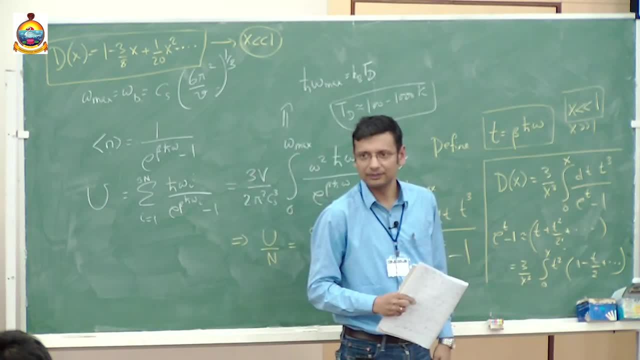 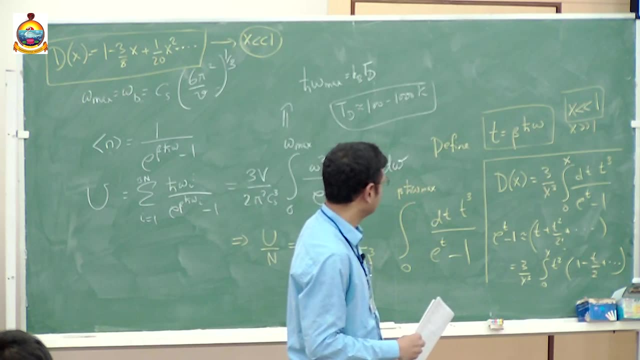 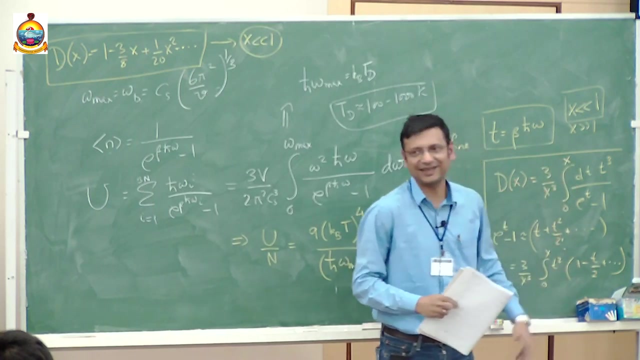 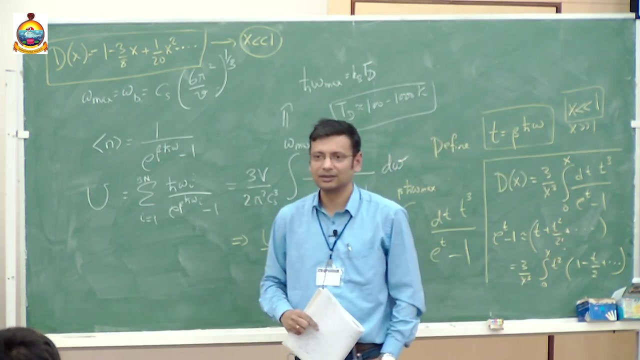 one person at a time. there are too many things. just talk a bit loudly. no, no, there is no t and all here. there is only x here. just tell everything. there is no t, there is just a function of x. where is the t here? what is this? when x is very large? now, what is it? i mean, i am. 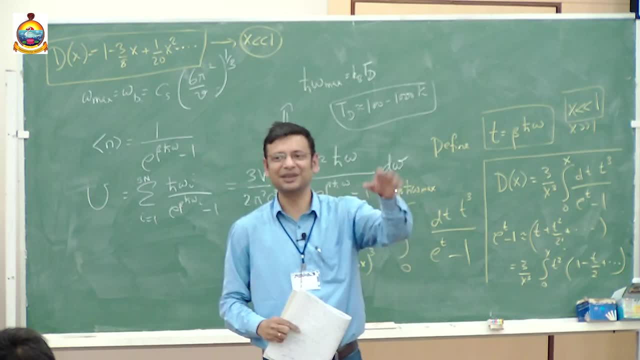 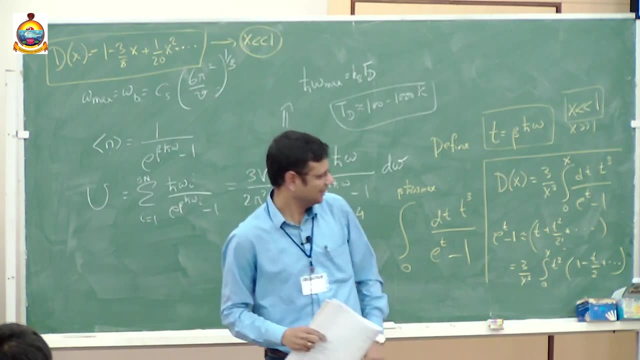 not, i mean just tell me the approximate form. if x is very large, what is it? i mean, i am not. i mean, just tell me the approximate form. if you wish, There is some number you can ignore, But what do you get? Constant, No, I mean. 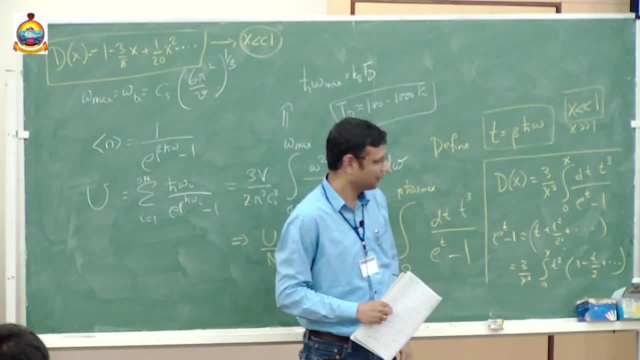 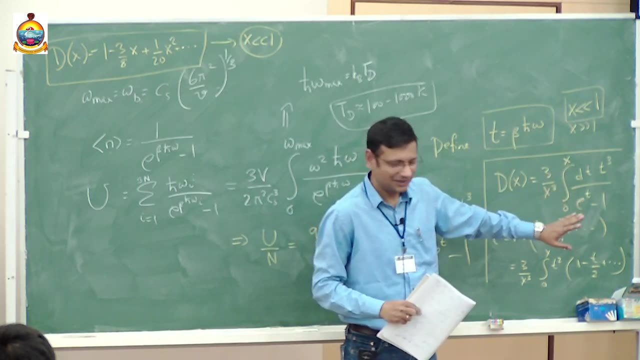 just look at it. It should be absolutely clear to you. What is the No, no, no, no, no. Okay. If x is very large, this integral can be replaced from 0 to infinity. Right, Okay. Now what? 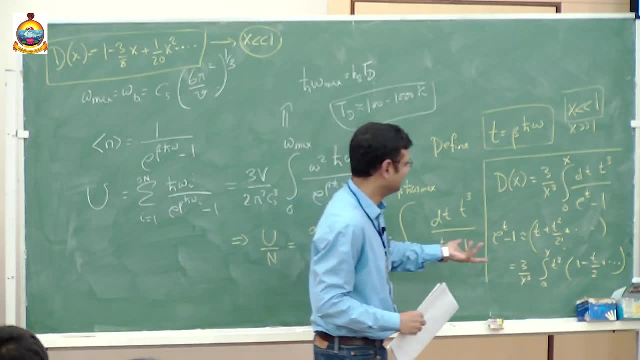 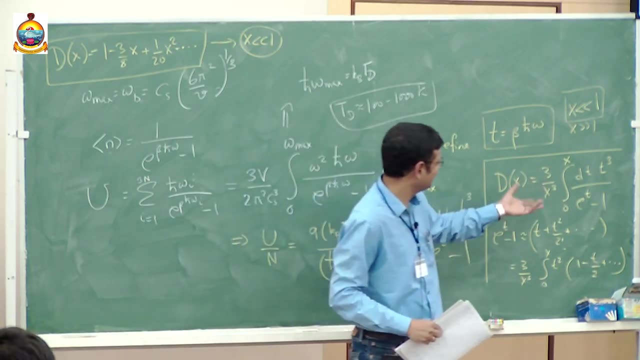 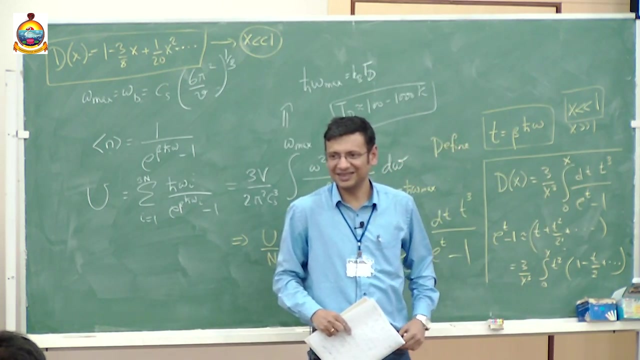 is the behavior of this integral. I mean, does it give you a finite number, infinite number, Finite number. So the leading behavior at large x is this: finite number times 3 divided by x cube. Is there any disagreement? It is some number divided by x cube. No, no, no. 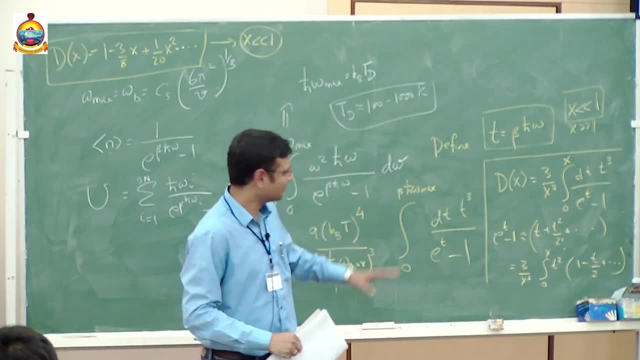 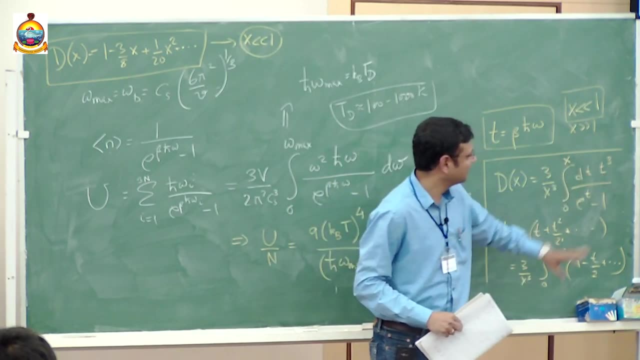 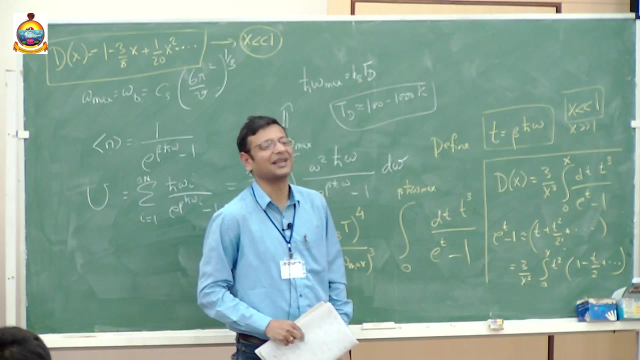 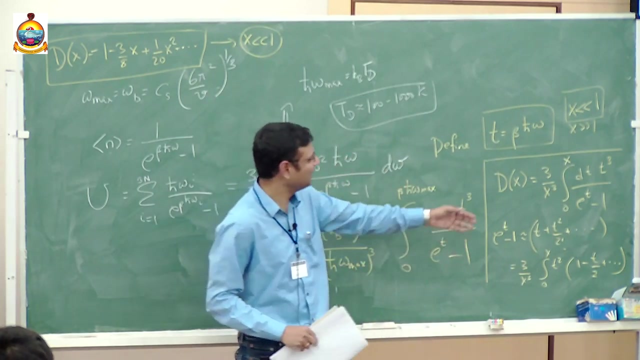 I said x is very large, Correct? So the leading behavior at large x is just some number Divided by x: cube. Okay, Why is this integral finite? Is everybody clear on that? Why is this integral finite? Why are you speaking? Okay, Anyway, he answered it Anyway, for. 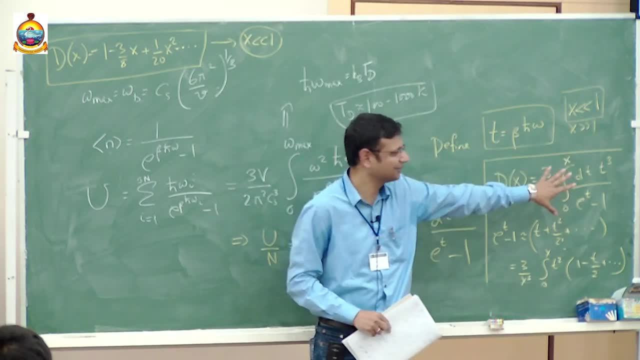 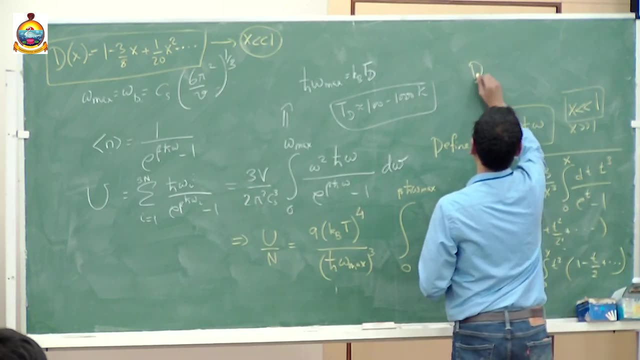 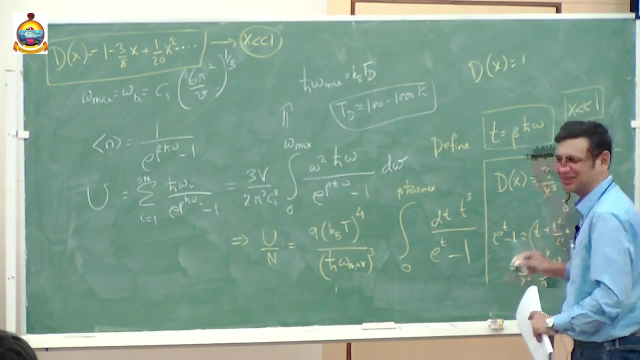 the lower limit and the upper limit, both the limits, it converges, So it is a finite integral, Right, Okay, Good, Okay, So in fact you can even calculate this integral. So you can. Thankfully, I could see the answer in Kersenwang, So I did not calculate the integral. 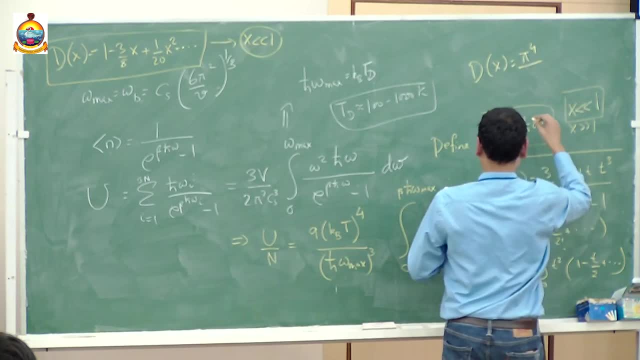 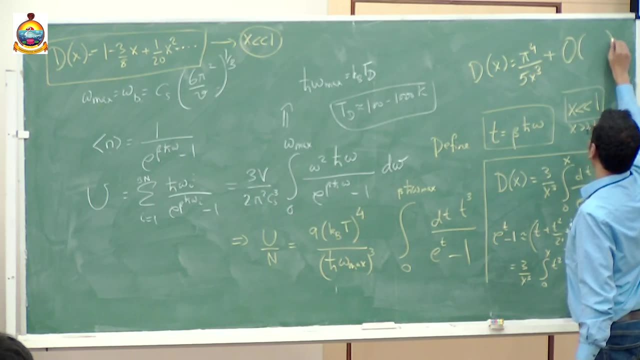 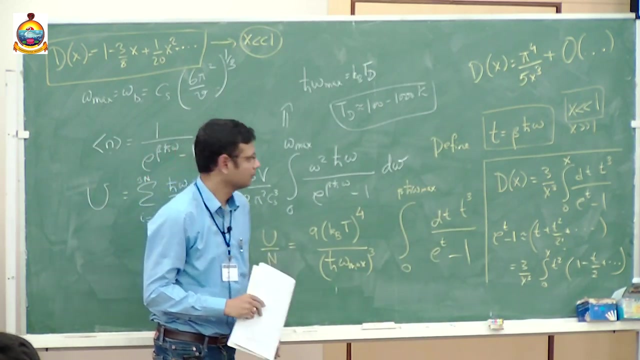 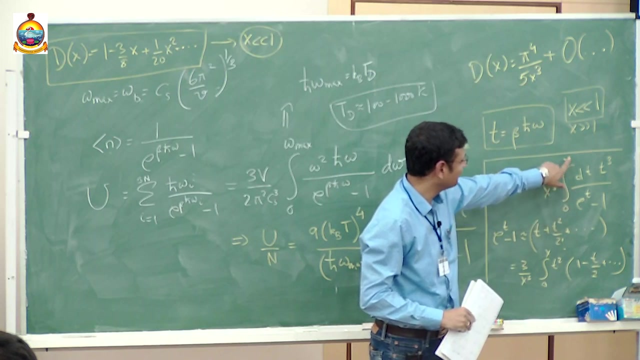 But okay, Okay, So this is the leading piece. Now comes the next question. What is the next piece? What should I write Plus what? How do you approach this problem? Now? think carefully. What is the approximation I made? I replaced this integral from 0 to x. I replaced from 0 to infinity. So I made some approximation. 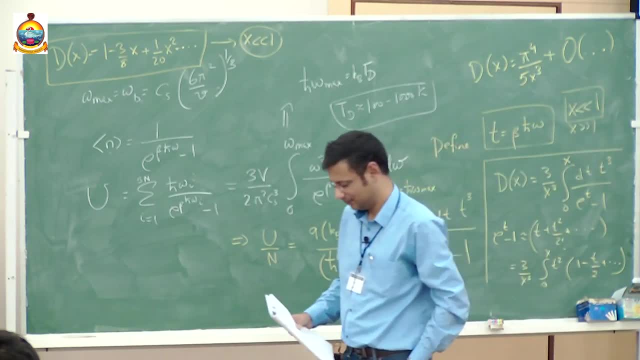 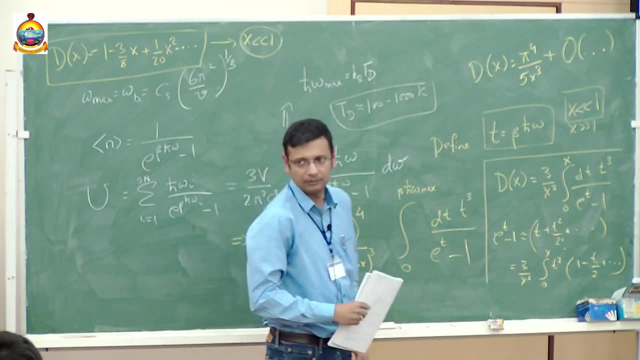 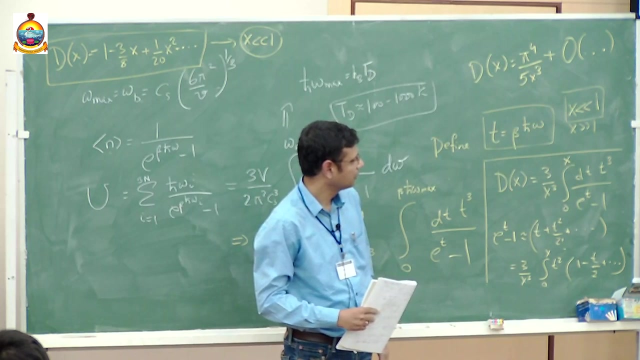 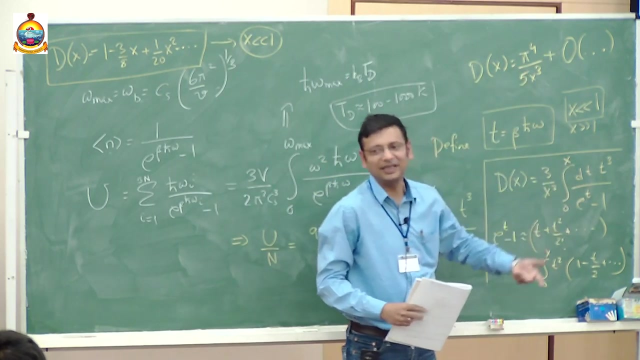 Right, So now, what is the sub leading correction? 0 to 1.. 0 to 1.. Yeah, So there is no. There should not be 1 here. X is very large, So to calculate this I just replaced x by infinity, but then I am of course making a. 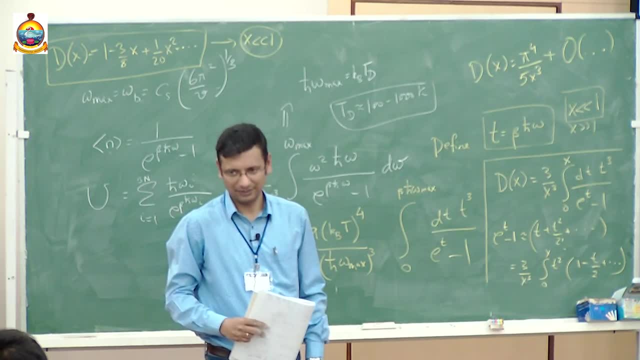 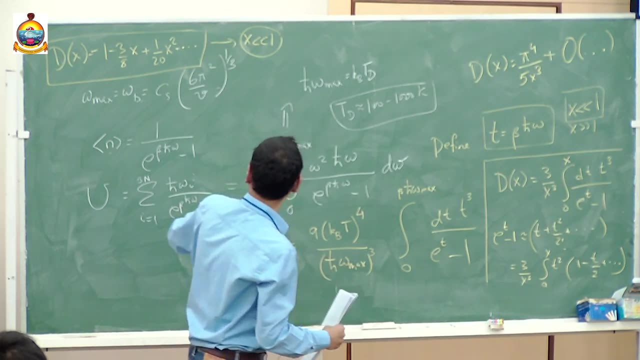 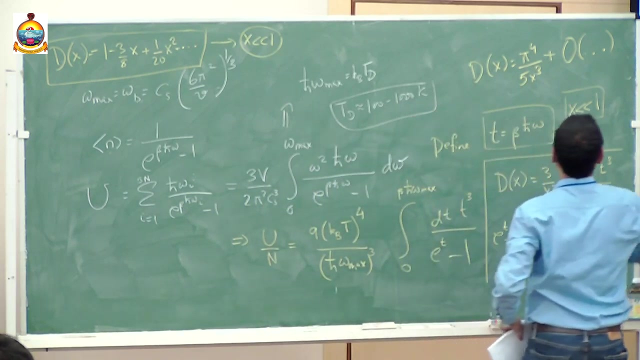 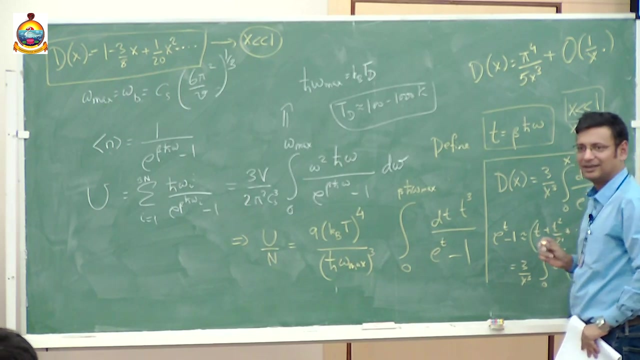 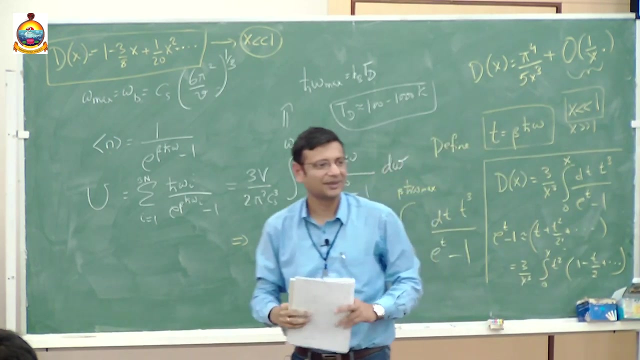 Yes, yes, That is correct, but for the smaller values of x, you got this kind of an expansion, linear in x. Do you think this would be, for example, 1 by x? Do you think so? 1 by x to the power 4, why? 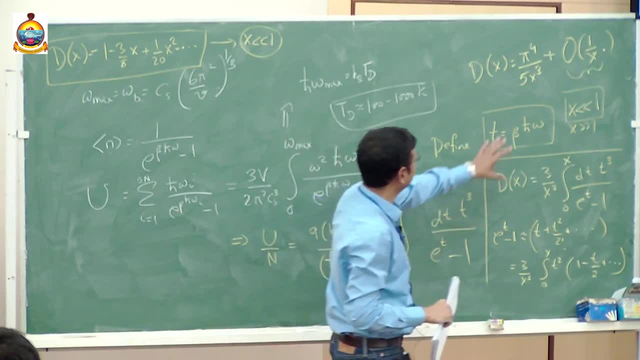 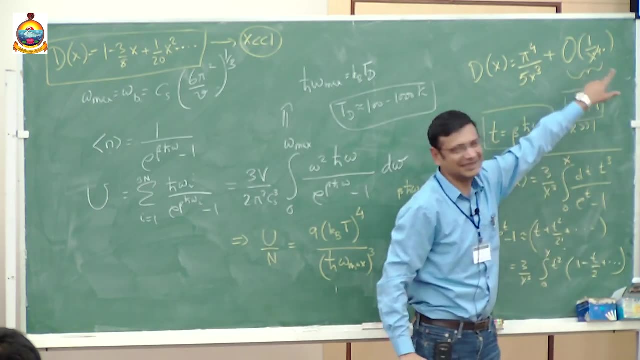 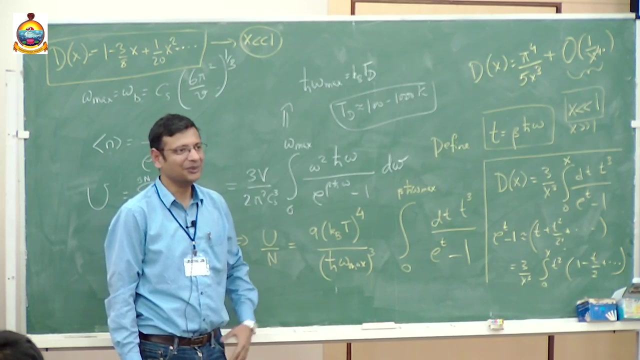 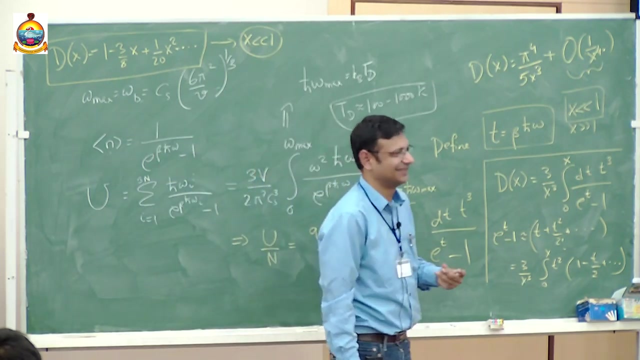 What? That is already there. This is the leading behavior. Sorry, I get what you mean. So do people think that this is the answer? How many people think this is the answer? Nobody thinks this is the answer. Just now, you were thinking that this is the answer. 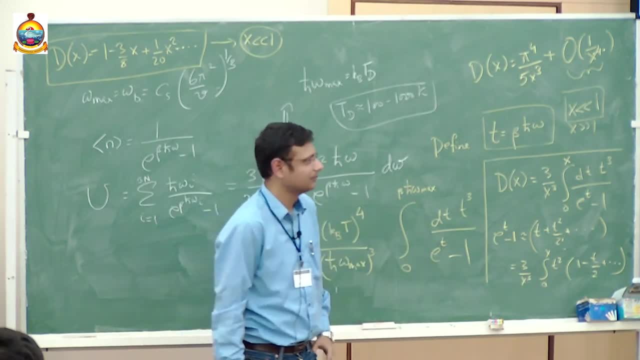 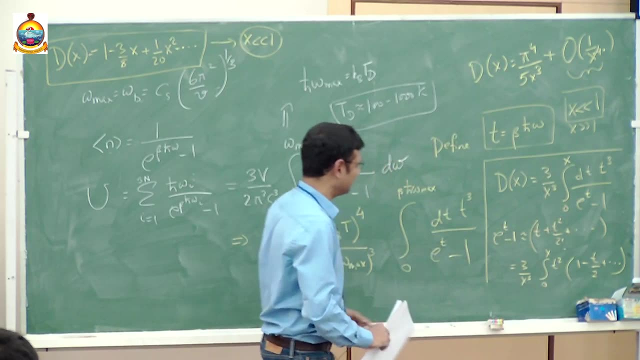 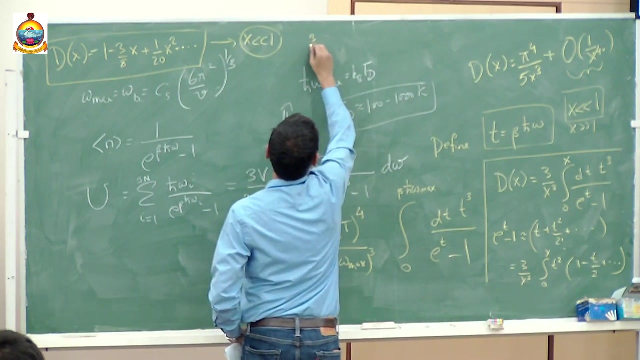 What is the answer? No, let us think a bit right. It is not very hard right? How did we get the leading term? So where should I write? Let me write there. So the way I got the leading term was: 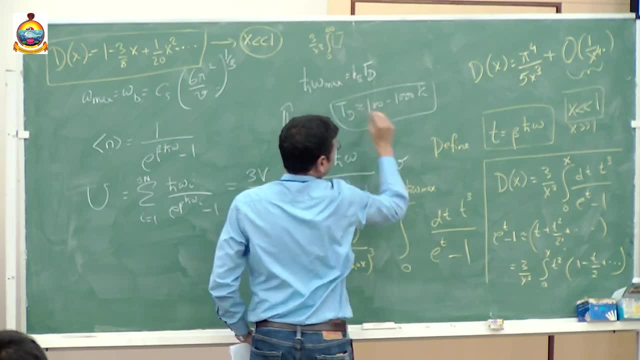 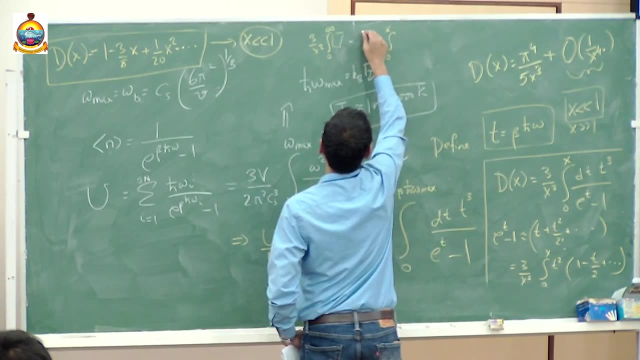 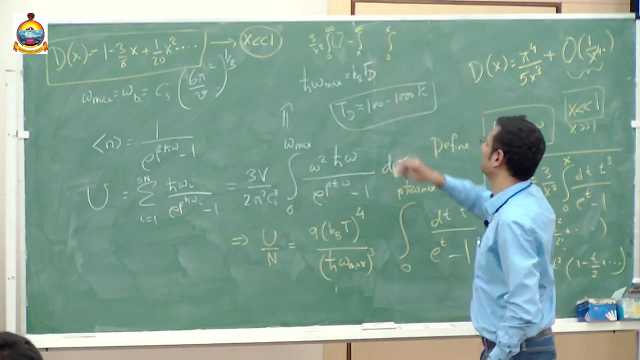 I replaced this integral to 0, to infinity, some integral right. But what is this integral actually? This is actually this right. So then, effectively- sorry, effectively- I need to do something like this, some subtraction like this right Of this object Now can. 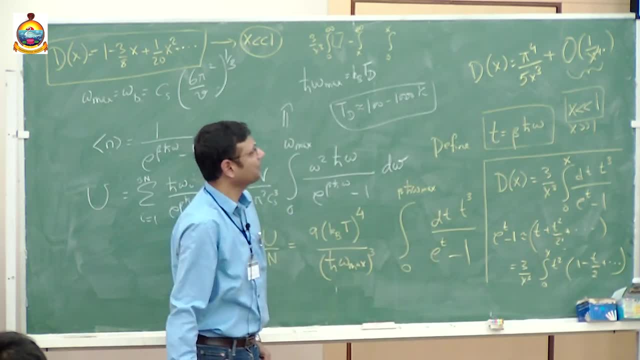 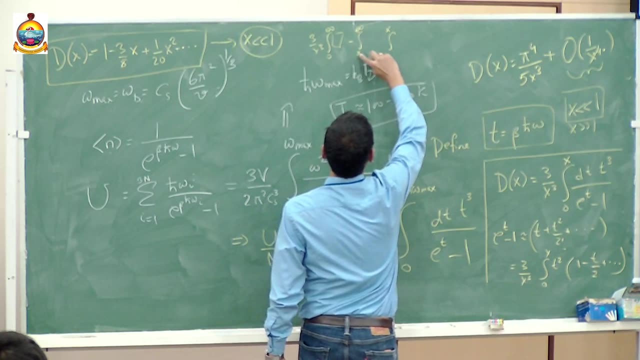 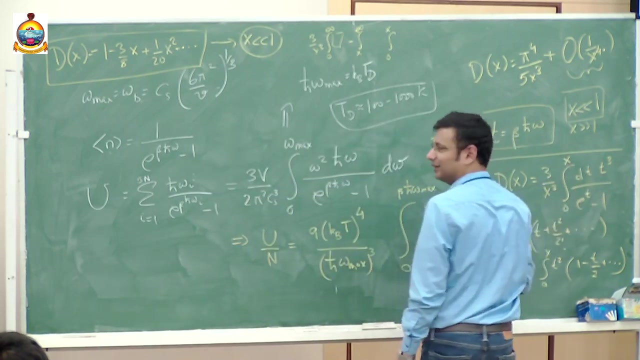 somebody tell me What should I put there? It is not 1 by x to the power 4.. That is wrong. Now look at this. So the piece that I am ignoring is from x to infinity right, What? 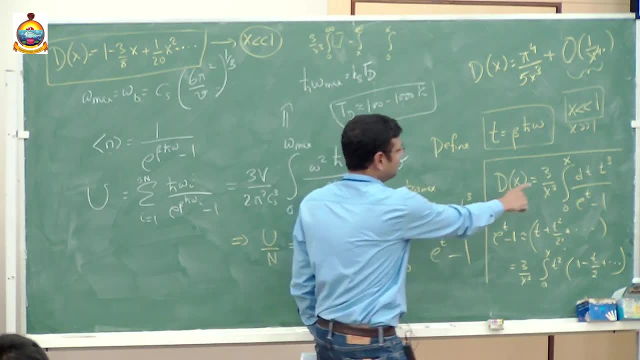 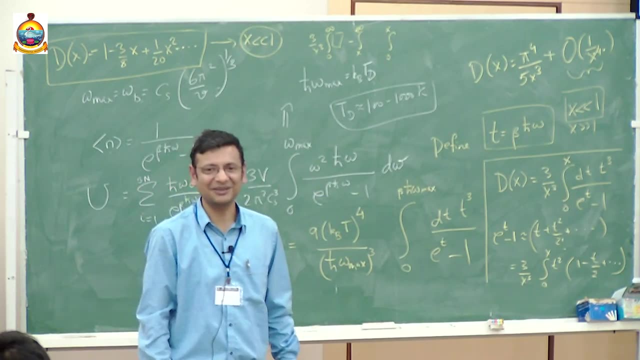 1 by x to the power 4.. Why Look at the integrand as well? I mean this is a mathematics problem, right? You do not look at half the expression in mathematics, You look at the full thing. I mean this is: 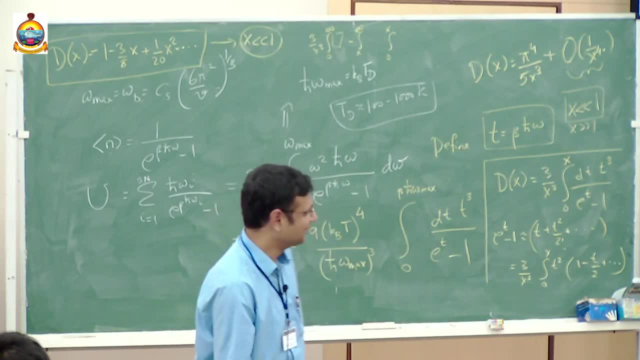 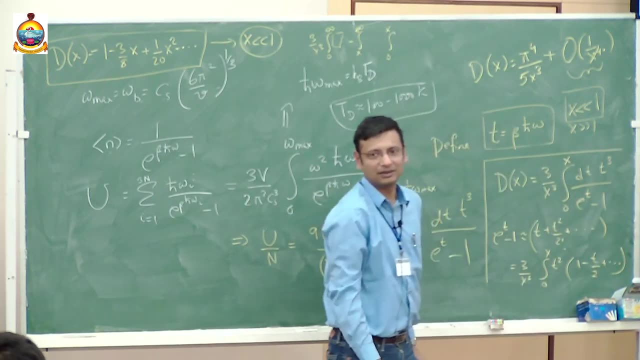 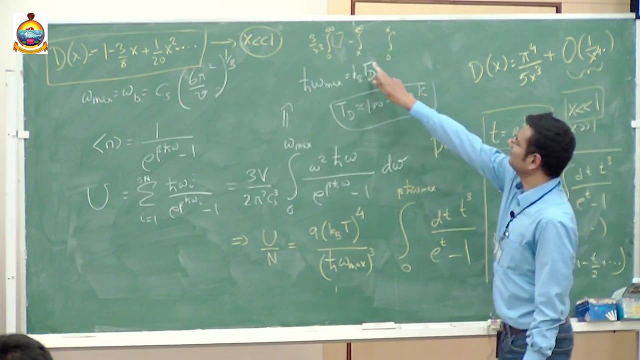 something we even learn in school. Yes, Look at it, right, Look at the full thing, Look at this, Look at this, Look at the integral. That will tell you the answer. But you do not seem very confident, right? But it should be obvious, right? So the integral: 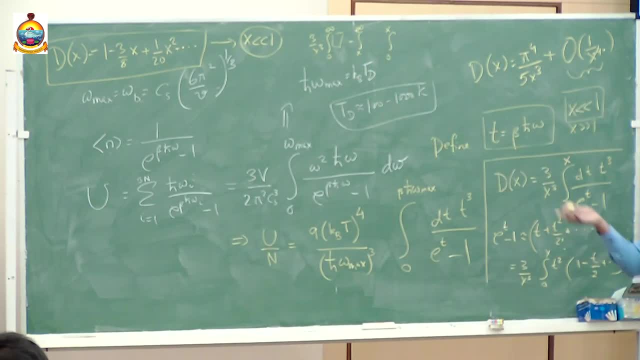 is from x to infinity, right, So x is always large, because that is what my assumption is. So then what is the leading behavior here? I can just this guy is a very large number because x is large. So I can take it to the numerator: So it is roughly equal to 0. So 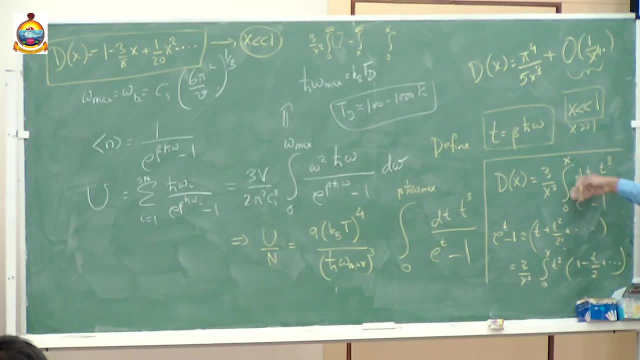 it is roughly like e to the minus t and from x to infinity, So I can just pull out the e to the minus t. So the correction goes like e to the minus x, because this is a very small number, right, And how small is it? It is characterized by order: e to the minus. 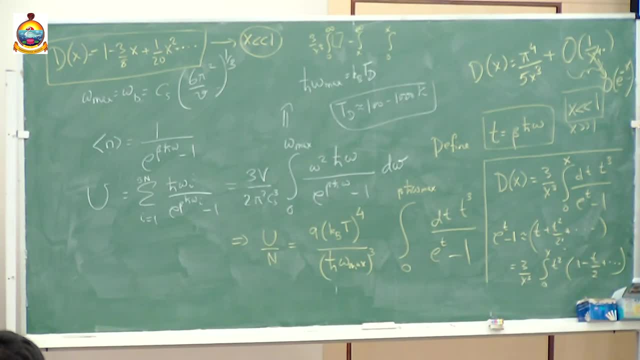 x. okay, Is this clear? So this is actually faster. This is actually faster than any inverse power law that you could have written here right Just from the simple analysis. Then you can continue. Okay, good, So we got all this, So we got the behavior of this. 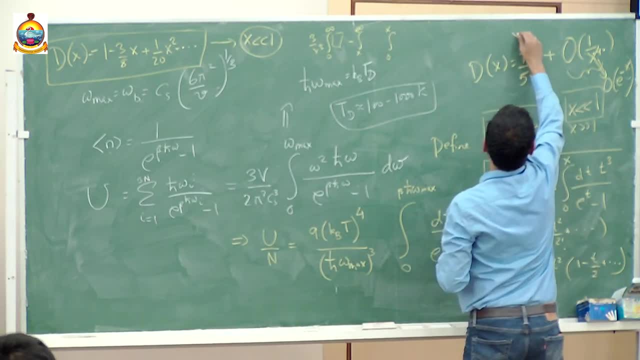 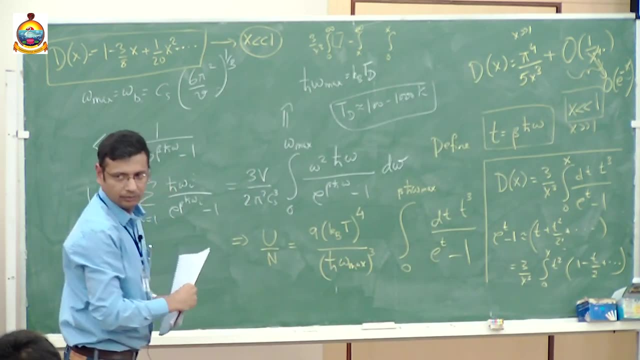 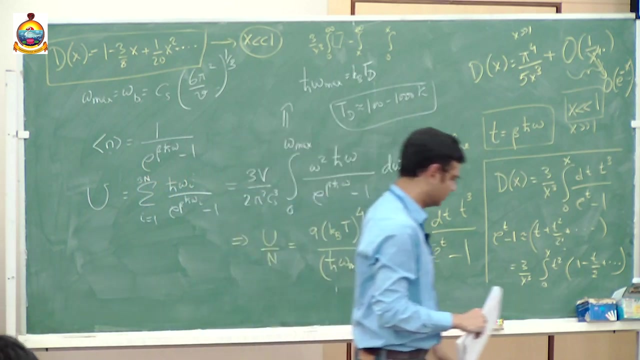 function at large x and we got the behavior of this function at small x right. Good So now I will just write the answers there and then we will immediately get the specific heat right. Good So I have to write the answer. 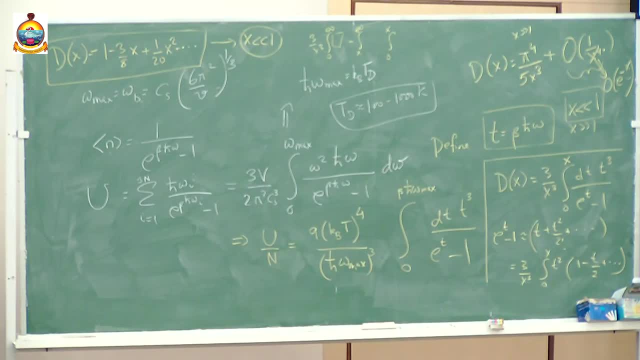 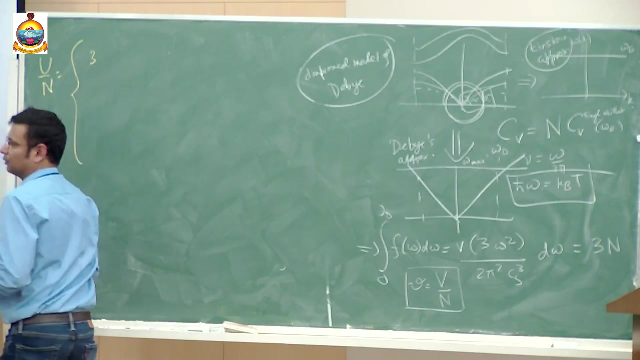 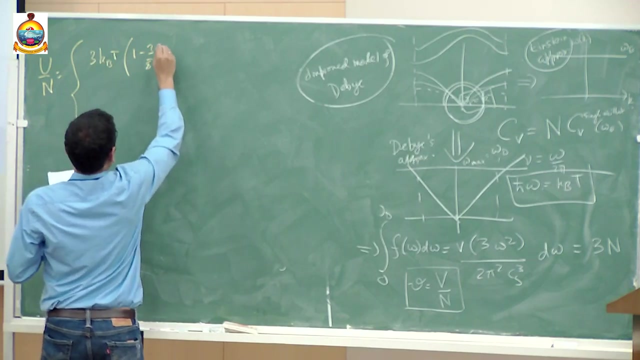 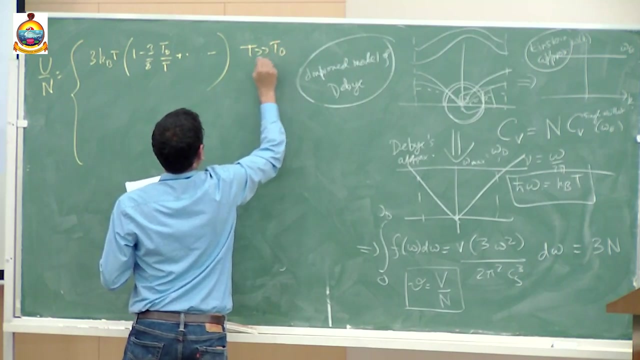 Okay, So let me use both these things now. right, This and that. So let me first use that power series, Then, at high temperature I get. So see, this is very nice, because this recovers your. 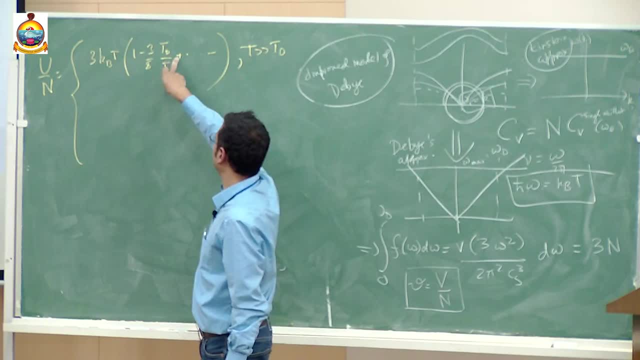 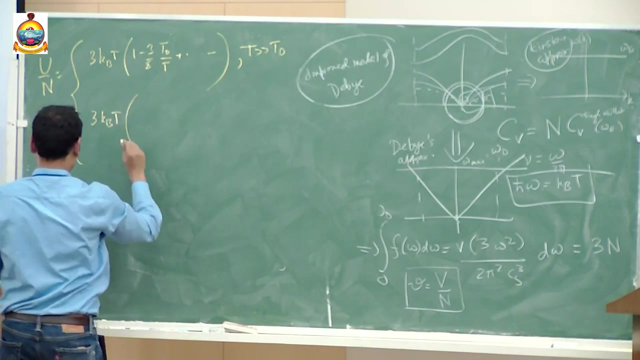 classical answer. right, This is your classical piece, and then it of course gives all the corrections as well. right, As you go lower in temperature. okay, Now let us look at that thing: X much, much greater than 1.. So see, this is C is much greater than 1. by 2, by 2 into x, to 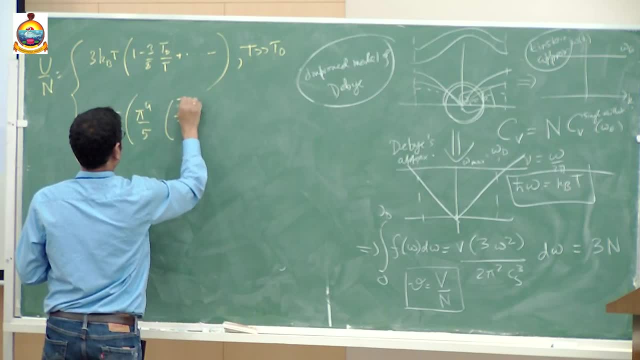 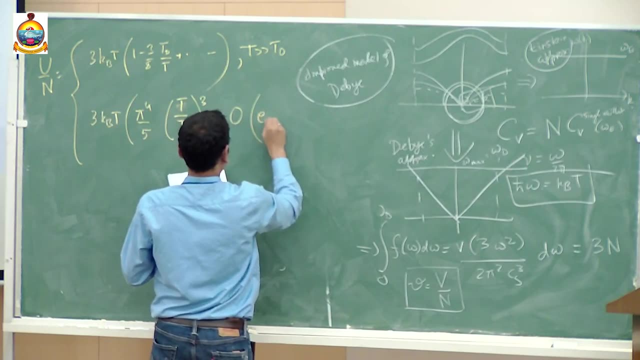 the power minus 1.. Okay, So now you can get this particular parameter. You can get this parameter. X is much, much greater than 1 by 2 into x to the power minus 1.. So once again you can see at x and C are co Technical parameters. Percentage incidence of x is 1.. Okay, So it. 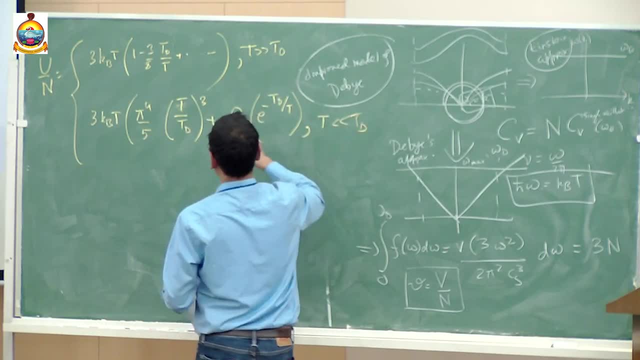 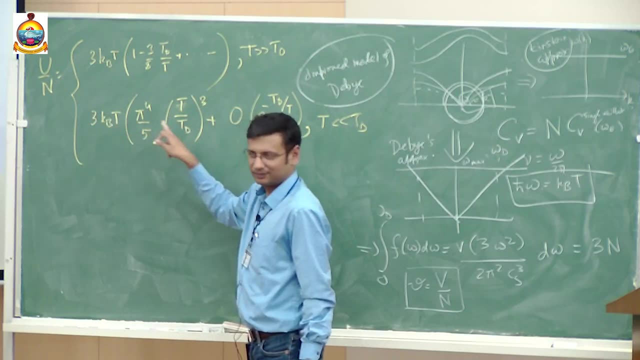 is a lot more similar than will be x, So it will be x by 2 into x to the power minus 1.. So So see, the energy is actually going as T to the power 4. I just use that right. So 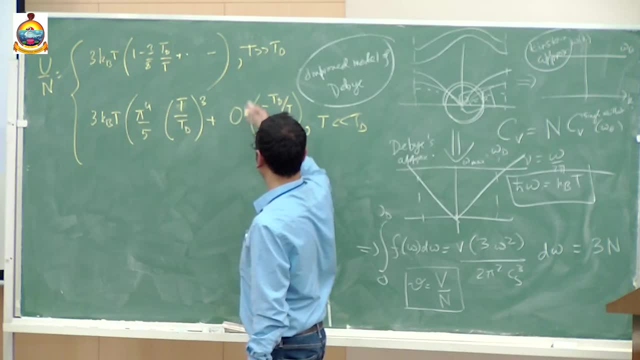 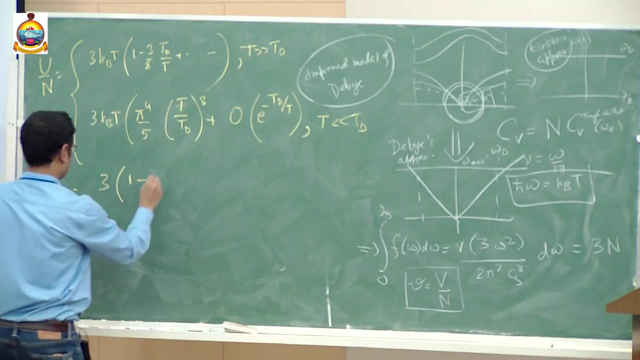 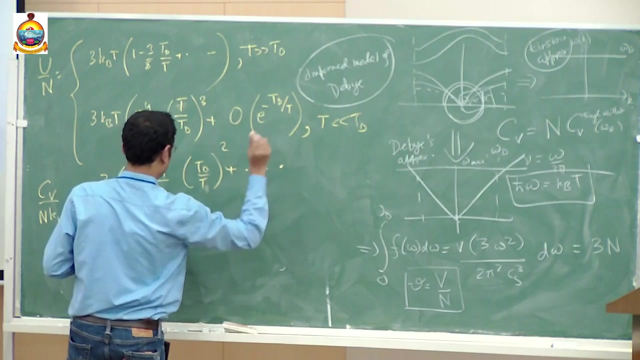 it is actually going as T to the power 4, and then there is a exponentially rapid correction on top of it, right good. So now we know what the specific heat is. we just differentiate this and that with respect to temperature. this is for that and for this. 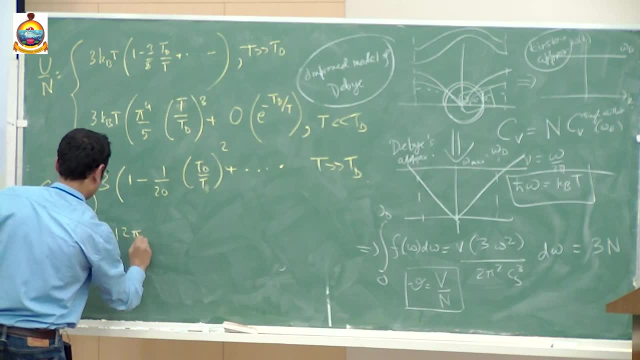 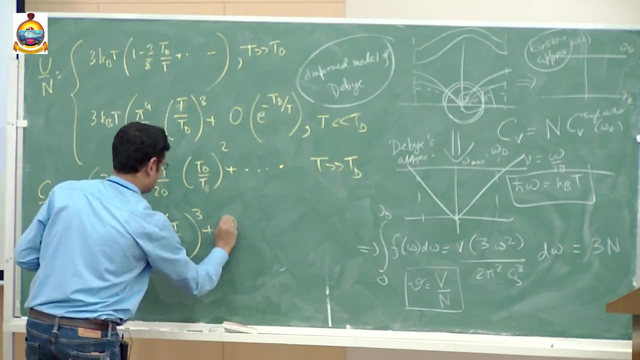 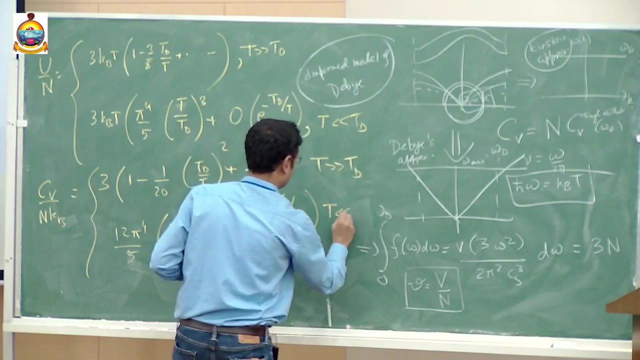 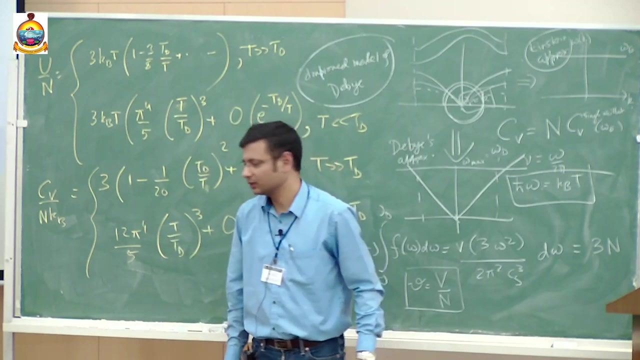 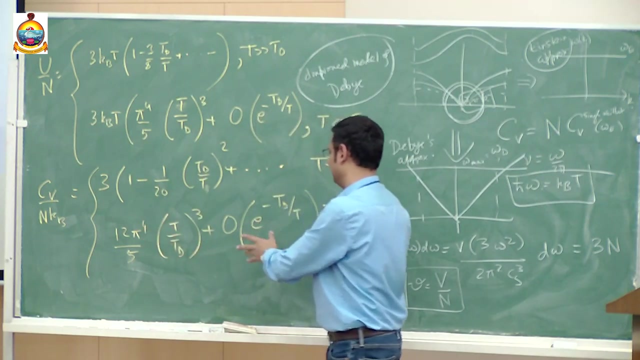 That is it right. So automatically we see that in the Debye approximation this specific heat causes T cube right. For any temperature scale which is reasonably small compared to T sub D, this specific heat actually goes like that, in fact. 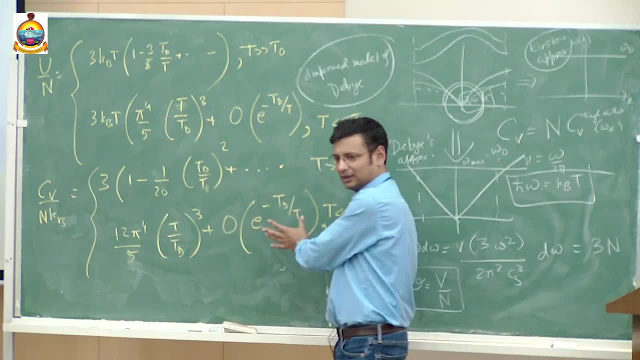 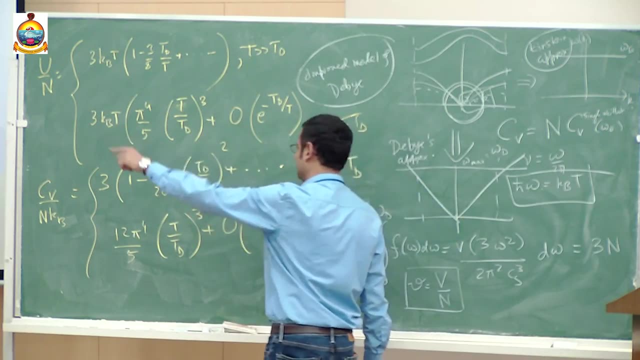 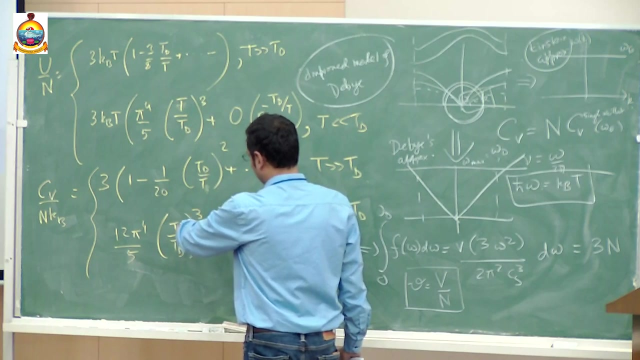 it does not even need to be too small, is exponentially small, right? so we also get the first correction here and the first correction here. here, actually, it's straightforward to get more corrections as well, but it just gets more and more tedious. okay, so, as I said, as I hope I have conveyed to you the universal physics that 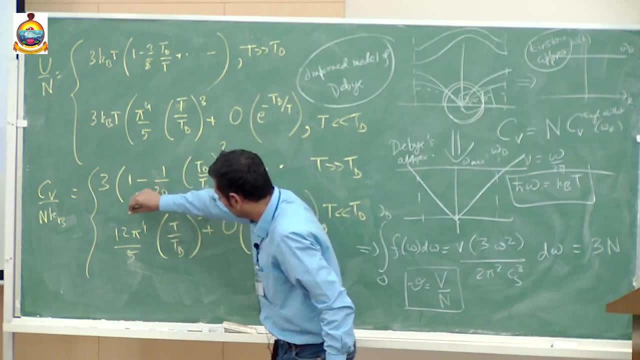 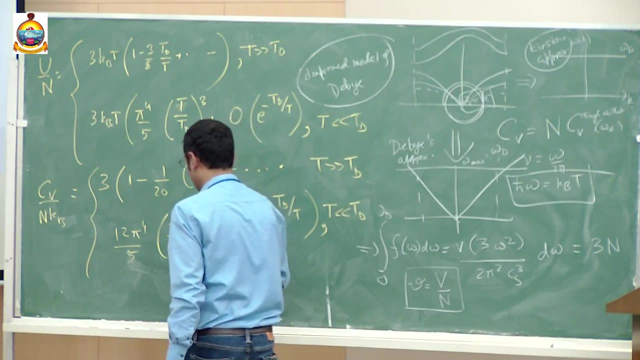 you should keep in mind. here is the TQ, this number. so see, as I said in the insulator, the specific, it is a times TQ, right? so here in the Debye approximation the number is 12 pi by 4 divided by 5 times, sorry, divided by T sub the whole cube, right, that's the number. but this might. 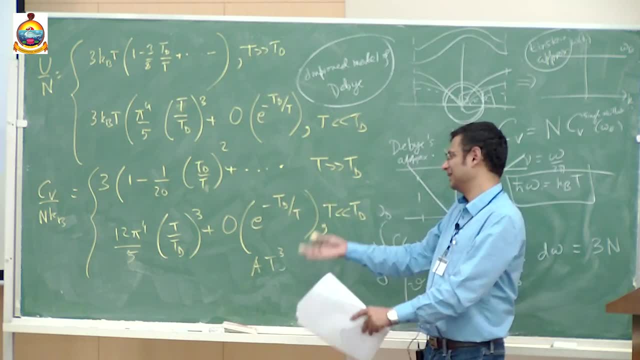 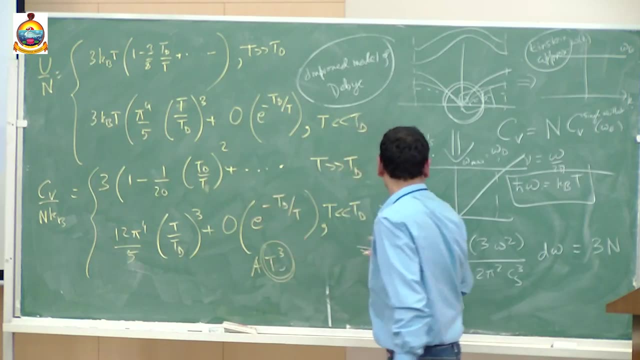 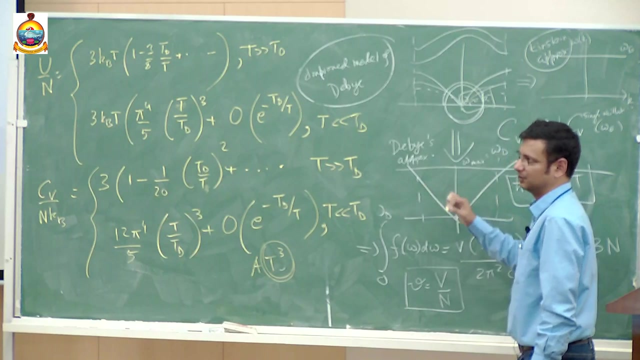 not be the real number. it might be for certain things, but it might not be the real number for certain other things. but whatever it is, this power would be correctly captured because the important physics which gives you this power is that the modes are gapless and they are linearly dispersing. that's the key point. okay, right, that's the key. 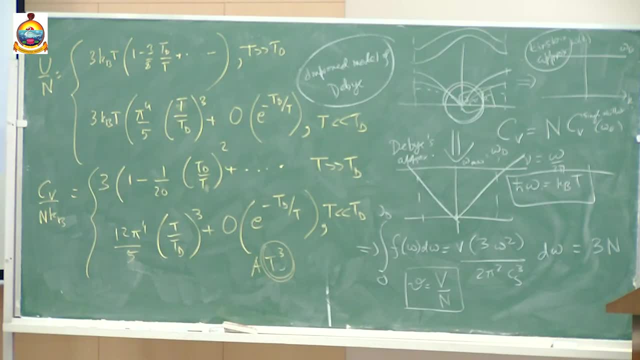 point. so actually now, some after this was done, people also thought, oh, let me use a combination of Debye theory and Einstein theory, right, and try to get the whole specific heat curve right. so what did they basically do? you see, the Debye theory is taking care of the acoustic modes, right, and then 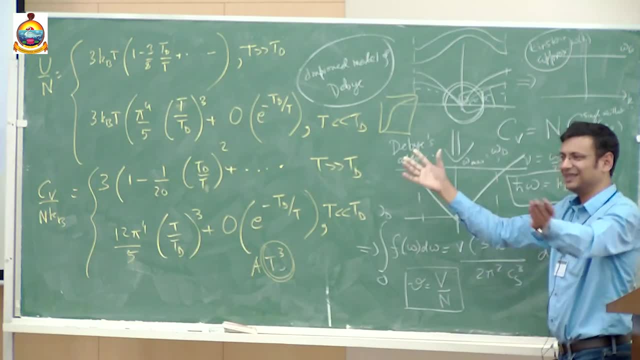 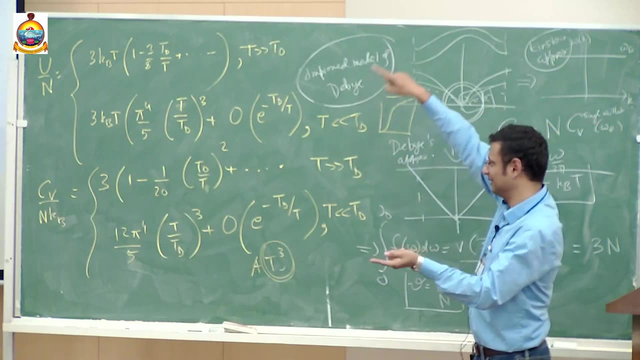 they took care of the optical modes using Einstein's approximation and then they just patched up the two answers and of course that answer had a wider range of validity in temperature space. but of course that still didn't change this T cube. but that is also a very nice interplay of 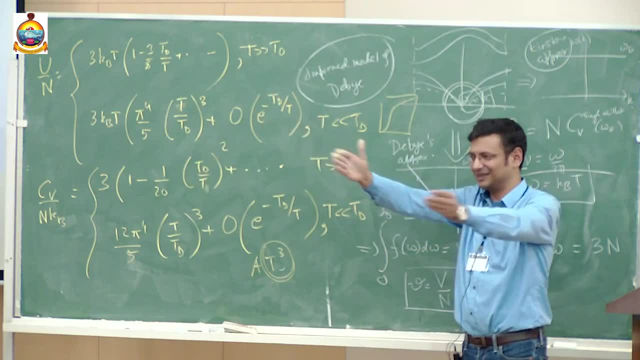 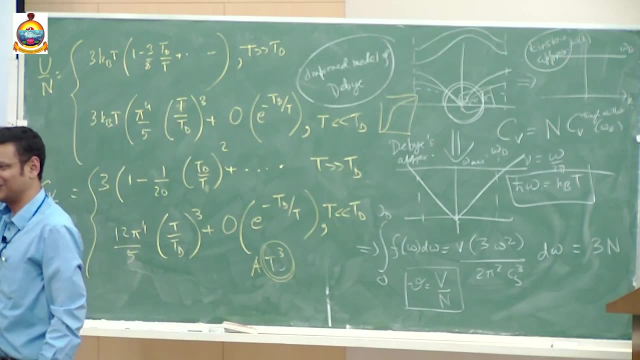 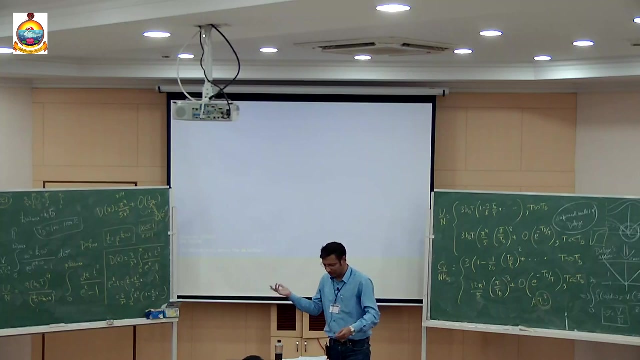 using two approximations and patching them up to get an answer which is relevant at a broader temperature scale, right, so people did all kinds of stuff and then in that last paper I showed you people have done very clever stuff and they can just match everything from experiments, right, okay, good, so I am right on time. so I think this is a good point to stop and I'll take any questions you have, but at least we have proven one very important thing: that the specific heat of insulators goes like this and this is the physics of it, okay. 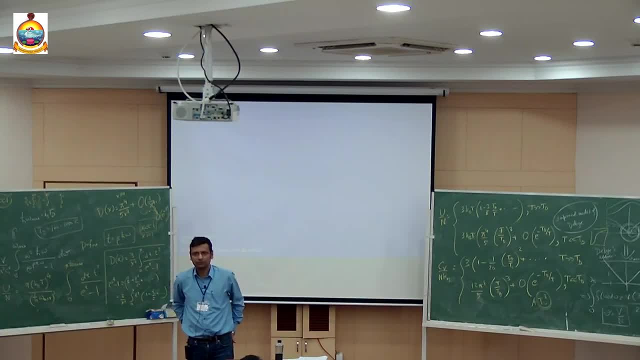 Sir, at the time of Debye's transformation was the actual dispersion of the No, the experiments came a bit later. Oh, for some simple crystals. people appreciate that this thing should happen. No, no, Goldstone theorem was not known. but you don't see, when I first learned this, I didn't know Goldstone theorem. 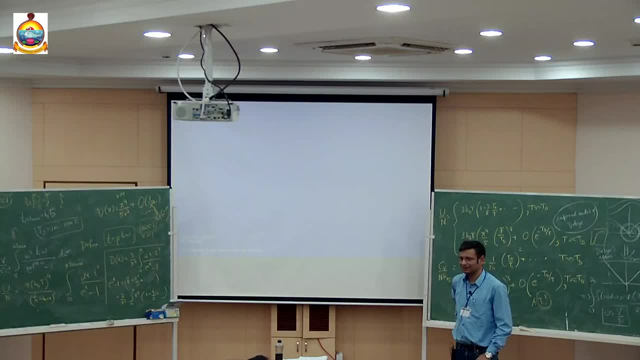 K square, K square, So guessing it? K? Hmm, Correct, See, Debye's insight was. Debye's key insight was that he realized that if you are considering soft modes, like modes with very low energy, they have very long wavelength. and if you have a very long wavelength, Debye made a very reasonable assumption: that you can ignore the crystal structure. and then it's like you have an isotropic solid. and for an isotropic solid, people already knew that the traveling excitations were sound waves. 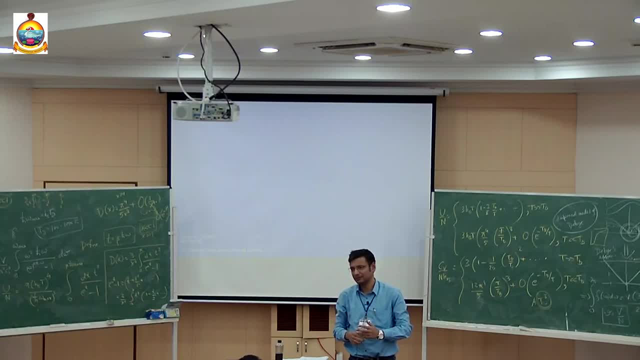 Yes, So that was his insight. Correct, The dispersion curves were not known, but the specific heat curves were known, Correct? Correct, Is that what you are asking? No, No, Okay, Anyway, whatever he is asking, I think he got an answer. 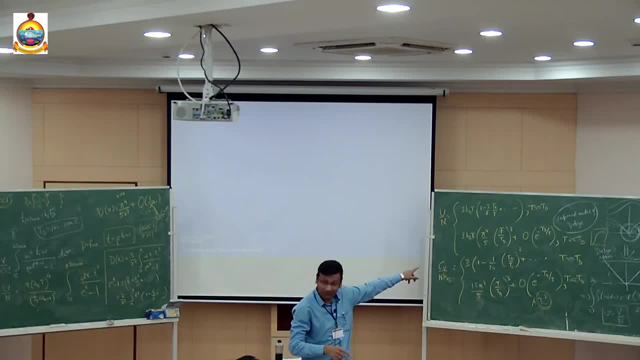 But you see, I mean, yeah. So the specific heat curves were of course known. Einstein even worried about this before Debye, but then we discussed what was wrong in his thing. No, no, that was the sound wave, that was his insight, Correct. 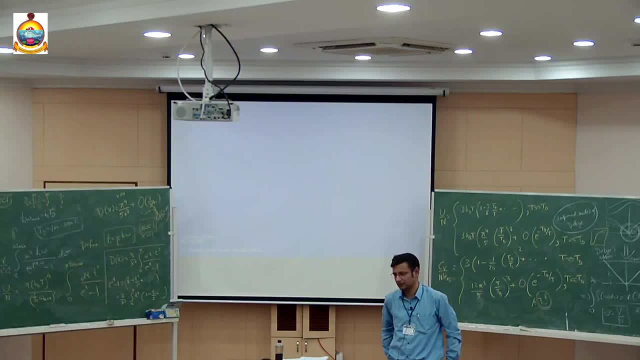 Correct? I think so. Yes, So that linear input. that was the answer. So this omega t by T by T d. you know, T by T d is coming from omega d, right, T d is coming from omega d, Yeah, 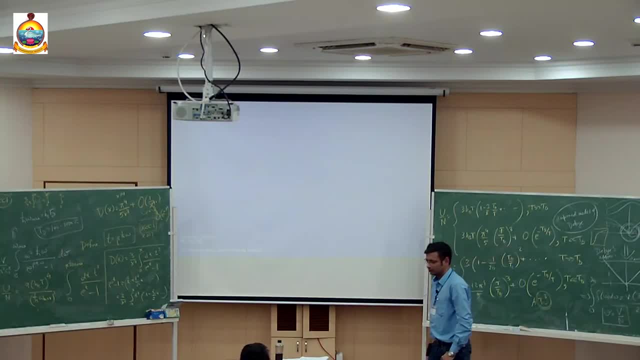 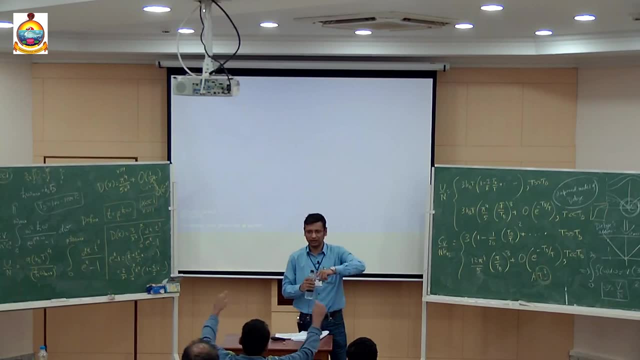 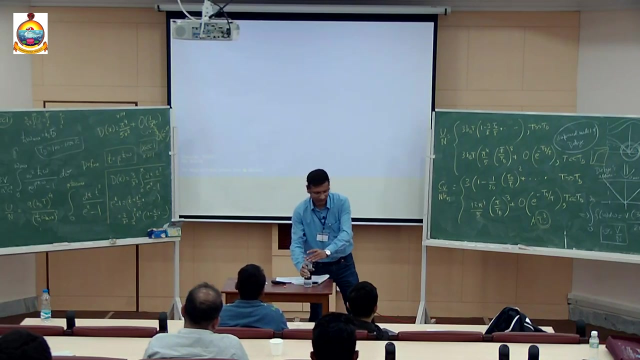 So if you, if this calculation, if you replace by a function, for example sin, some alpha x, rho, So you go like, Oh, like There is, no, There is no way to put a external cut off from outside. No, no, but see, this omega d cut off is roughly related to this. debye. 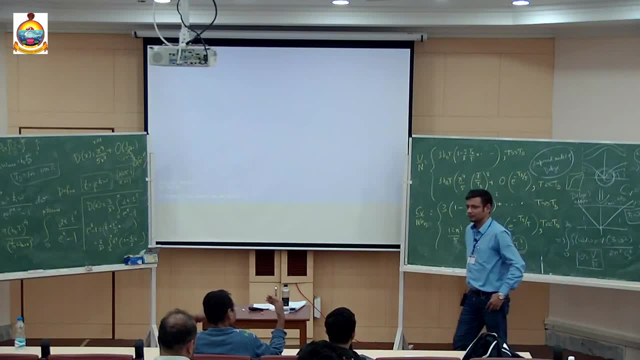 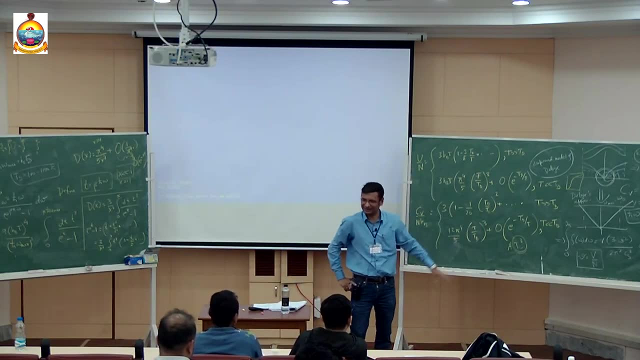 Roughly related to this bandwidth. Yeah Yeah, You can take this function, Yeah Yeah, For example, But still you will have a temperature scale like this. Yeah, You will have a temperature scale like this. That is related to the bandwidth, as I said. 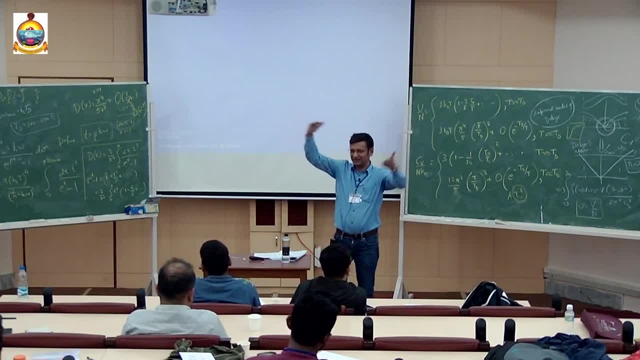 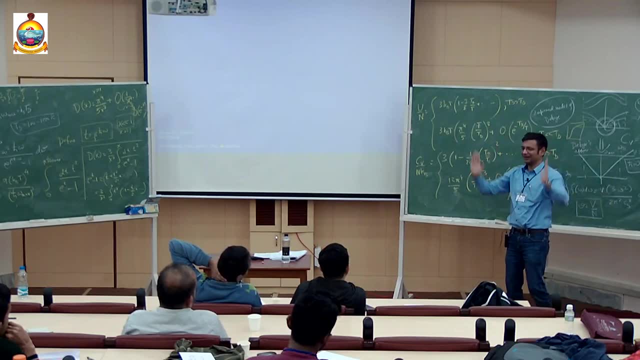 Yeah, Yeah, Because it will deviate from linearity and it is related to the bandwidth. Yeah, Exactly, See both: in Debye's model you have to cut it, and in this thing you have to still cut it. So the relevant thing is the bandwidth. 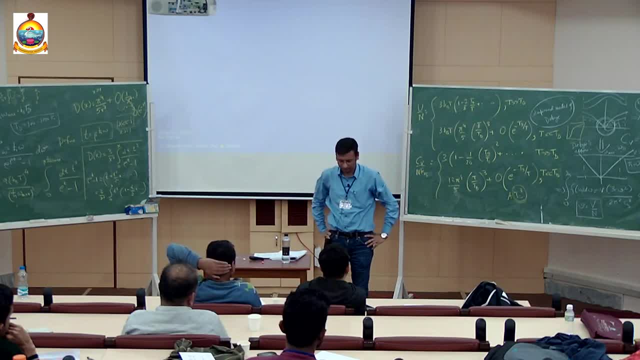 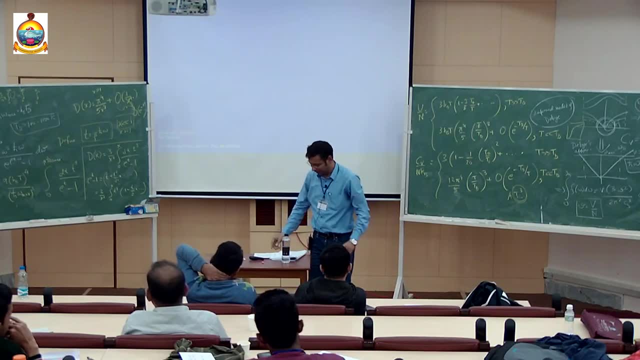 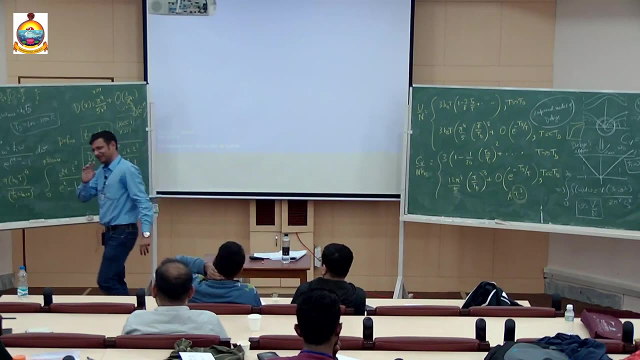 Oh, thank you for this question. Since I have minus 1 minute left, I can answer your question. See, we should sometimes be surprised at our own calculations. Yeah, Let me tell you what is surprising. So you said that I just took quadratic interactions. 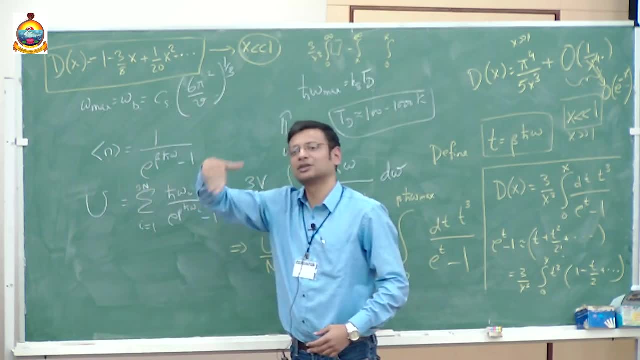 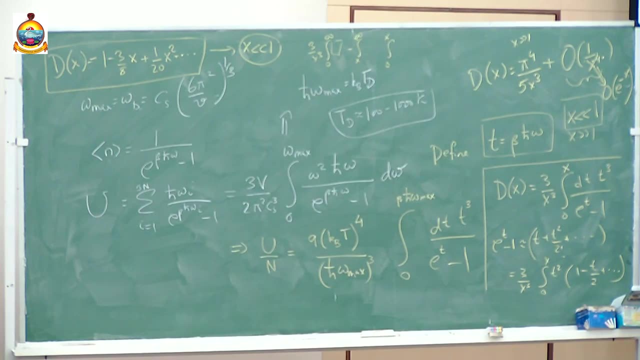 Of course, in my full model there is cubic interactions, Cubic interactions, quartic interactions and so on. So then the harmonic oscillator problem does not remain harmonic Right If the temperature increases, for example, Because then the fluctuations become higher. 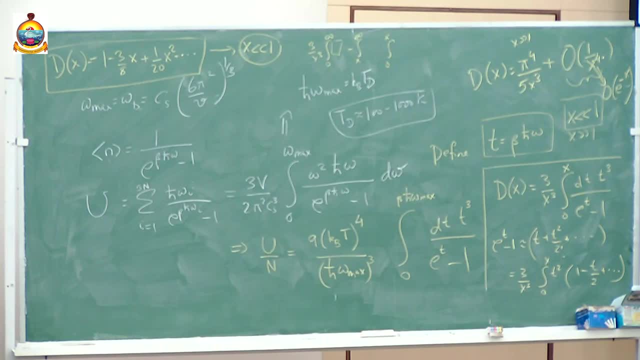 Right And you can. you should then think of corrections to the model. So, of course, as I gave in one of the exercises, it is like a harmonic, anharmonic oscillator, And then there are interactions between the different modes at different k. 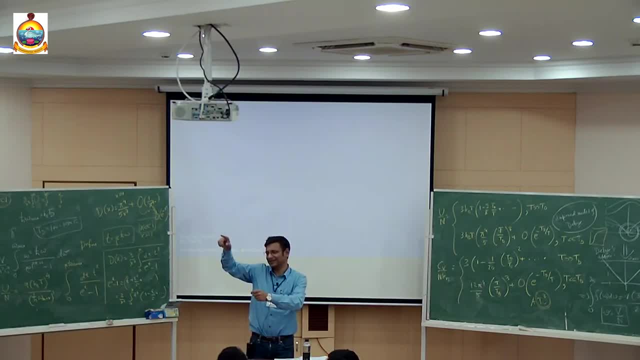 There will be terms like: Yeah, A dagger k1, a dagger k2, a k3, a k4.. For those who do not understand, ignore. But k1 plus k2 plus k3 plus k4 would conserve momentum, and so on and so forth. 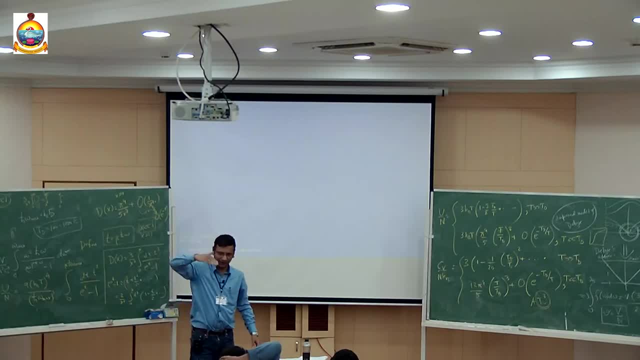 So there will be interactions between the phonons as you raise the temperature. So now you can ask: does it actually? Of course, there are anharmonicities. Does it actually lead to anything interesting? So the first part of your thing is this: result is not affected by that. 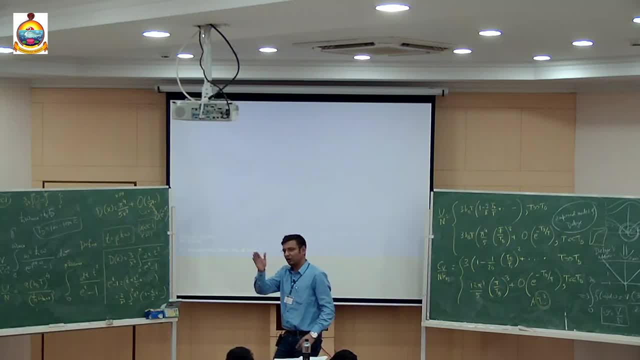 Why? Because this is a low temperature result At low temperatures. automatically you are back to the assumption that the fluctuations are small, So that part is okay. Of course, if you keep on cranking up the temperature, the crystal can even melt. 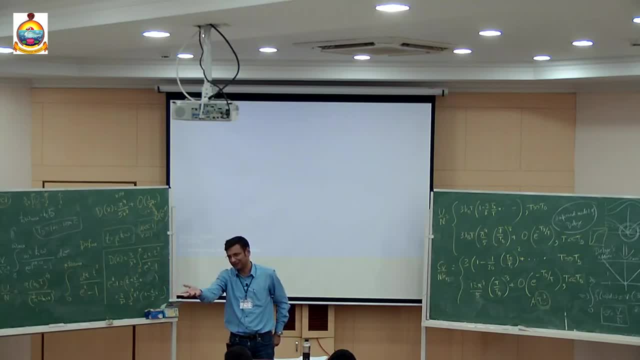 Obviously, most crystals melt and that is an anharmonic effect, for example. Second effect is- which happens even before that You know most crystals, when you heat them up, there is an expansion of the length. In this kind of a harmonic theory you can never get an expansion. 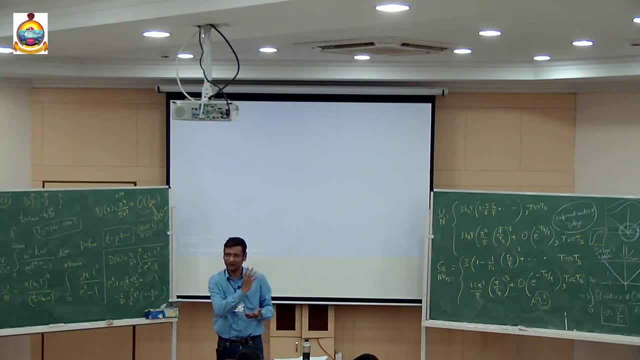 That is impossible. I mean that you can just argue by symmetry, So you need anharmonicities for an expansion. The third thing which is also immediately clear is, if you just consider a harmonic theory like this, like what I said, The harmonic theory captures one thing very correctly: that it is T cube specific heat. 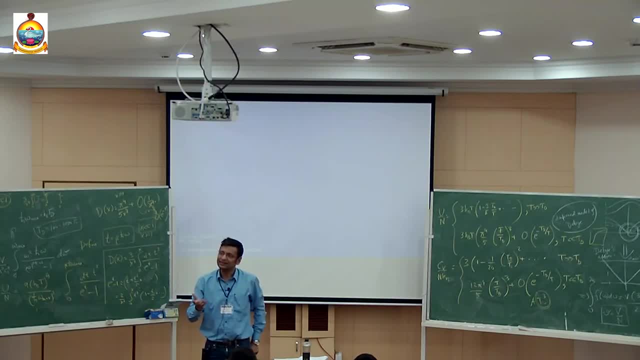 at low temperature. right, But then you can ask the question: does it capture everything correctly at small t? That is a perfectly valid question to ask. It captures one aspect of the physics correctly at low temperature. That is, the behavior of the specific heat, how the energy changes, and so on. 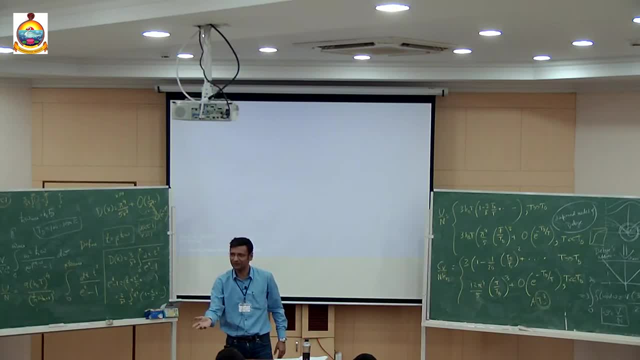 But let me give you a quick answer of what it gets completely wrong, even at low temperature. So suppose you have a crystal and you make this harmonic approximation and you ask about, let us say, thermal transport, Like you just pump in some heat and measure the thermal transport in the crystal. 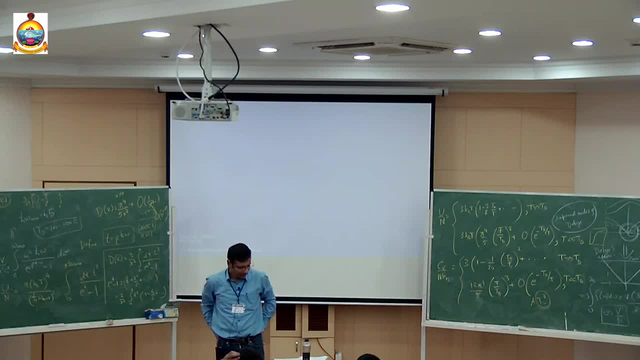 Try to define some conductivity from that. In this approximation we will get infinite conductivity in this harmonic approximation. But even at low temperature if you do an experiment you will always get finite conductivity And that finiteness of conductivity comes due to the phonon-phonon interactions that 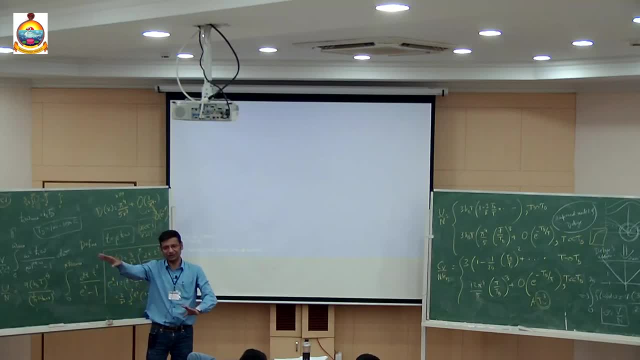 we have ignored. That is one reason. There are other reasons. There are some disorder effects, whatever, whatever. But if you take a completely clean model, phonon-phonon interactions make the infinite conductivity finite, So there are certain things which is incorrectly captured by this model, even at small temperature. 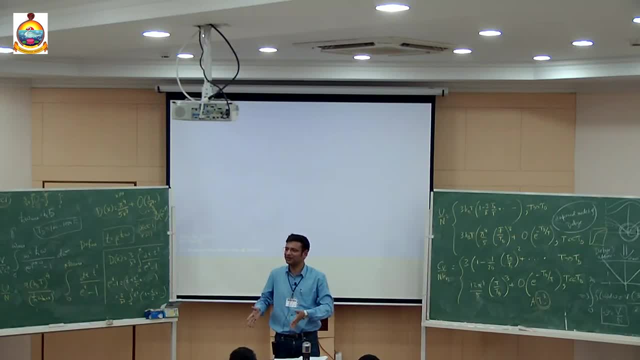 But there are certain other things which are correctly captured. So whenever you make an approximation, you should always ask yourself that what am I capturing and what am I not capturing? Just because one thing matches does not mean that everything else would match. That is very important to realize. 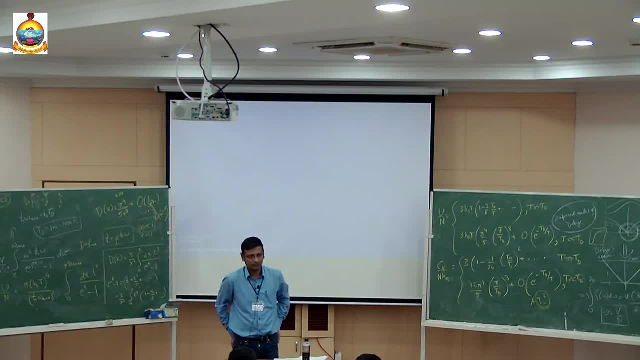 Just remind me what is this Wiedemann-Kanzler that says… Heat… Right, What is the heat? Electrical? No, no, Thermal by electrical. But here it is irrelevant because we are talking of insulators. But yeah, you are correct. 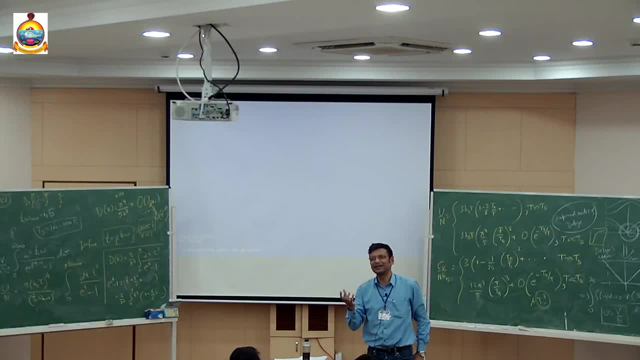 I mean? Wiedemann-Kanzler essentially says that for metals, what is carrying the current is also carrying the heat Roughly. that is the statement. But this is an insulator. And what point you mean for doing that? this is an insulator? 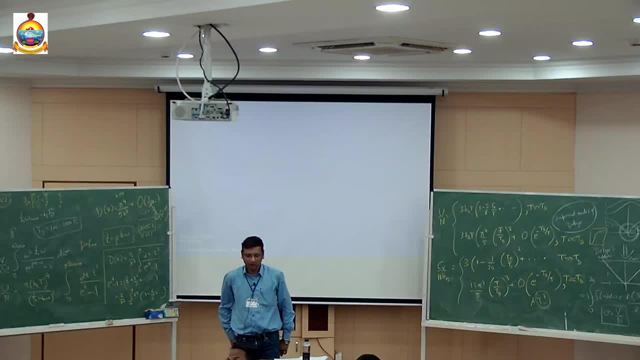 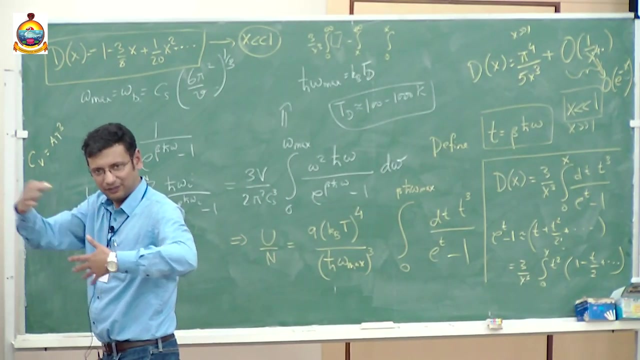 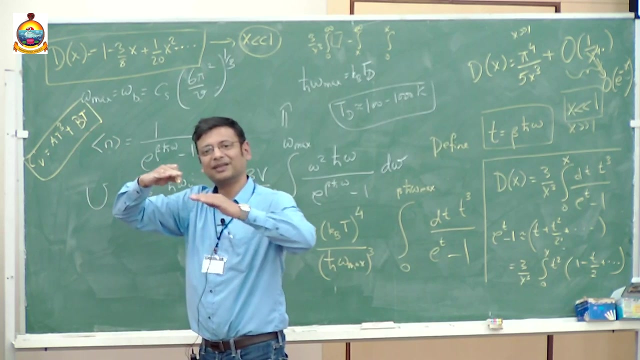 Oh, very good, I have not explained that to you Somewhere during the course of my lectures. I will show that for a metal, in fact, this A times T cube will remain there because it is due to the crystal vibrations, But there will be another term, which is B times T, And this would come because of the 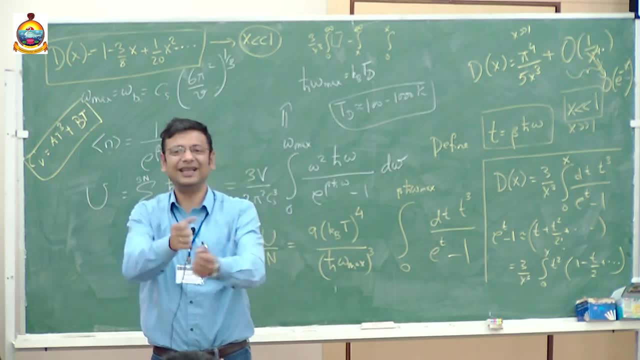 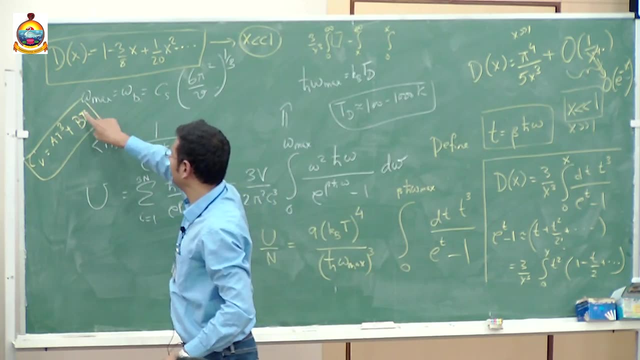 fluctuations of the electronic degrees. See, in an insulator the electrons are not free to move. You need to pay a very high energy cost to move electrons around. So for an insulator this piece is exponentially damped. again for the electronic degrees. 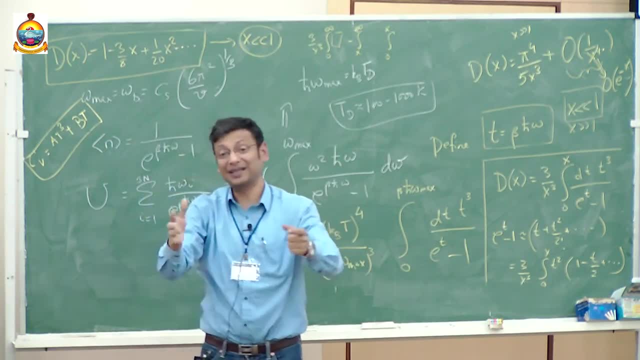 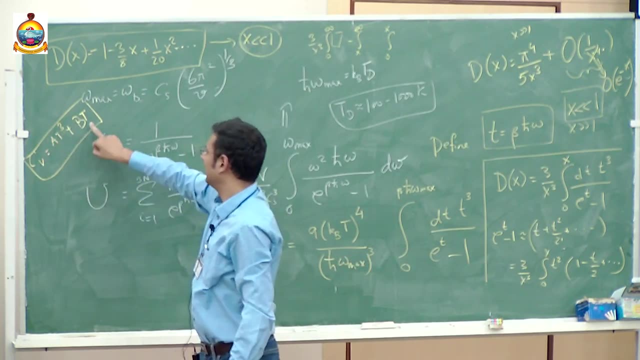 You see, because there is a big energy gap to moving electrons, But for a metal electrons can move freely apart, So then you will get a non-exponential thing again for the electronic contribution And that contribution in fact at low temperature. you see, this goes linearly and this goes as. 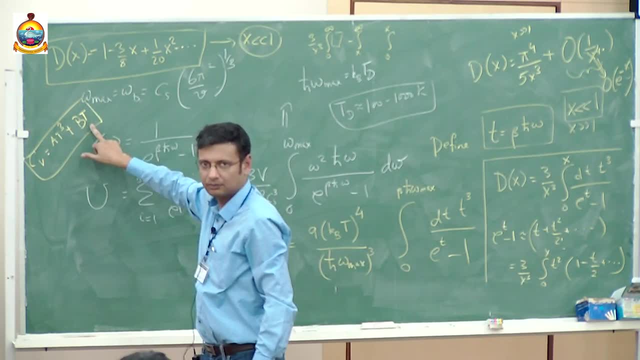 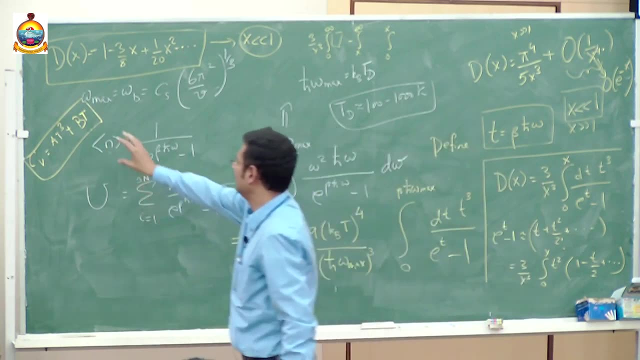 cube power of T. So this is bigger right, So this is more important. So we will study that, So we can just think of a free term, Free electron system and we will get this piece out of it. So the approximation I used is: I can ignore this because it is an insulator. 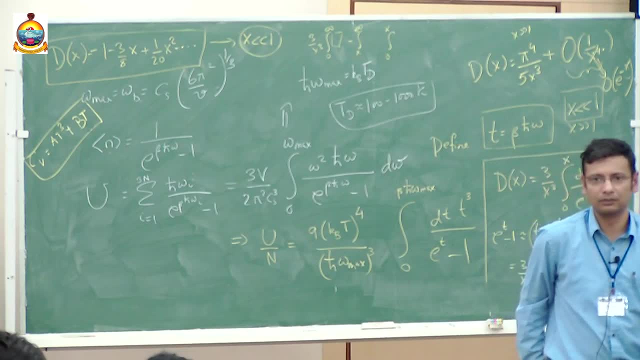 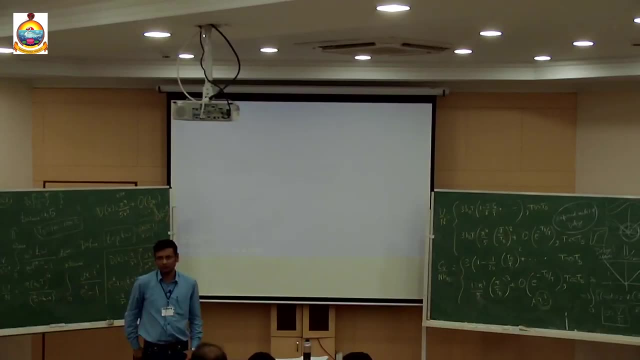 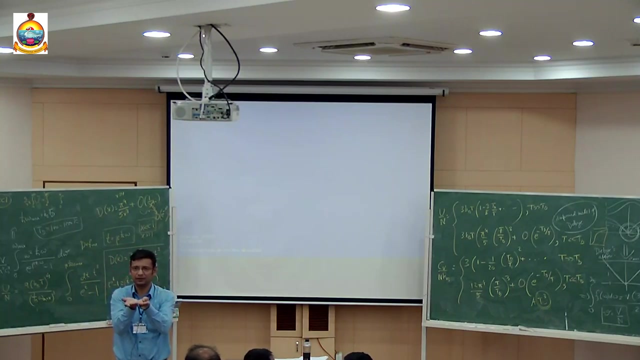 Sir, we have a general idea of what is an insulator, based on the band filling, Correct. So when it is a metal, you see there is something called a Fermi surface Right Now, basically, roughly the picture is, but this is very crude. 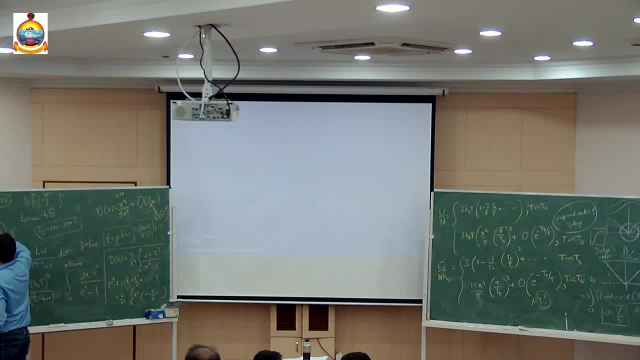 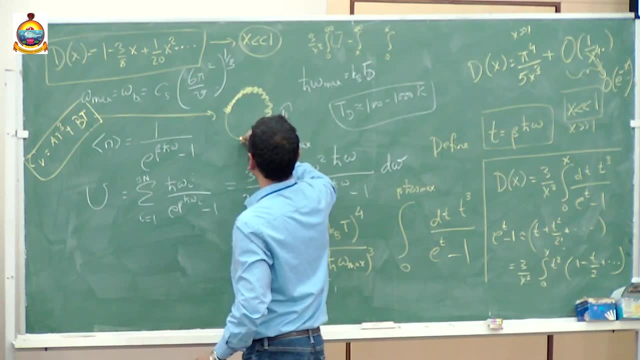 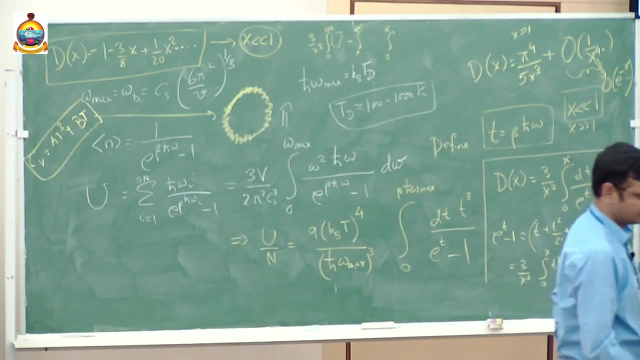 We will do a calculation Roughly. the picture is so. this is the Fermi surface and the fermions which are sitting near the Fermi surface. they can have gapless excitations like this And these gapless excitations give this. 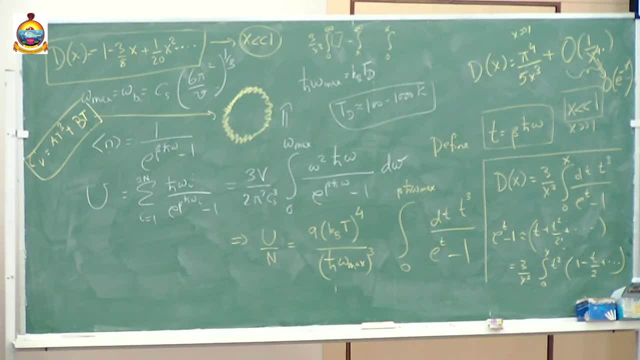 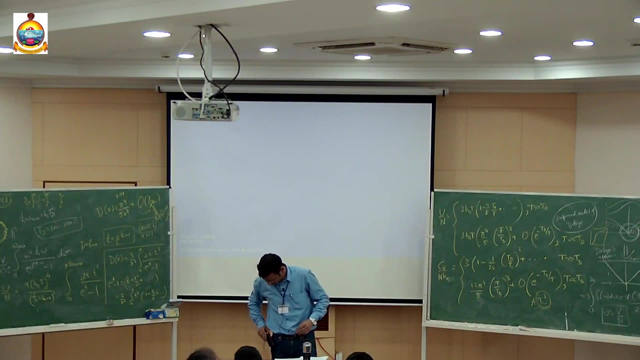 Okay, If there are no further questions, then we break for lunch.